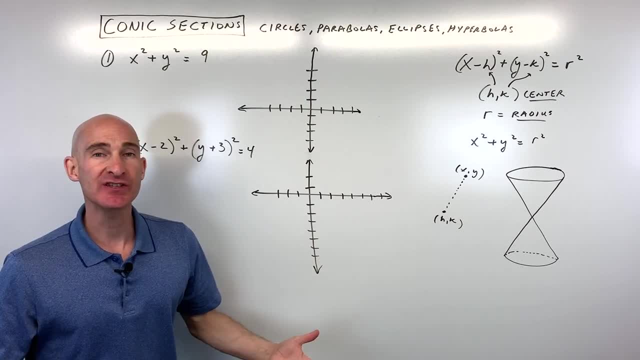 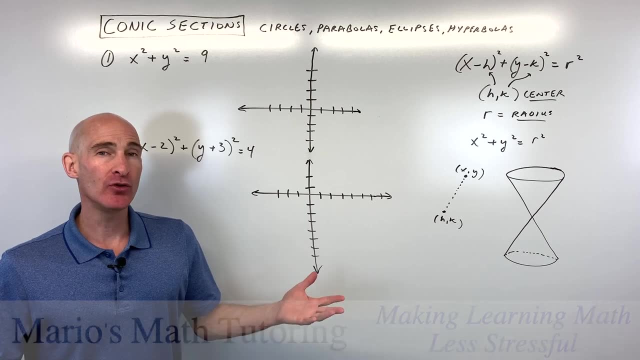 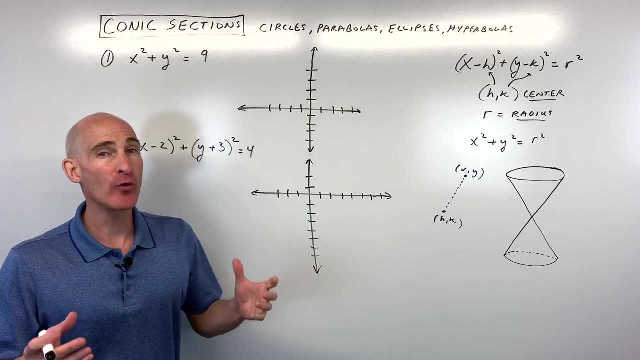 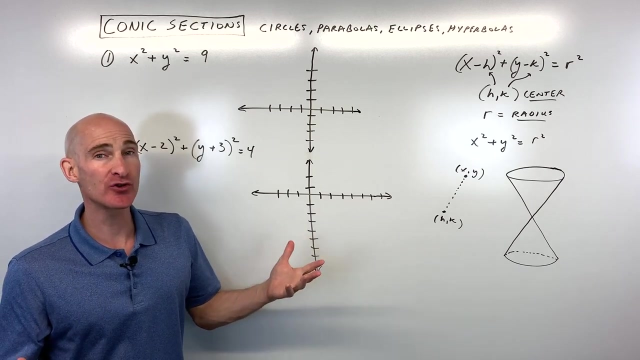 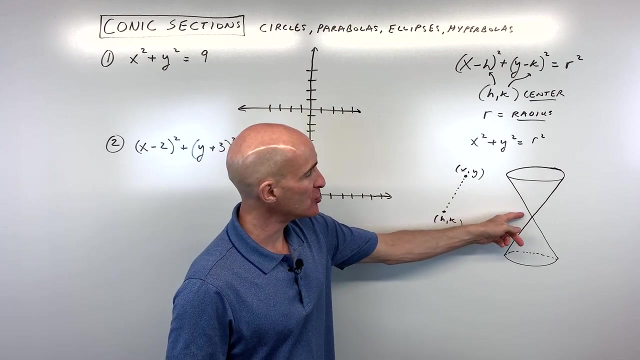 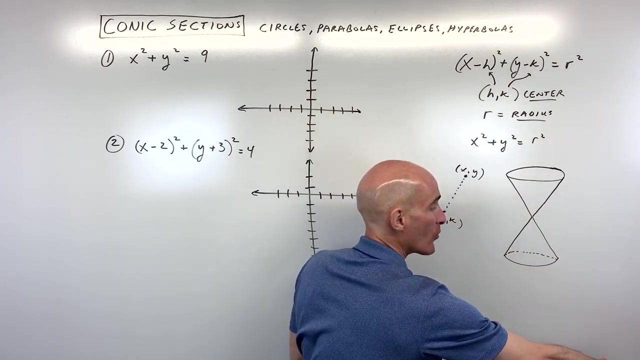 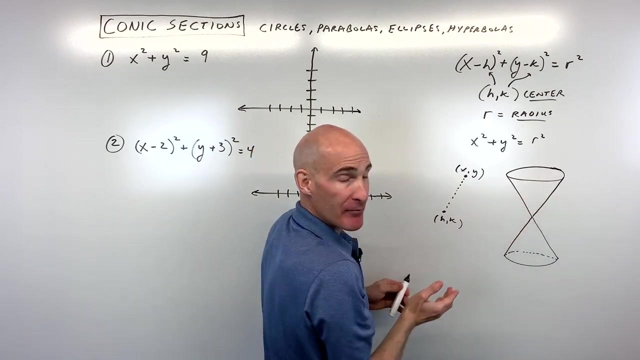 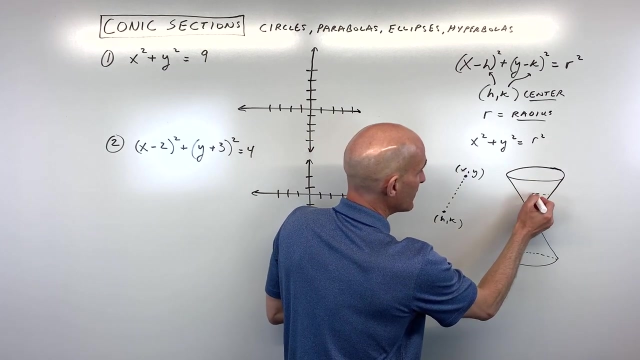 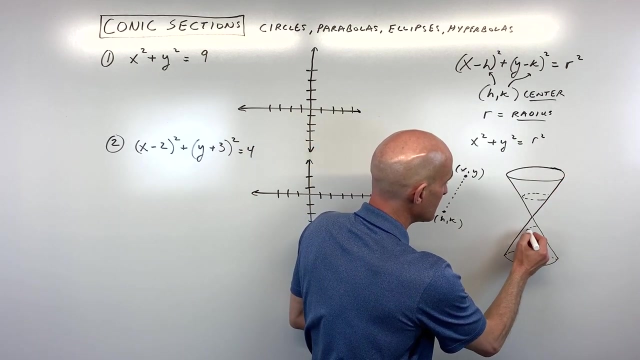 In this lesson you're going to learn how to graph the conic sections when they're in the standard form. We're going to be talking about circles, ellipses, parabolas, hyperbolas. And what makes this difficult normally for students is that there's a lot of formulas, a lot of things to memorize. So we're going to go through the different formulas and how to get a good sketch of the graph when it's in that standard form. So let's start off easy and we'll get progressively more difficult as we go through this lesson. First, let's start off with circles. They're the easiest and basically when we're talking about conic sections what that comes from is like if you were to have two cones like this like end to end and what you want to visualize is this cone keeps like expanding upwards and downwards forever and ever. And these are hollow cones and if you take like a plane like a flat surface right if you were to you know cut through that plane depending on the angle that you cut through you're going to get a different shape. So for example if I cut through just like this I'm going to get a circle which is what we're going to talk about later. So I'm going to get a circle which is what we're going to talk about later. So for example, about first but if I was to cut through a little bit on an angle okay say for example like this see you you'd get like an ellipse okay like an oval shape if you're to cut through it say for 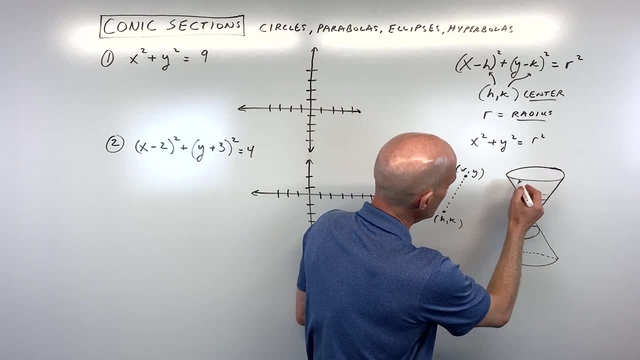 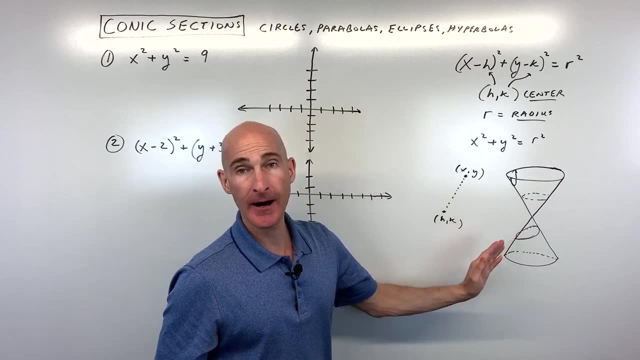 example like that you could get let's maybe cut through on a little bit of an angle here you could get like a parabola shape okay like that and if you cut through where it cuts through both cones you'll get like a hyperbola okay so we'll talk about all those in this video but first 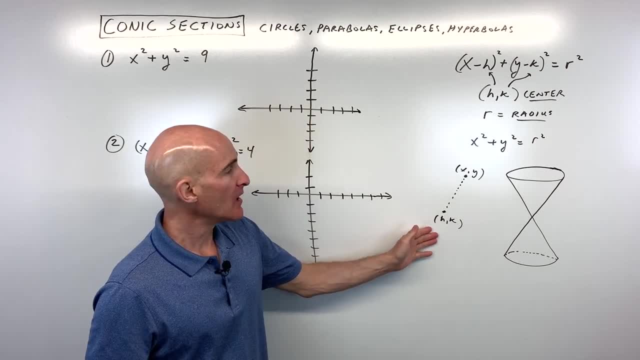 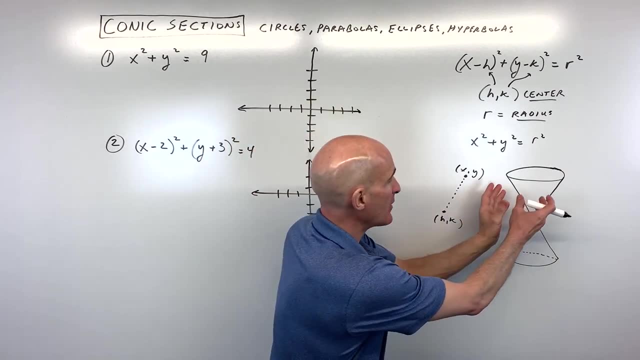 the easiest and basically, when we're talking about conic sections, what that comes from is like if you were to have two cones like this like end to end, and what you want to visualize is this cone keeps like expanding upwards and downwards forever and ever, and these are hollow cones. 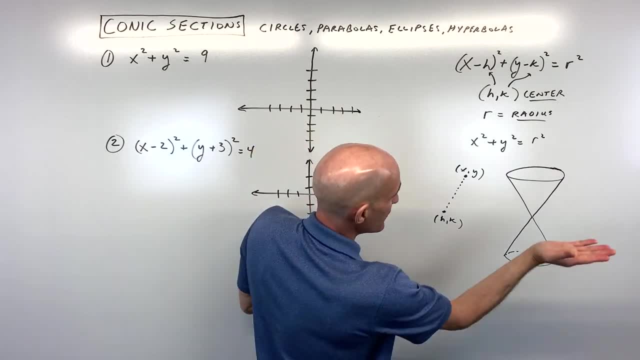 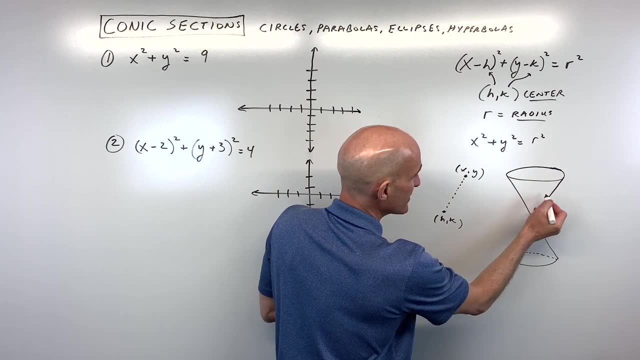 And if you take like a plane, like a flat surface, right, if you were to, you know, cut through that plane, depending on the angle that you cut through, you're going to get a different shape. So, for example, if I cut through just like this, I'm going to get a circle, which is what we're going to talk. 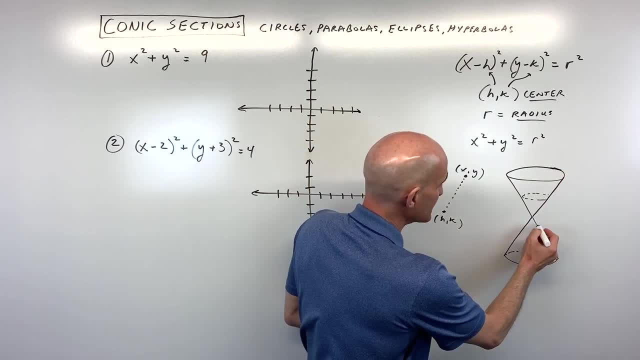 about. So I'm going to get a circle, which is what we're going to talk about. So, for example, if I cut through, just like this, I'm going to get a circle, which is what we're going to talk about First. but if I was to cut through a little bit on an angle, okay, say, for example, like this: 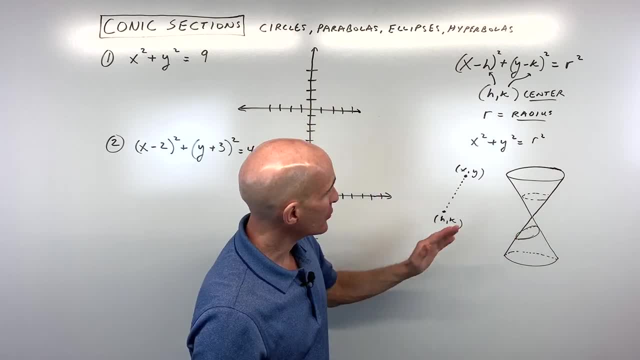 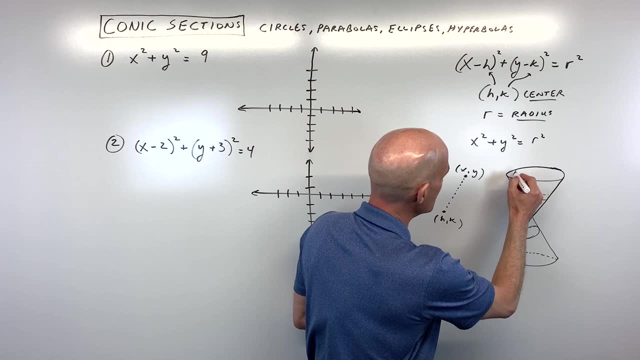 see, you'd get like an ellipse- okay, like an oval shape if you were to cut through it, say, for example, like that you could get- let's maybe cut through on a little bit of an angle here. you could get like a parabola shape- okay, like that. and if you cut through where it cuts through both. 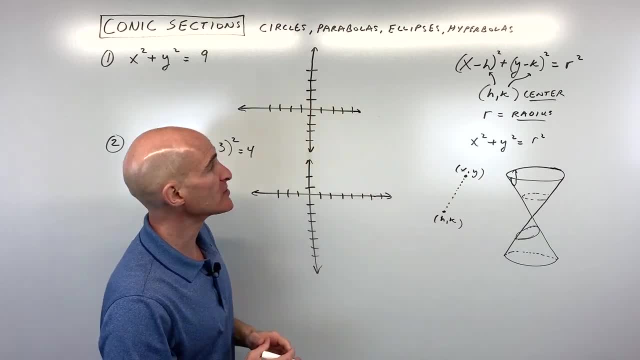 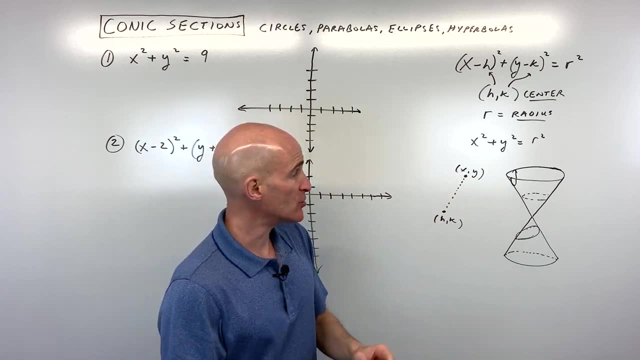 cones, you'll get like a hyperbola, Okay. so we'll talk about all those in this video, but first the circle. what exactly is a circle? it's a set of all points that are equidistant from a given point, which we call the center, okay, and the distance from that center we call the. 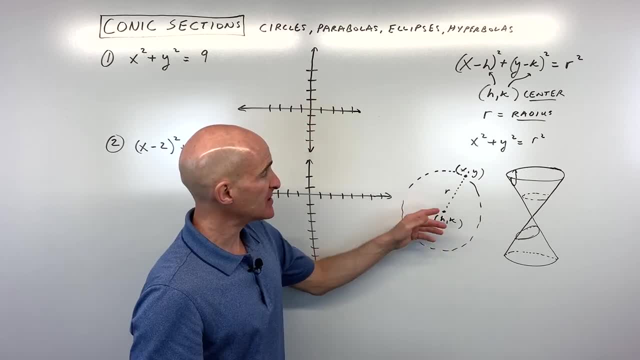 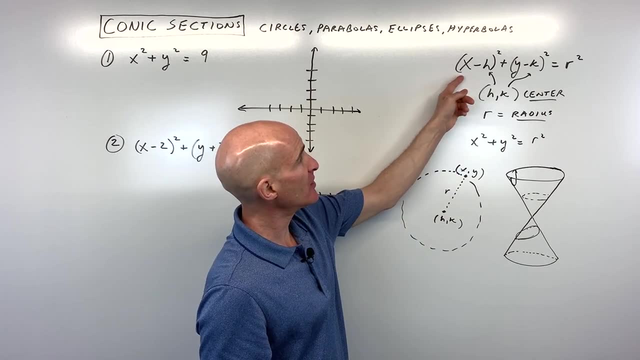 the radius. so we all know what a circle looks like, but basically what it is, it's always all these points that are that same distance from that h comma, k, center point, and the standard form for the equation of a circle is this one here: x minus h squared, plus y minus k squared. 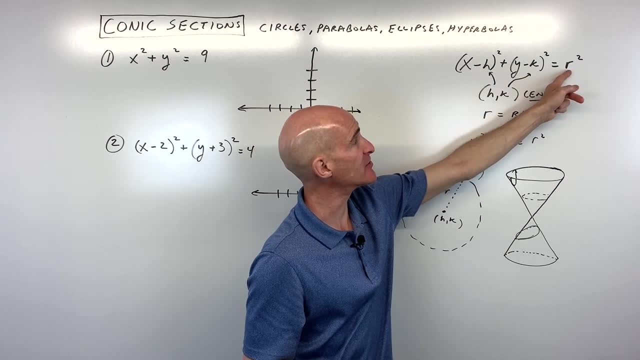 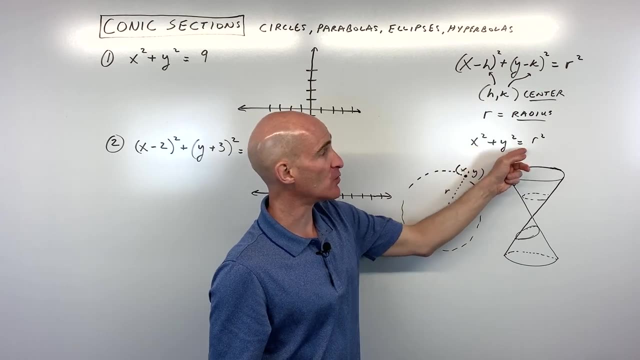 equals r squared. h comma k is the center and then r is the radius. of course, if the center is at the origin, h and k are zero. so then it collapses down to this form: x squared plus y squared equals r squared. let's look at two examples so you can see how this works. 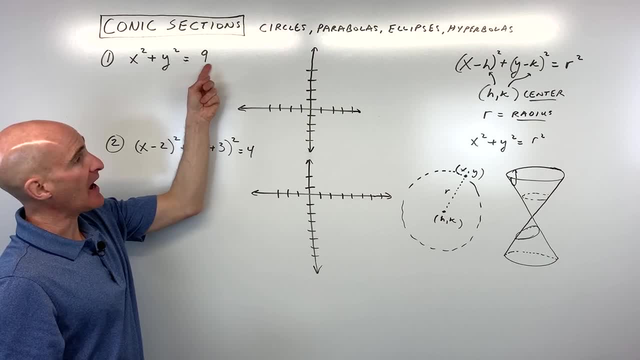 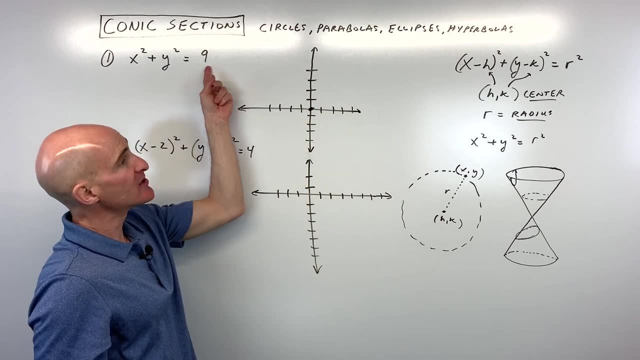 so for number one you can see: x squared plus y squared equals nine. so you can see that h is zero and k is zero. so that means that our center is here at zero, zero, the origin, and then notice that this is nine, which is really the radius squared. so if we take the square root of nine, 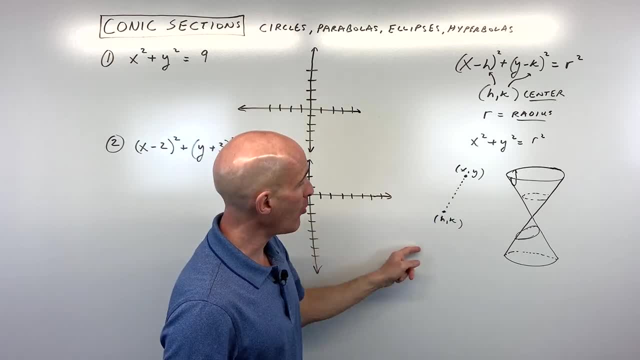 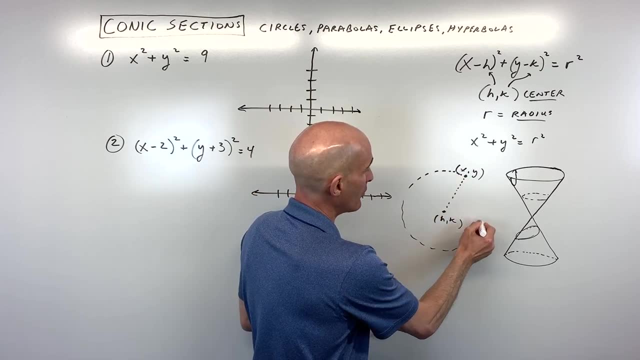 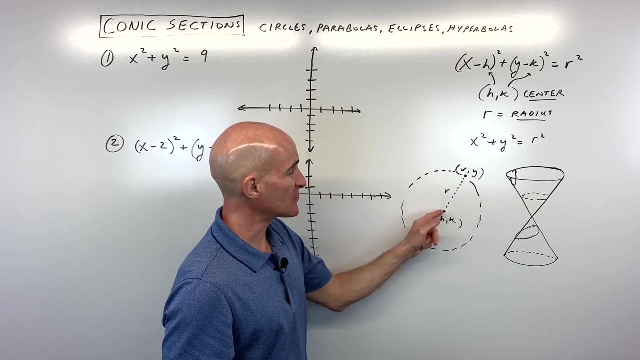 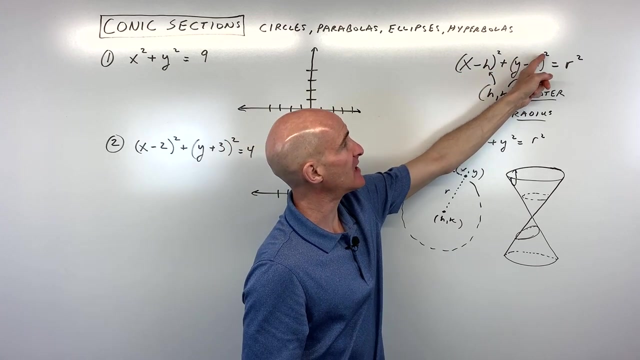 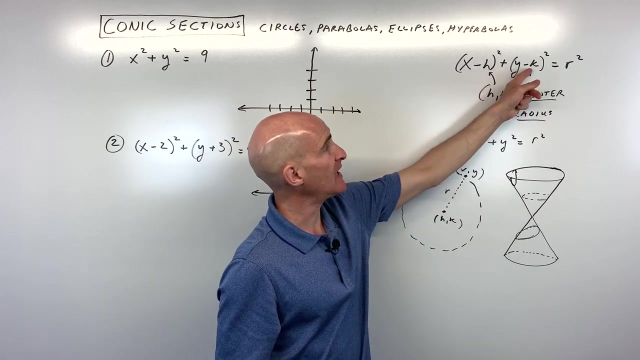 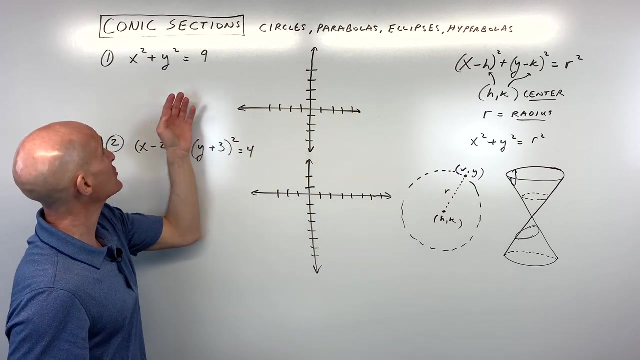 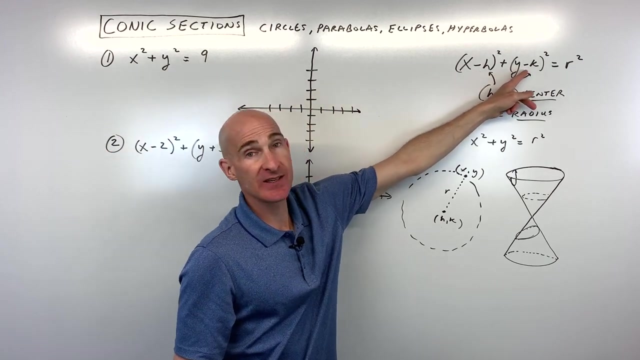 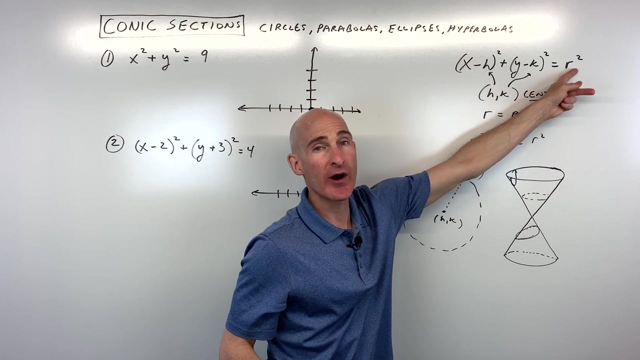 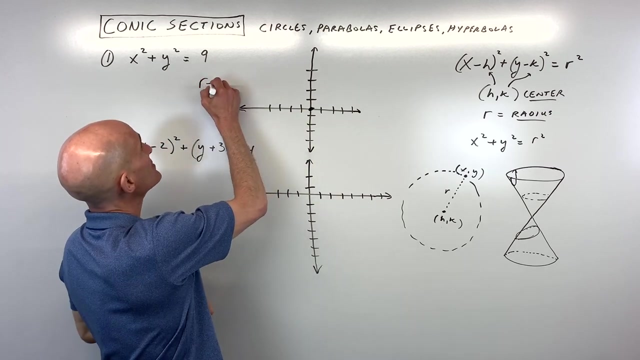 the circle what exactly is a circle it's a set of all points that are equidistant from a given point which we call the center okay and the distance from that center we call the the radius so we all know what a circle looks like but basically what it is it's always all these points that are that same distance from that h comma k center point and the standard form for the equation of a circle is this one here x minus h squared plus y minus k squared equals r squared h comma k is the center and then r is the radius of course if the center is at the origin h and k are zero so then it collapses down to this form x squared and then it collapses down to this form x squared plus y squared equals r squared let's look at two examples so you can see how this works so for number one you can see x squared plus y squared equals nine so you can see that h is zero and k is zero so that means that our center is here at zero zero the origin and then notice that this is nine which is really the radius squared so if we take the square root of nine that'll just give us r by itself the radius is three so now we know the radius is three and 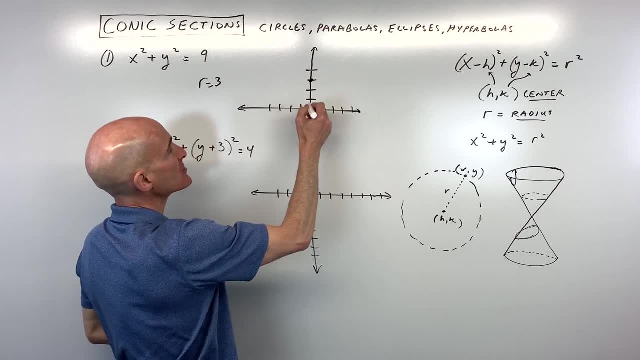 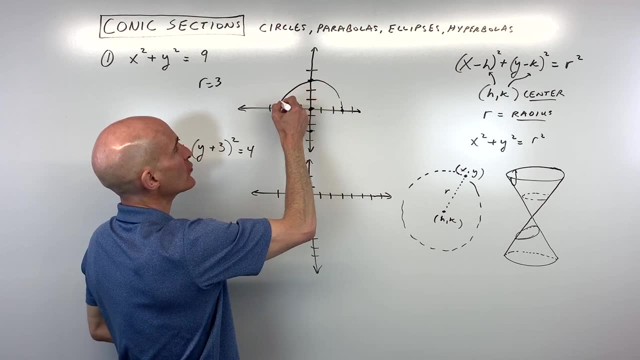 what you can do is from that center go up three units go down three units go left three units and go right three units and then you can just kind of draw a nice smooth curve through those points to get a good sketch of your circle let's look at a little bit more challenging 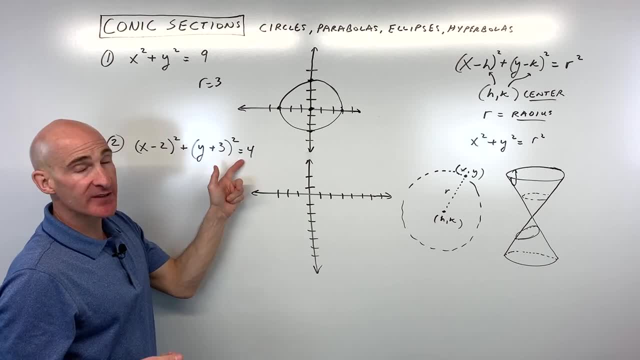 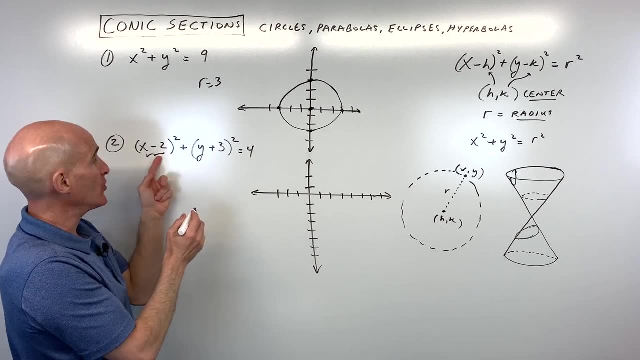 one now so for number two what do you think the center of this circle is well notice that this number here grouped with the x it looks like negative two it's actually the opposite positive 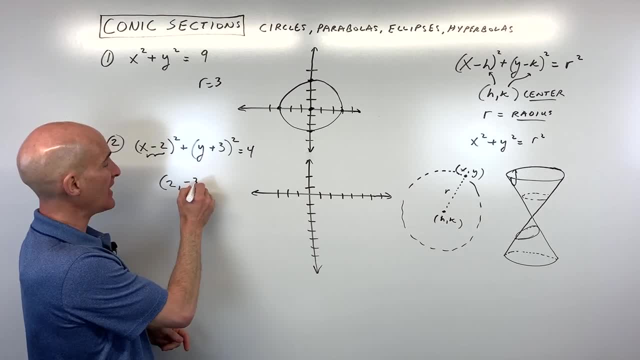 two this one looks like positive three it's actually negative three so you have to remember 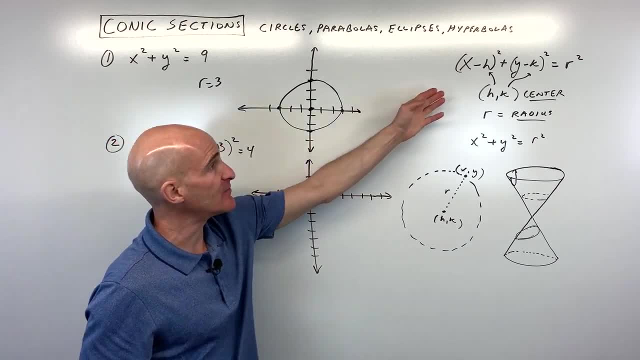 that these are the opposite signs and again it's not a positive three it's actually a negative three so you have to remember that these are the opposite signs and again it's actually the opposite three so you have to remember that these are the opposite signs and again it's because 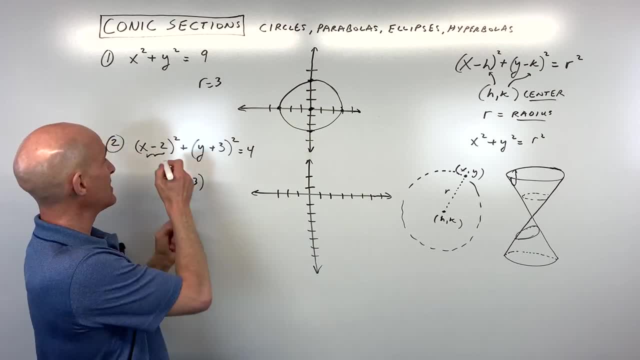 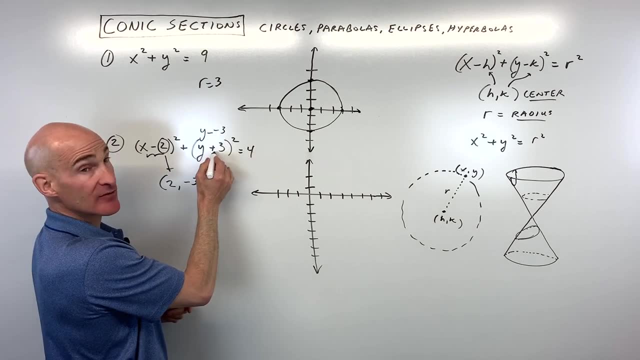 x minus h right see x minus see h is just a positive two this is really like y minus a negative three right because the two negatives give you this positive so you can see it's really 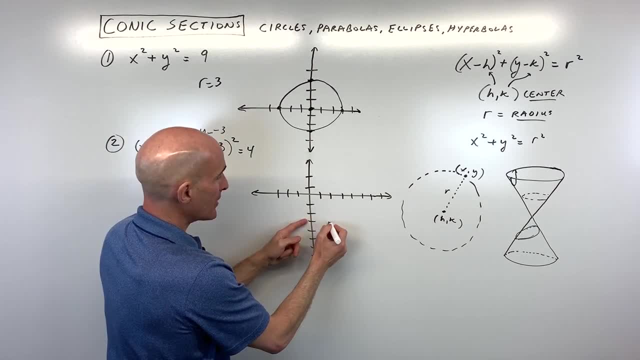 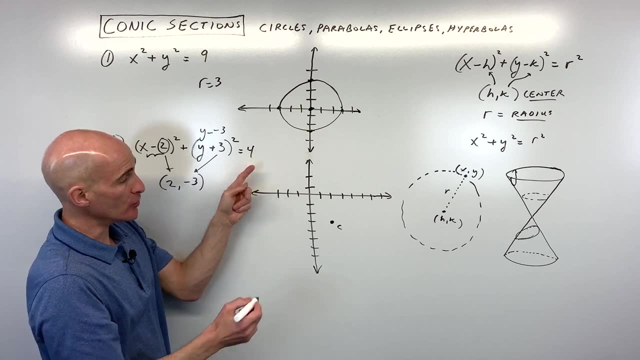 like the opposite sign so two comma negative three is our center point so let's go ahead and plot that and then the radius because this is uh r squared we have to take the square root of four which is two so from the center i'm going to go up two i'm going to go left two i'm going to go down 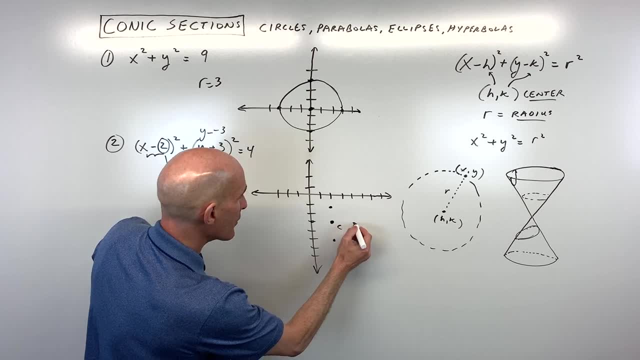 and i'm going to go right to which is right about there and if we sketch a smooth curve 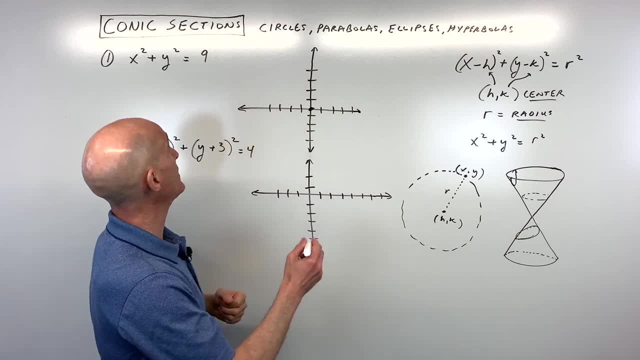 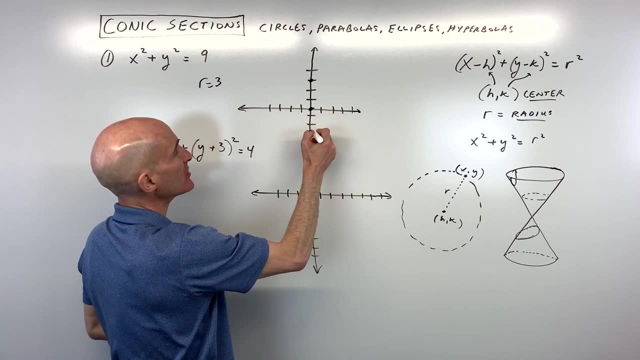 that'll just give us r by itself. the radius is three. so now we know the radius is three and what you can do is, from that center, go up three units, go down three units, go left three units and go right three units, and then you can just kind of 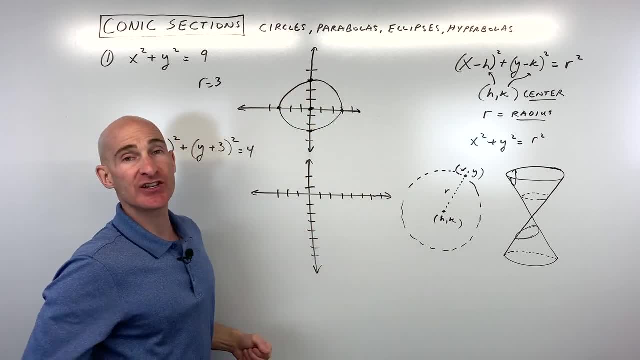 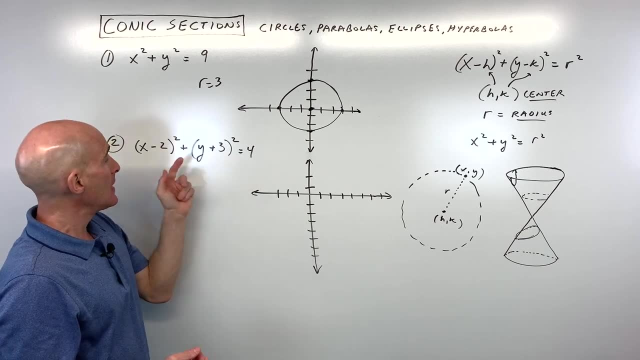 draw a nice smooth curve through those points to get a good sketch of your circle. let's look at a little bit more challenging one now. so for number two, what do you think the center of this circle is? Well, notice that this number, here, grouped with the x, it looks like negative. 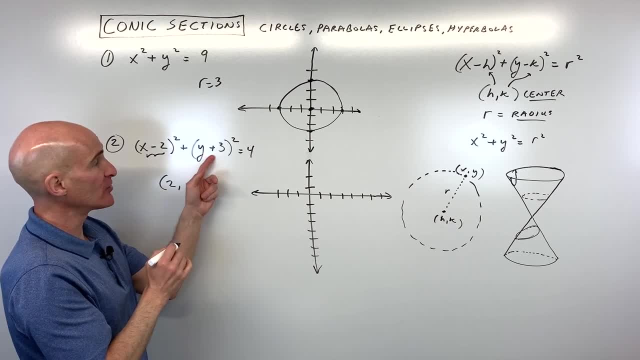 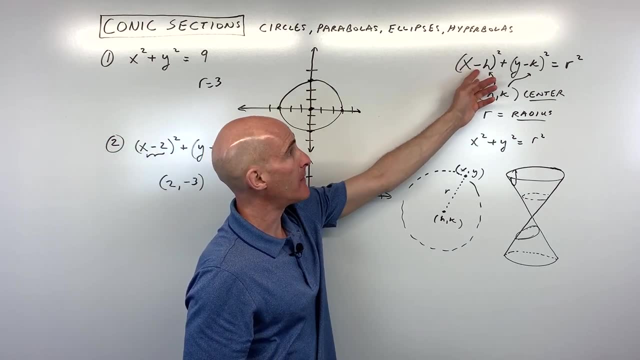 two: it's actually the opposite. positive two: this one looks like positive three, It's actually negative three. so you have to remember that these are the opposite signs, because x minus h- right, See x minus see h- is just a positive two. 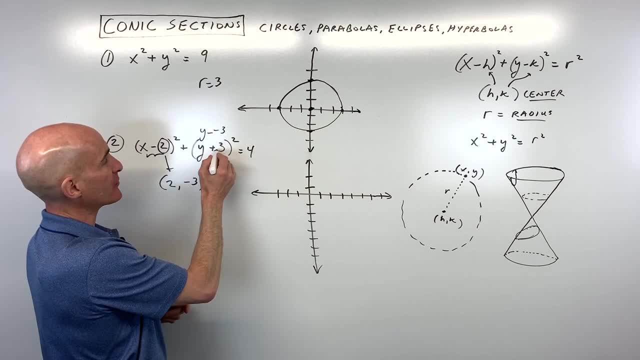 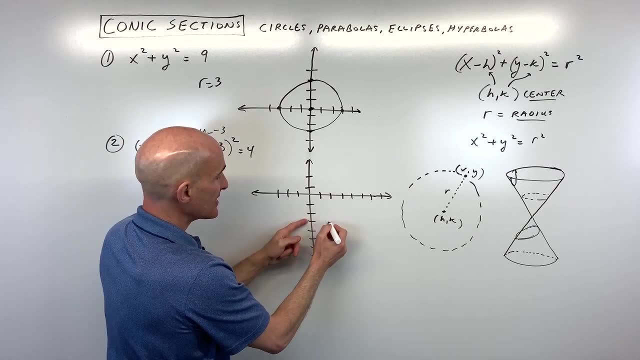 This is really like y minus a negative three. right Cause the two negatives give you this positive. So you can see it's really like the opposite sign. So two comma, negative three is our center point. So let's go ahead and plot that. 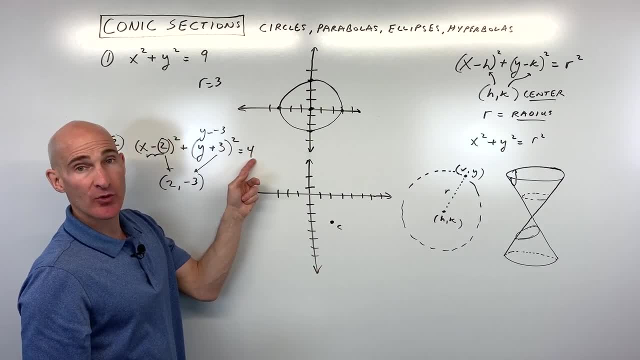 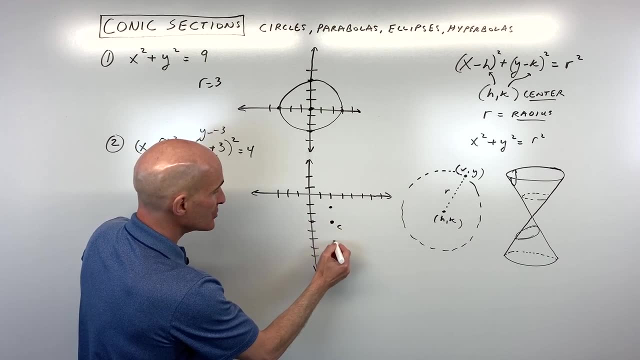 And then the radius, because this is our square. we have to take the square root of four, which is two. So from the center I'm gonna go up two, I'm gonna go left two, I'm gonna go down two. 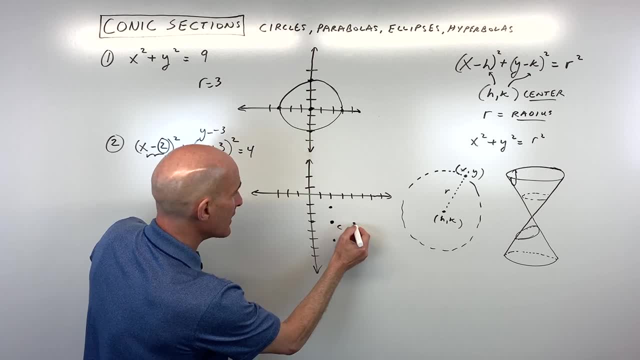 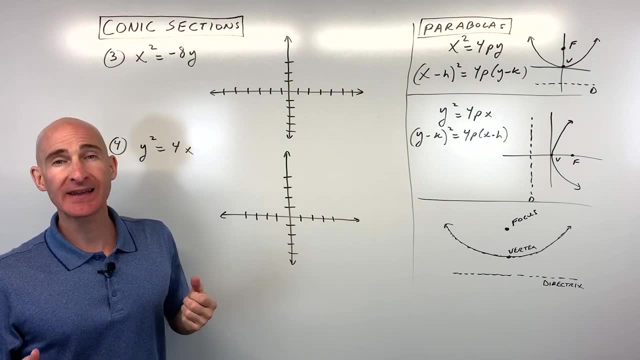 And I'm gonna go right two, which is right about there, And if we sketch a smooth curve, we've got a good graph. Okay, now let's talk about parabolas. So what exactly is a parabola? Well, technically speaking, what a parabola is? 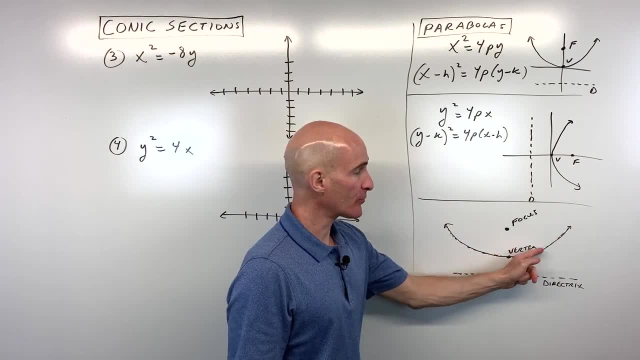 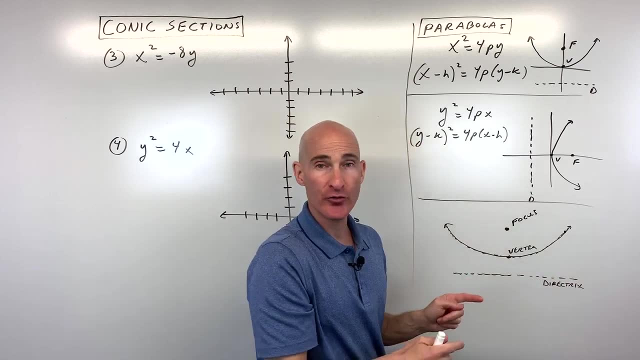 it's the set of all these points, okay, along the parabola, such that they're equidistant from a given point called the focus and a given line called the directrix. So, for example, if I was to pick a point right here, okay. 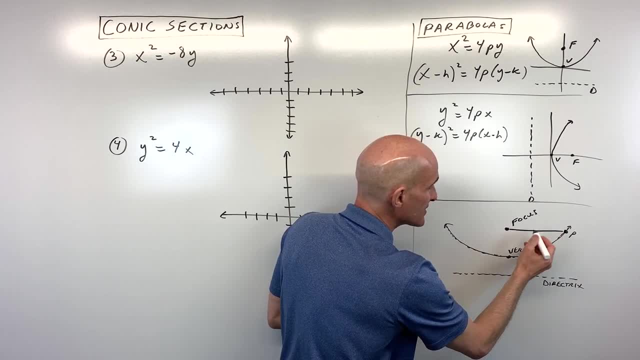 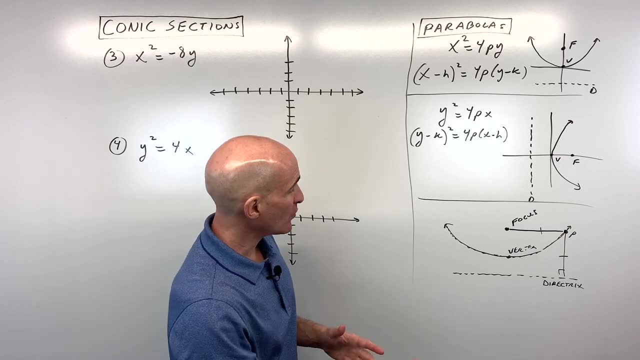 let's just call that P. if we measure that distance to the focus, that distance has to be the same distance as the perpendicular or the shortest distance to the directrix. Now kind of imagine what happens like, for example, as you go further out on the parabola. 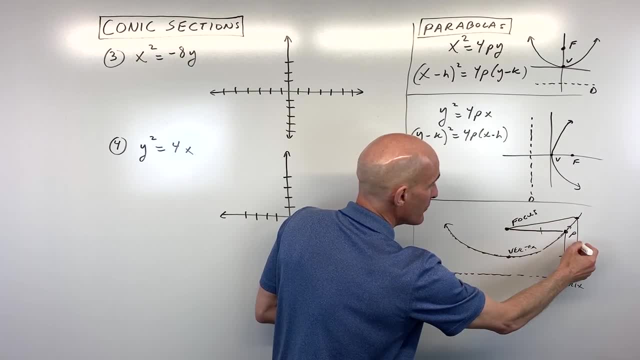 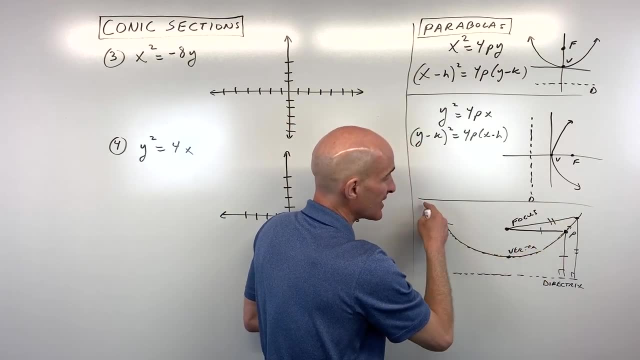 like say, if I pick a point here, this distance is getting longer, but so is that perpendicular distance to the directrix. But those lengths or distances are always gonna be the same. So that's what makes up this set of points along the parabola. 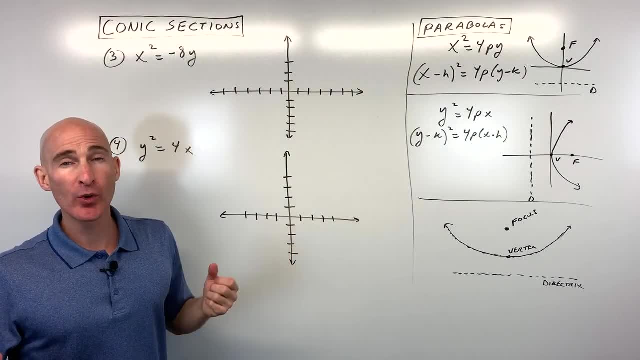 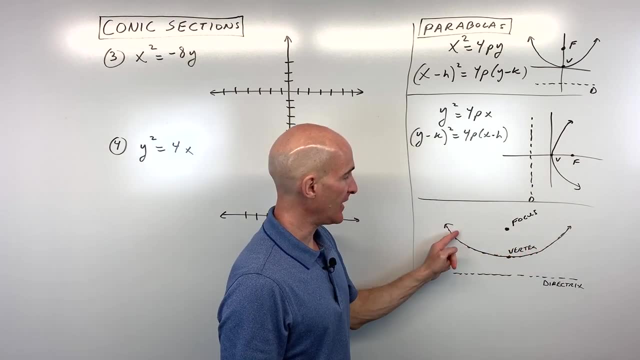 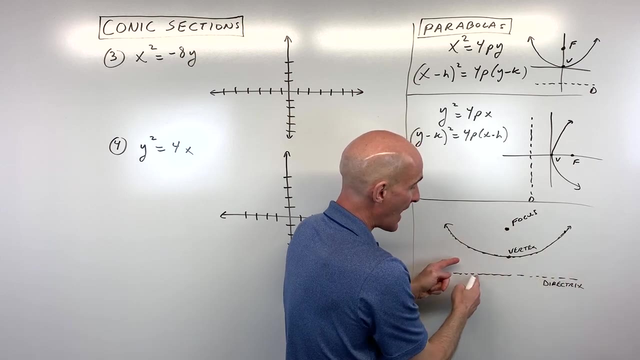 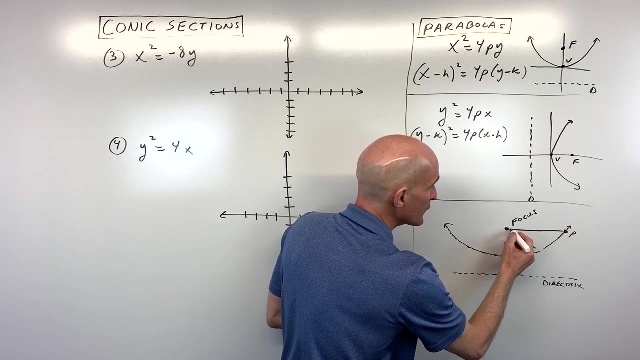 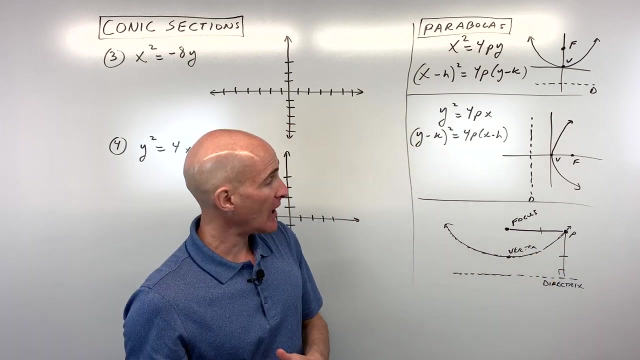 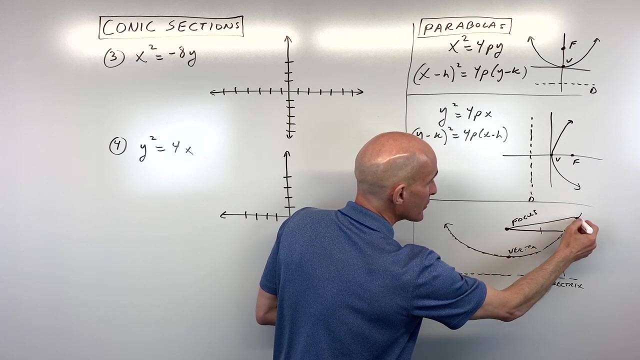 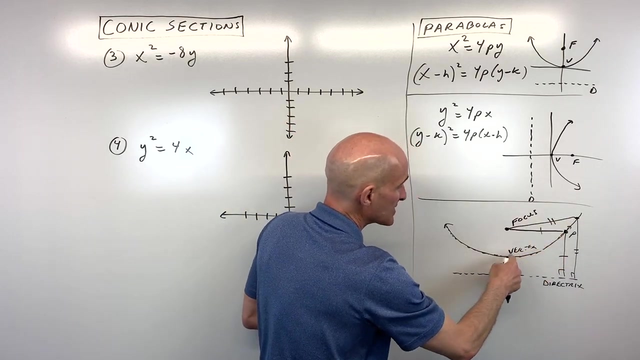 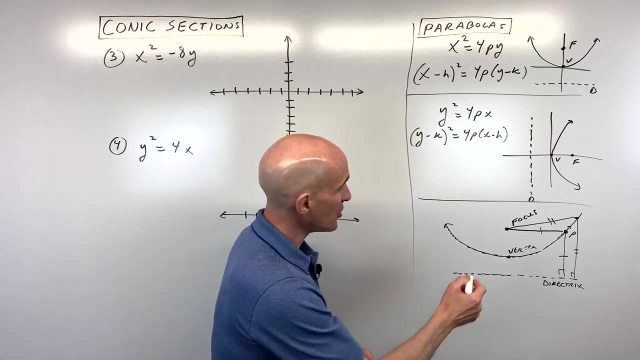 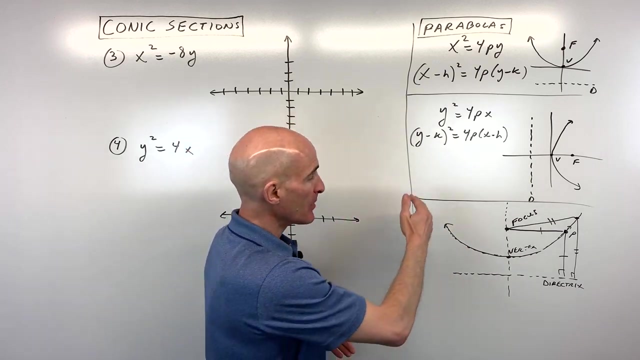 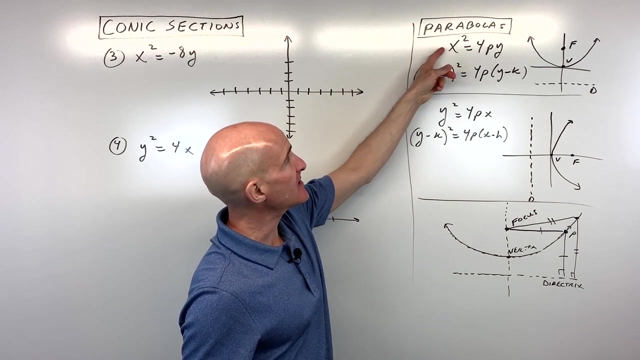 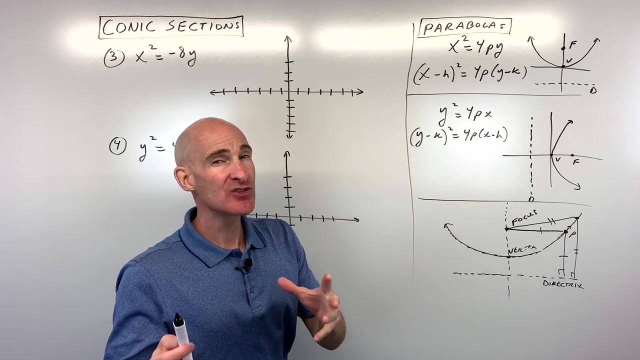 we've got a good graph okay now let's talk about parabolas so what exactly is a parabola well technically speaking what a parabola is it's the set of all these points okay along the parabola such that they're equidistant from a given point called the focus and a given line called the directrix so for example if i was to pick a point right here okay let's just call that p if we measure that distance to the focus that distance has to be the same distance as the perpendicular or the shortest distance to the directrix now kind of imagine what happens like for example as you go further out on the parabola like say if i pick a point here this distance is getting longer but so is that perpendicular distance to the directrix but those lengths or distances are always going to be the same so that's what makes up this set of points along the parabola but some key points are the focus the vertex and the directrix there's also this axis right here okay such that if you fold it over that axis the parabola is going to match with itself but essentially we're looking at this u-shaped graph which we call a parabola now there's a couple different types there's this type here where it's in the x squared equals 4py form and this one the y squared equals 4px form sometimes students get these a little bit confused i want to kind of make this simple for you when you see that the x term is squared you know that 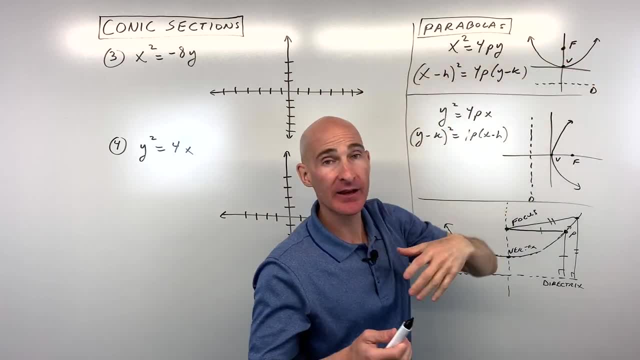 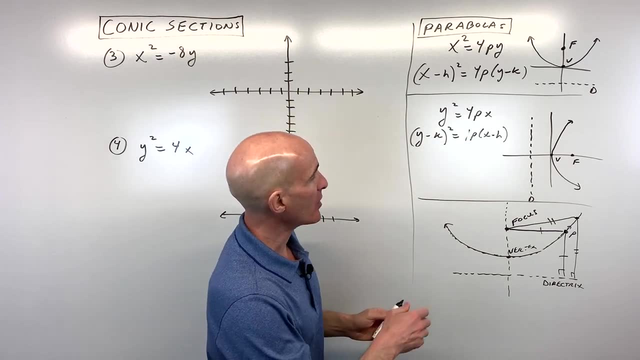 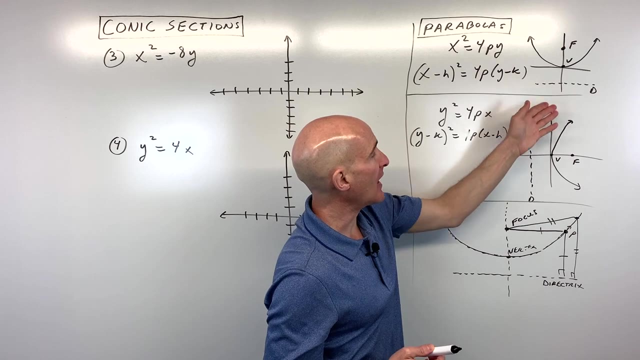 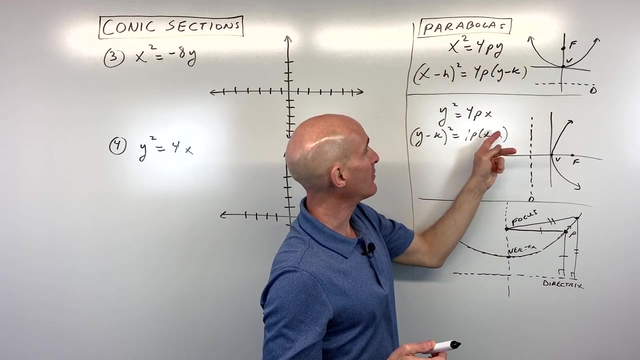 the parabola is going to be opening up or down kind of like y equals x squared you probably learned about previously but in the y squared term is squared right the y term is squared then it's going to be opening to the right or to the left okay now the next thing is how do you know if it's opening up or down right or left well if it's opening up this coefficient here is going to be positive if it's negative it's going to be opening down over here if this is positive it's going to be opening to the right 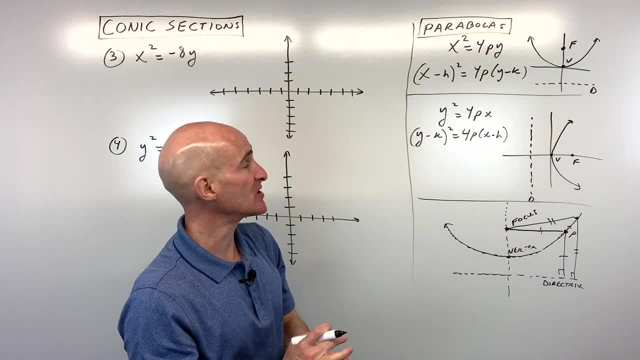 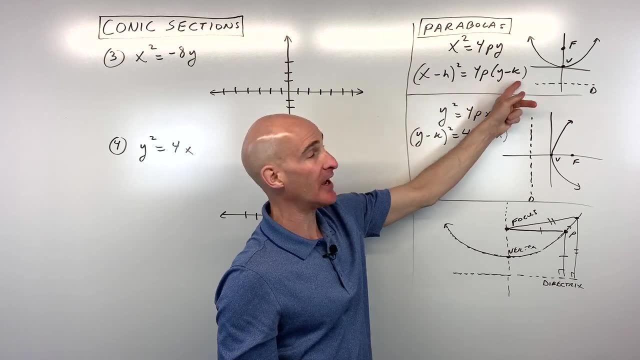 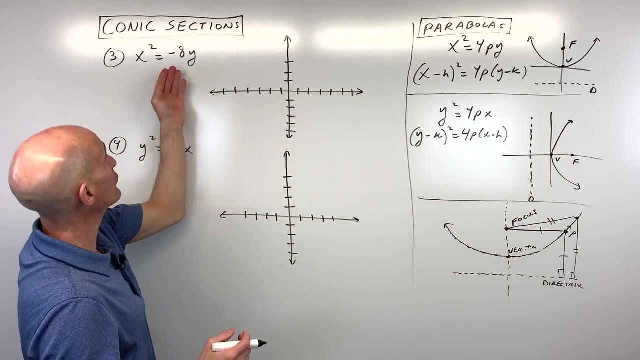 if this quantity is negative it's going to be open to the left we're going to go through examples so how this works but here you can see that the vertex to this point right here where the graph bends that's going to be h comma k okay so if there's not an h and a k that means that the vertex is at the origin so let's look at a couple examples we'll talk about it as we go through it so for number three x squared equals negative eight y we can see it's an x squared type that's 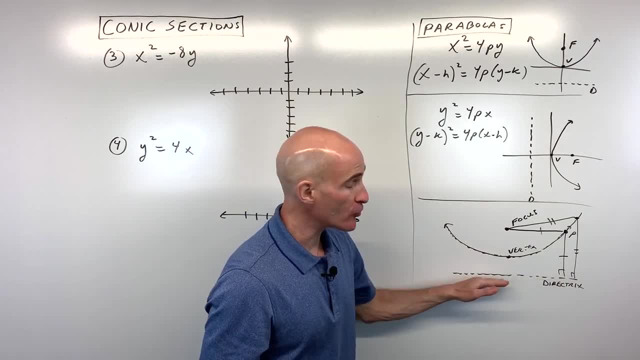 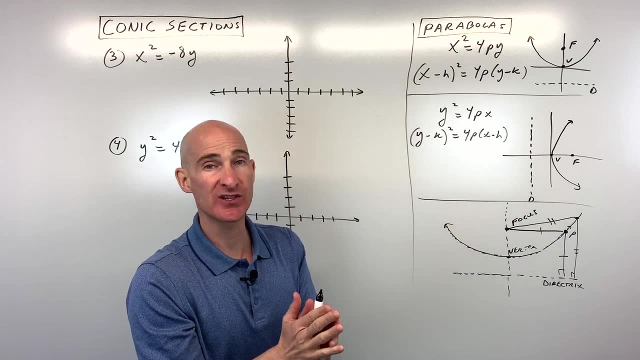 But some key points are the focus, the vertex and the directrix. There's also this axis right here, okay, such that if you fold it over that axis, the parabola is gonna match with itself. But essentially we're looking at this U-shaped graph. 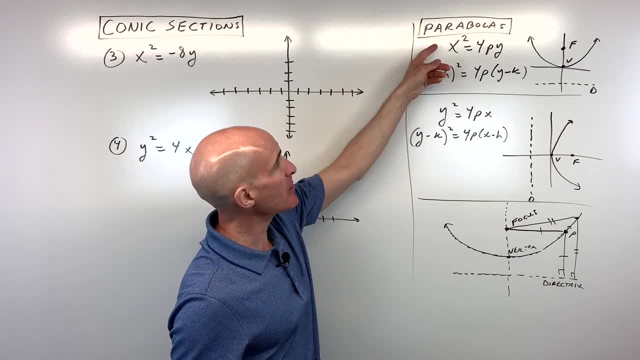 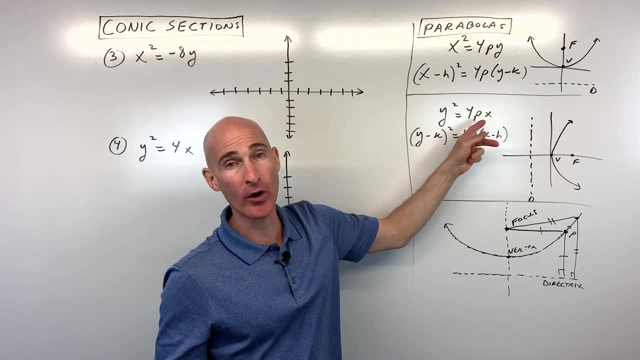 which we call a parabola. Now, there's a couple different types. There's this type here, where it's in the X squared equals four P Y form, and this one, the Y squared equals four P X form. Sometimes students get these a little bit confused. 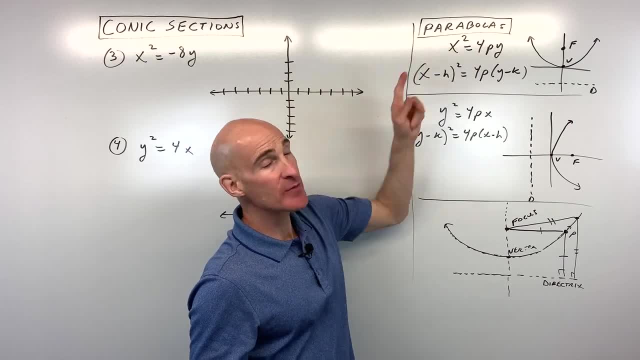 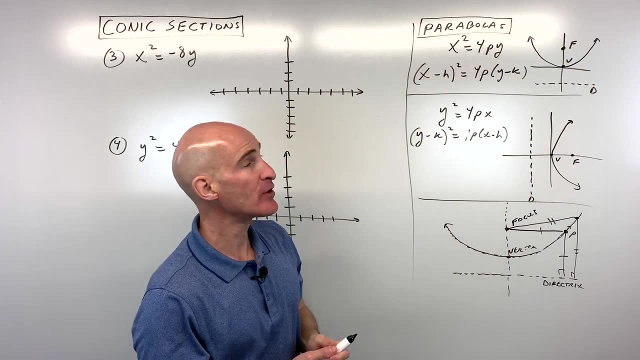 So I wanna kind of make this simple for you. When you see that the X term is squared, you know that the parabola is gonna be opening up or down, kind of like Y equals X squared. you probably learned about previously. But when the Y squared term is squared, right. 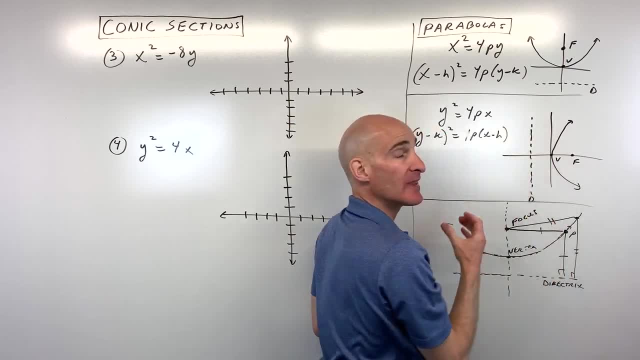 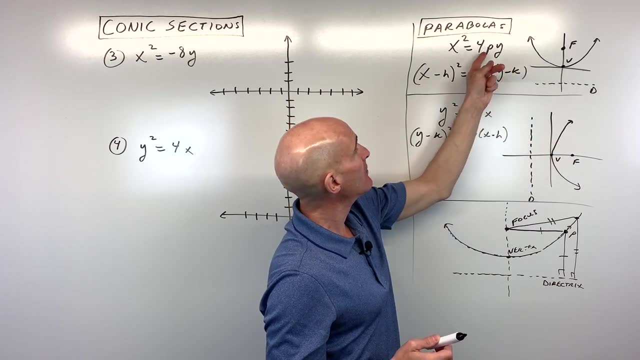 the Y term is squared, then it's gonna be opening to the right or to the left. Okay, now the next thing is: how do you know if it's opening up or down, right or left? Well, if it's opening up, 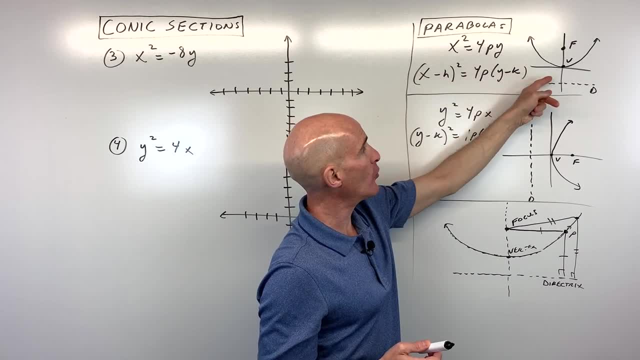 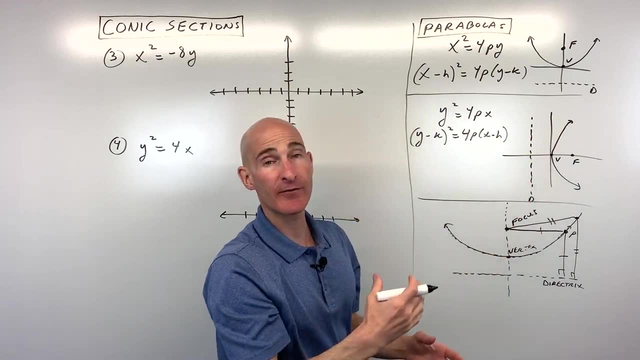 this coefficient here is gonna be positive. If it's negative, it's gonna be opening down Over here. if this is positive, it's gonna be opening to the right. If this quantity is negative, it's gonna be opening to the left. 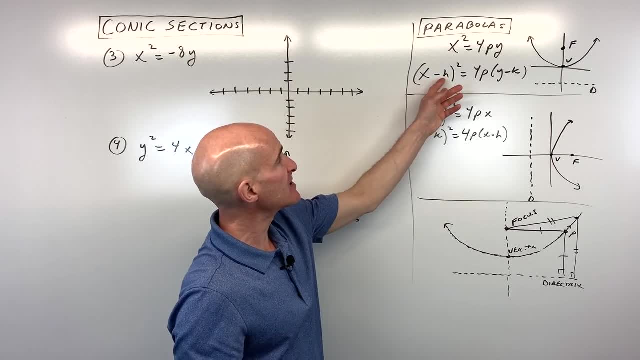 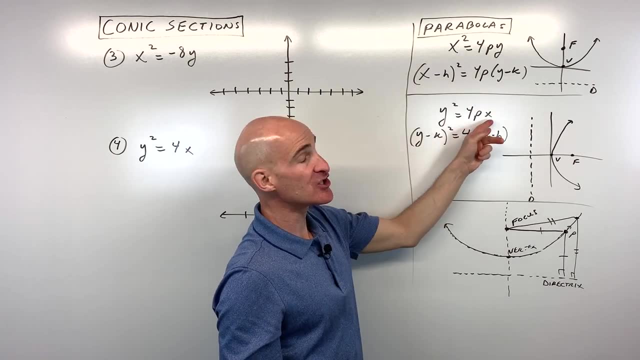 And we're gonna go through examples so you can see how this works. But here you can see that the vertex, okay, this point right here, where the graph bends, that's gonna be H comma K. Okay, so if there's not an H and a K, 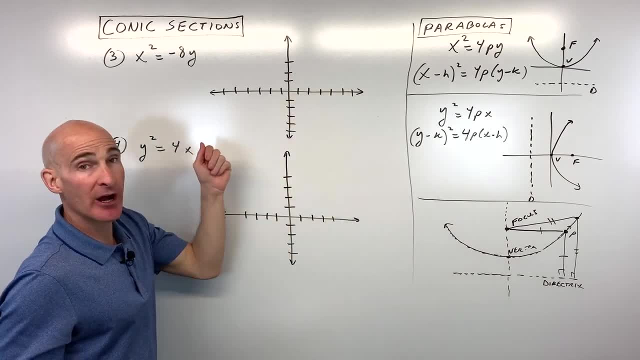 that means that the vertex is at the origin. So let's look at a couple examples. We'll talk about it as we go through it. So for number three, X squared equals negative eight Y. We can see it's an X squared type. 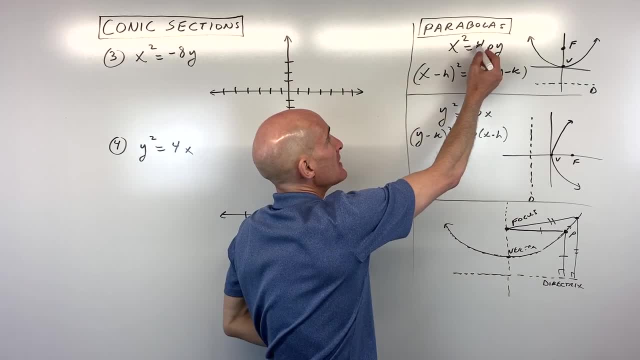 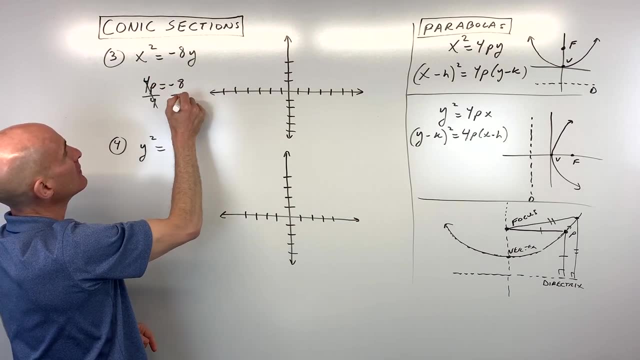 That's this type here, okay, And if we take four P, okay, and set it equal to negative eight, let's do that- Divide by four, You can see that P is coming out to negative two, Okay. so now what we're gonna do is: 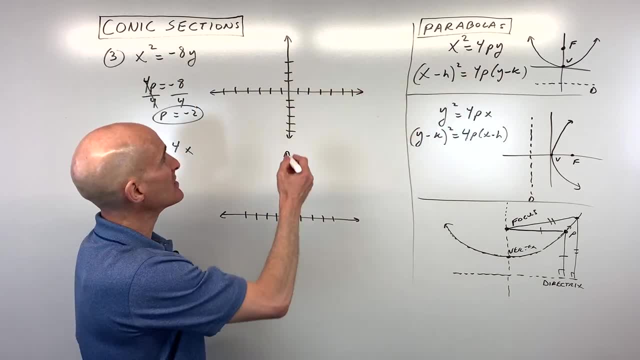 we can see that this hasn't shifted at all. There's not an H or a K, So that means that the vertex is right here. at the origin It's X squared. We know it's opening up or down, But because this is negative, 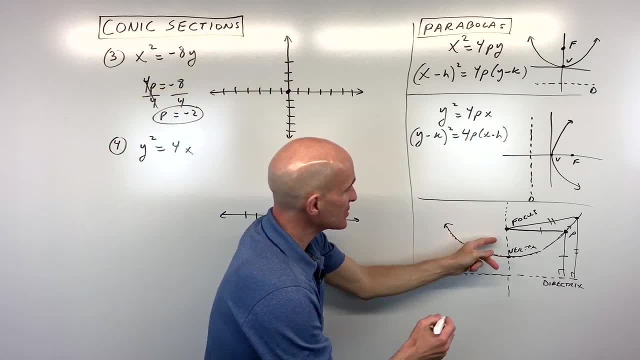 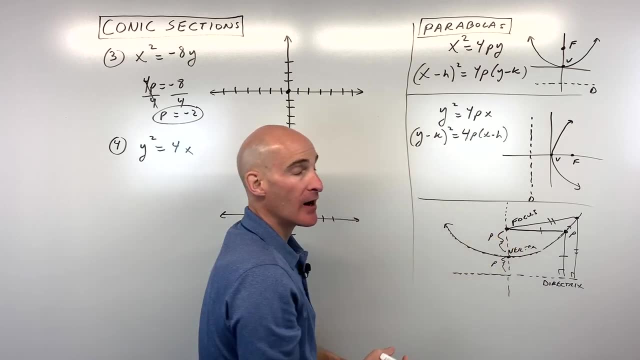 we know it's gonna open down The P value is this distance right here between the vertex and the focus, Also the distance between the vertex and the directrix. That's also that same length of P. So here we're gonna be going down two. 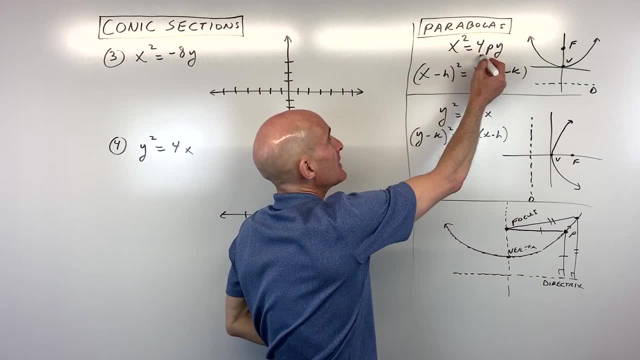 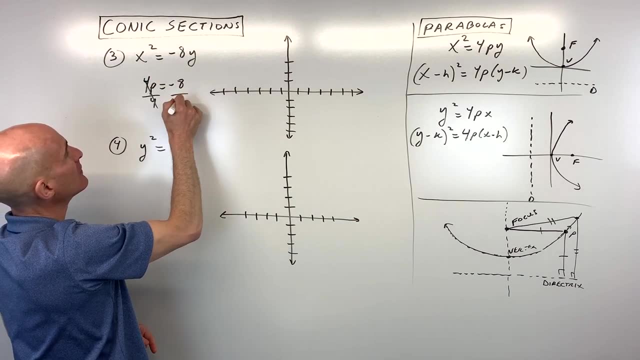 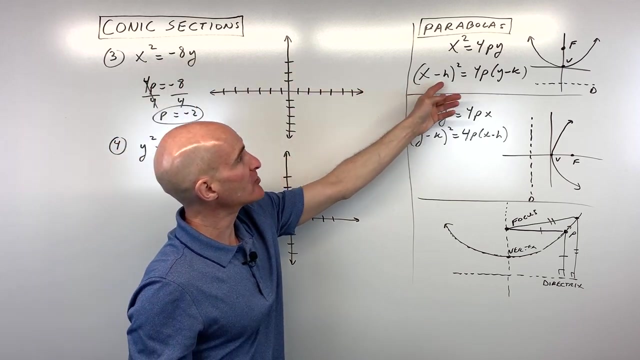 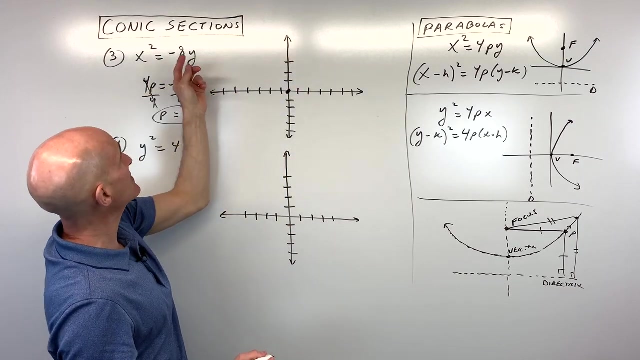 this type here okay and if we take 4p okay and set it equal to negative eight let's do that divide by you can see that p is coming out to negative two okay so now what we're going to do is we can see that this hasn't shifted at all there's not an h or a k so that means that the vertex is right here at the origin it's x squared we know it's opening up or down but because this is negative we know 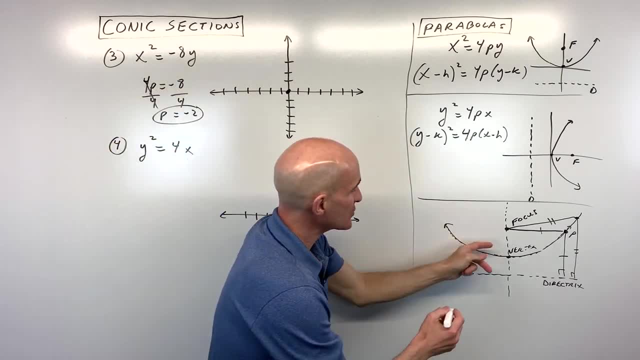 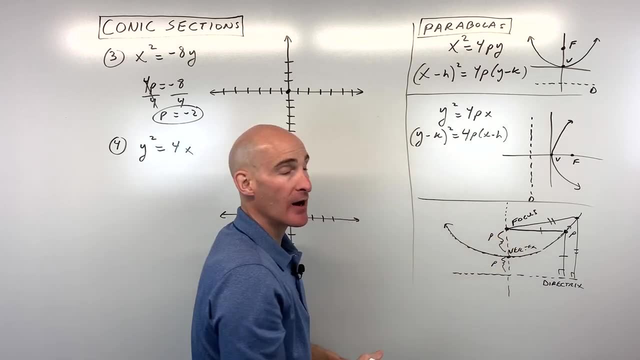 it's going to open down the p value is this distance right here between the vertex and the focus also the distance between the vertex and the directrix that's also that same length of p so here we're going to be going down two 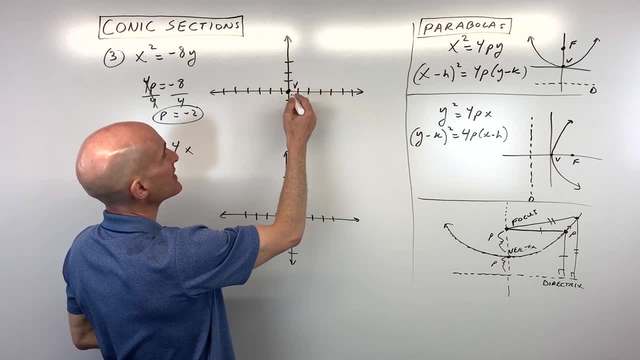 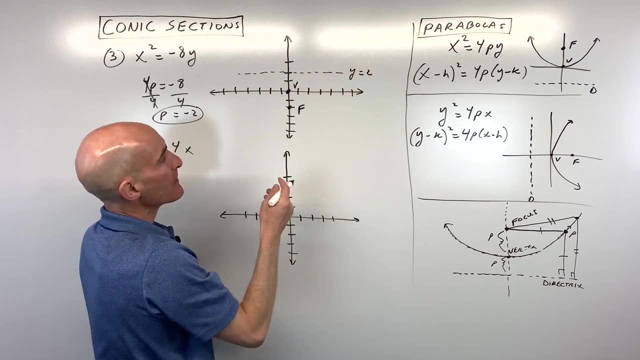 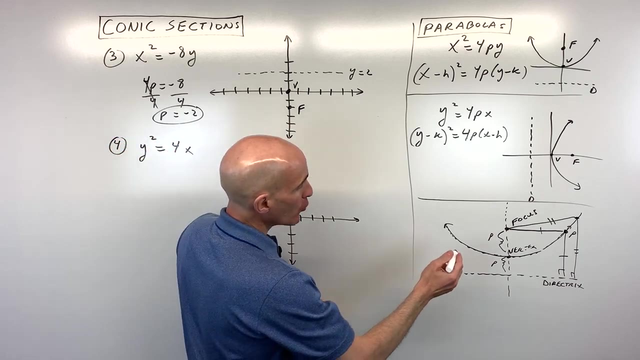 okay so that's going to be your focus this is your vertex and if i go up two this is where your directrix is going to be right here so this is the line y equals two now i want to show you another way to get a couple more points very easily there's something called a focal cord 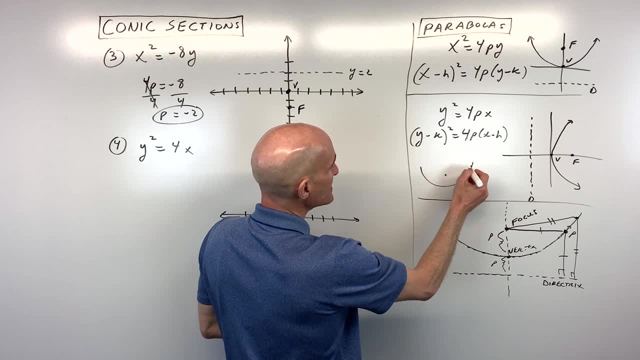 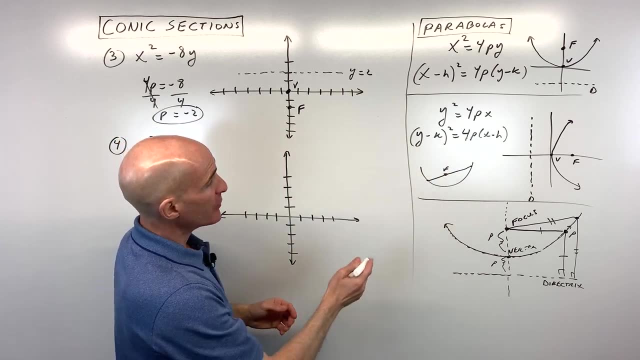 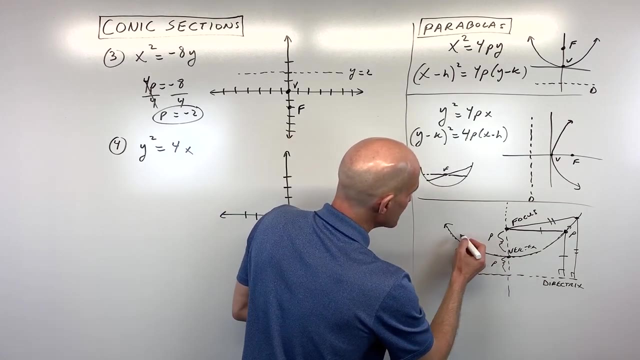 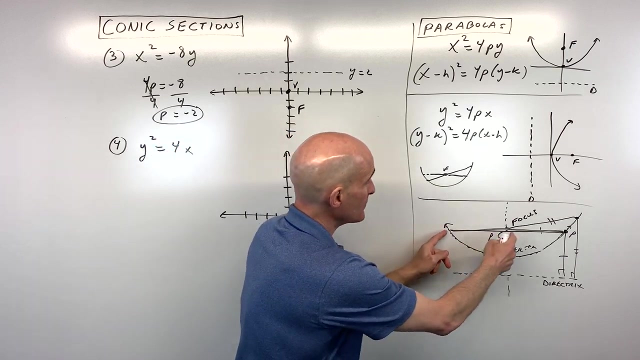 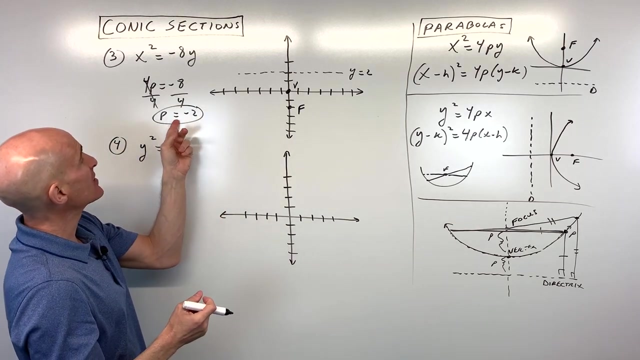 and what a focal cord is is if you take two points on a parabola and if you connect them and that segment goes through the focus they call that a focal cord but the focal cord is more of one peról that's perpendicular to the axis of symmetry like for example if i was to draw it in on this one right here this length right here is going to be four p it's going to be four times the length of p they call that the lattice rectum it's a special focal cord 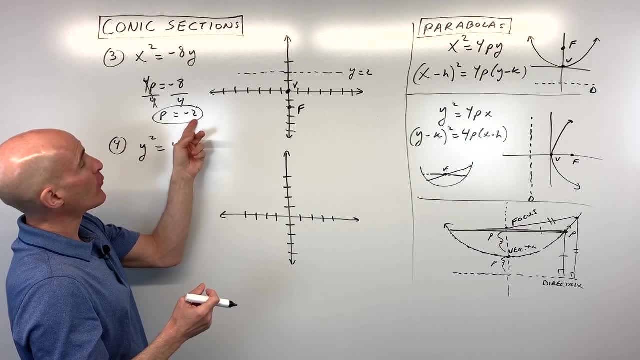 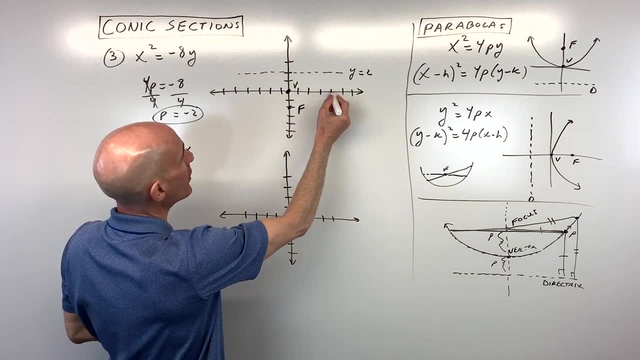 and so in this case because p is two okay negative two four times that is going to be the width of the parabola at the level of the focus so for example here it's going to be eight so i'm going to need a So I'm going to go right 4, and I'm going to go left 4 at the level of the focus. 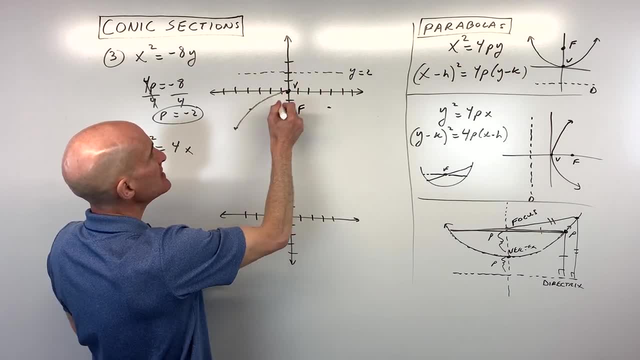 So that gives me a width of 8, and that's just a couple of easy points to get a good sketch of your parabola. 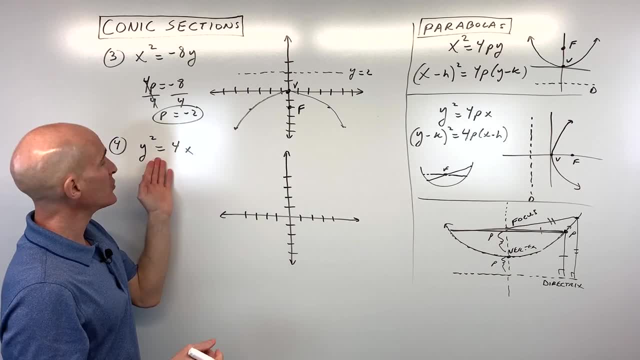 So let's go ahead and take a look at another example. You'll see how this works as we go through them. I'm going to do a few more. 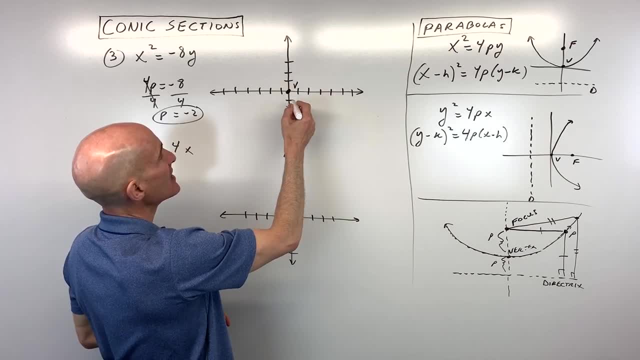 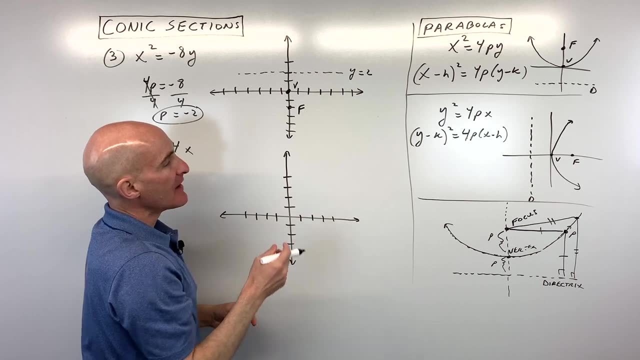 Okay, so that's gonna be your focus. This is your vertex, And if I go up two, this is where your directrix is gonna be right here. So this is the line. Y equals two. Now I wanna show you another way. 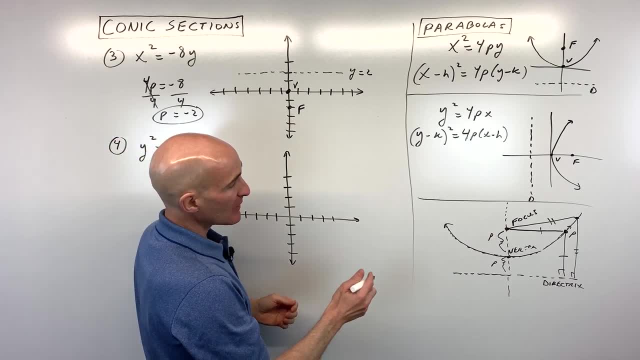 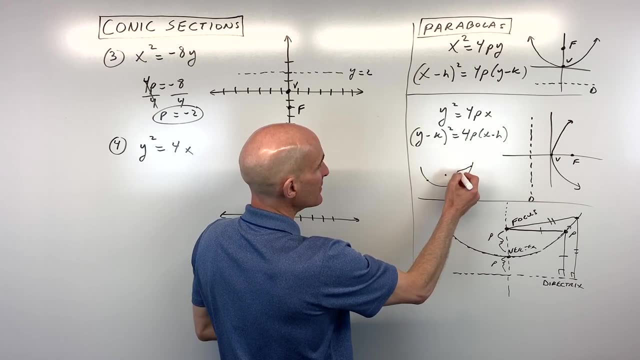 to get a couple more points very easily. There's something called a focal chord, And what a focal chord is is if you take two points on a parabola and if you connect them and that segment goes through the focus. they call that a focal chord. 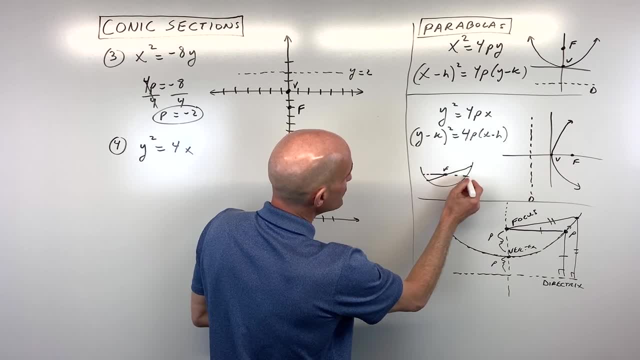 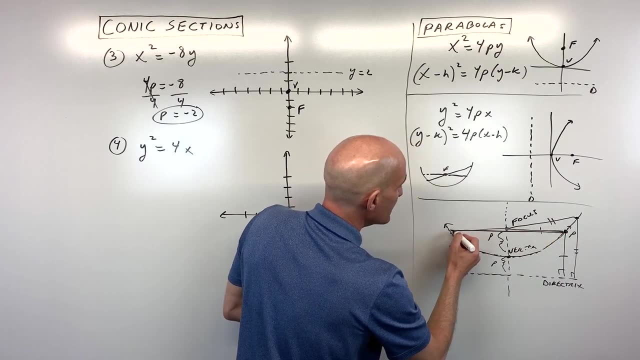 But the focal chord that's perpendicular to the axis of symmetry, like, for example, if I was to draw it in on this one right here, this length right here is gonna be four P, It's gonna be four times the length of P. 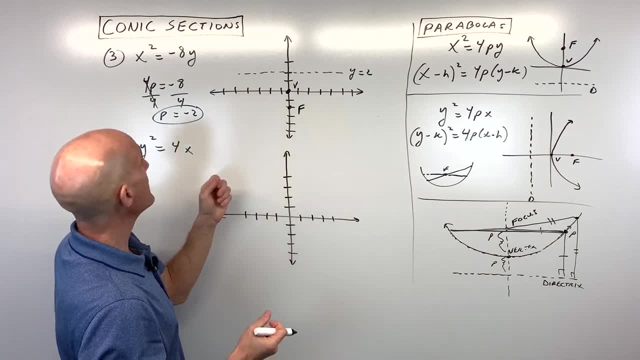 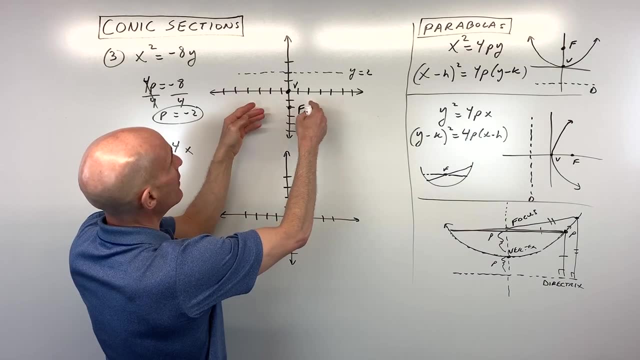 They call that the lattice rectum. It's a special focal chord And so in this case, because P is two, okay, negative two, four times that is gonna be the width of the parabola At the level of the focus. 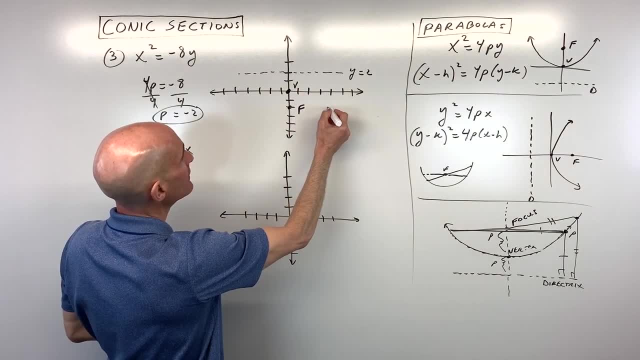 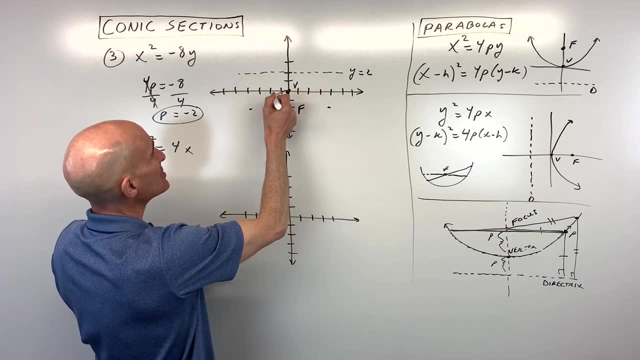 So, for example, here it's gonna be eight. So I'm gonna go right four and I'm gonna go left four at the level of the focus. So that gives me a width of eight. And that's just a couple of easy points. 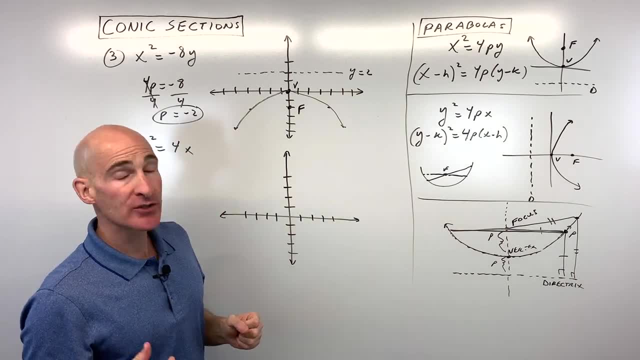 to get a good sketch of your parabola. So let's go ahead and take a look at another example. You'll see how this works as we go through them. I'm gonna do a few more. So number four: we've got Y squared equals four X. 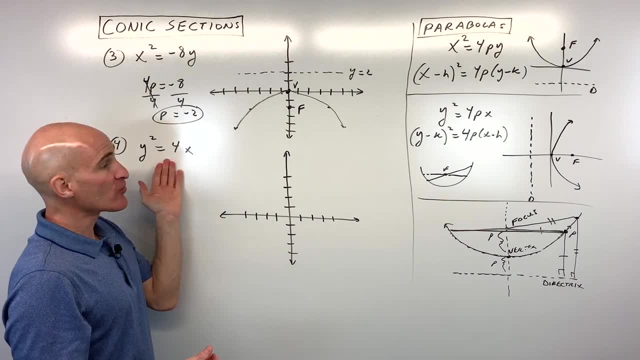 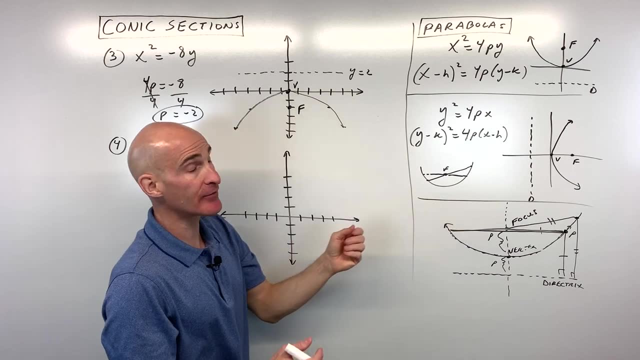 So the first question you wanna ask yourself is: does a graph open? Does it open up down, left or right? So what do you think? Well, it's Y squared. So we know it's gonna open to the right or to the left. 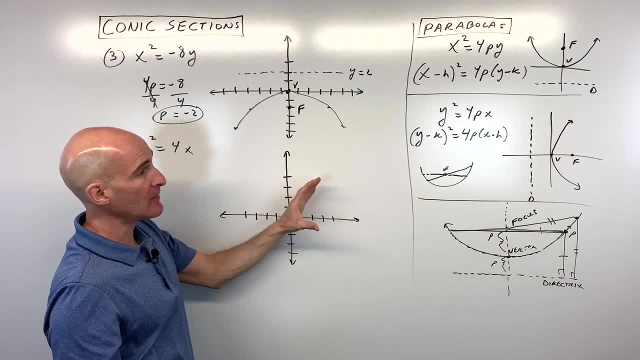 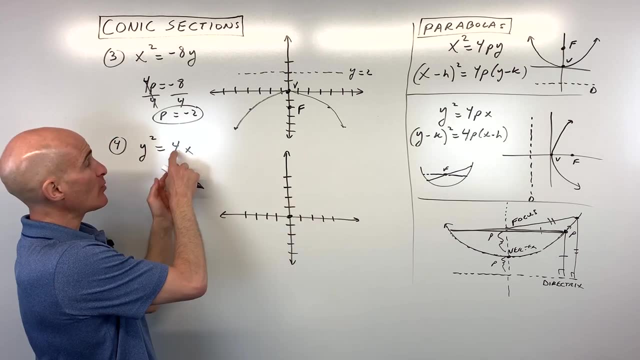 This coefficient here is positive, So we know it's gonna be opening to the right, So that we've got that part down. It hasn't shifted at all, So we know our vertex is gonna be right here at the origin. The next thing we wanna figure out is: what is this P value? 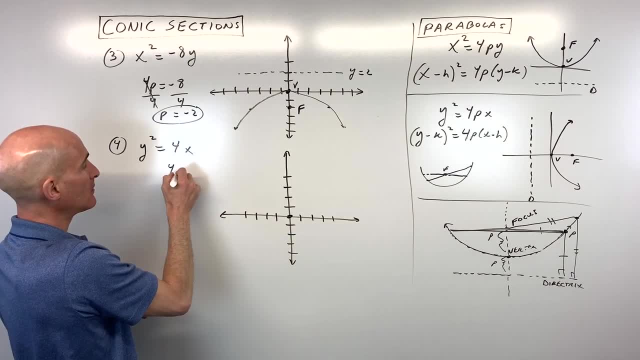 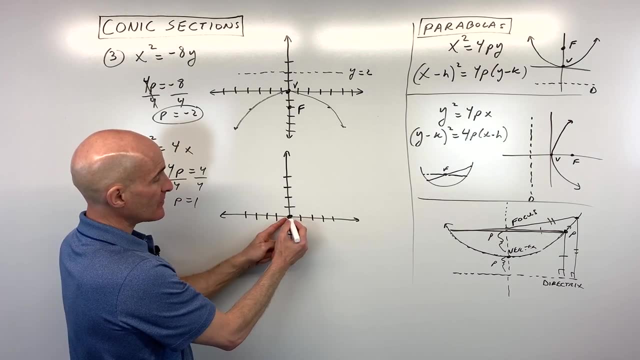 So if we take four P and set it equal to four, divide both sides by four, you can see that P is equal to one. So from the vertex I'm gonna go right one, That's our focus, And if I go left, one. 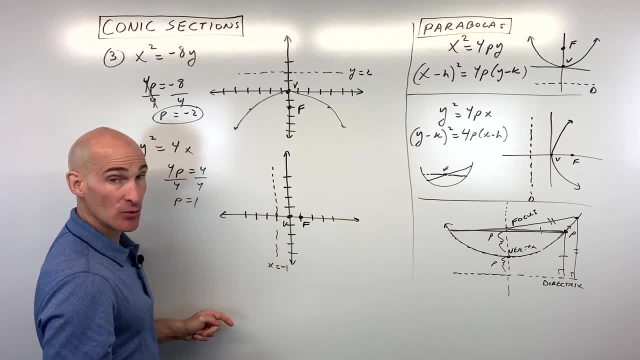 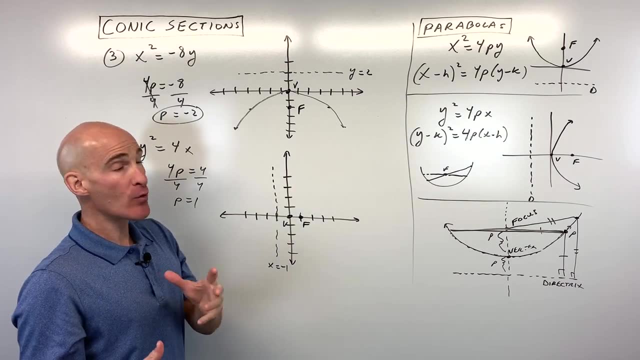 that's gonna be our directrix, which in this case is: X equals negative one, okay, Vertical lines, or X equals lines. So now we know the parabola is gonna look something like that. The only other thing is to get a few more points. 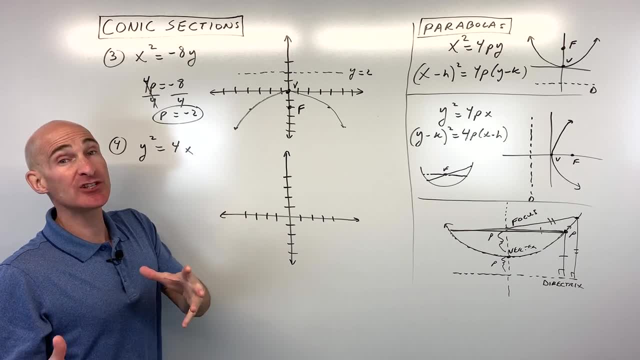 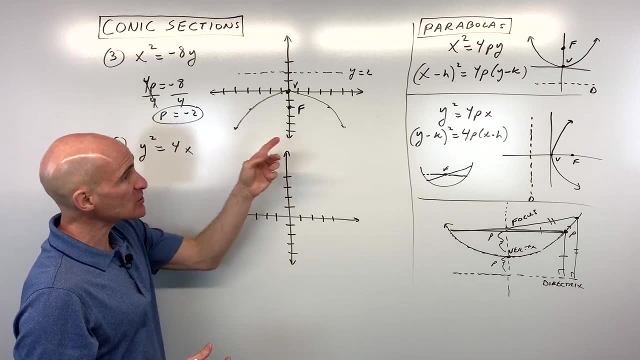 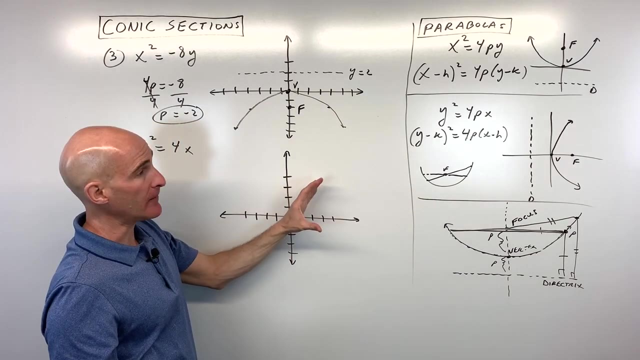 So number 4, we've got y squared equals 4x. So the first question you want to ask yourself is, you know, does a graph open up, down, left, or right? So what do you think? Well, it's y squared, so we know it's going to open to the right or to the left. This coefficient here is positive, so we know it's going to be opening to the right. So we've got that part down. 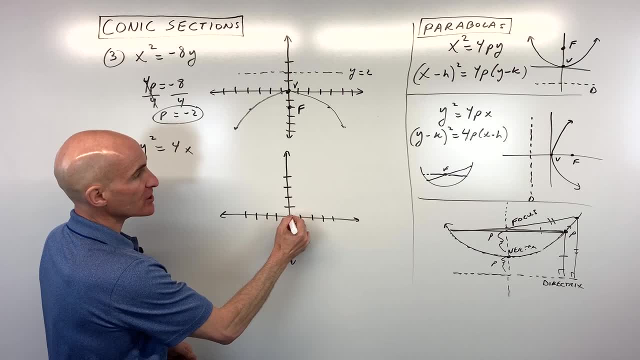 It hasn't shifted at all, so we know our vertex is going to be right here at the origin. 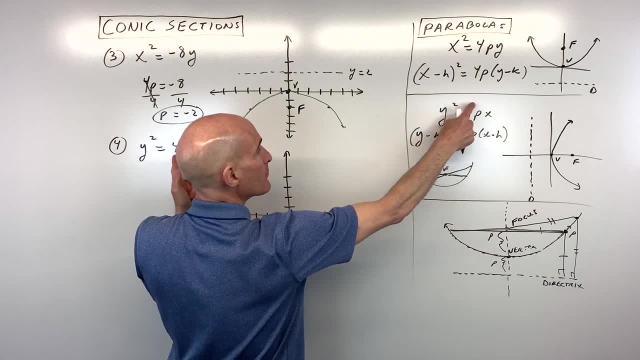 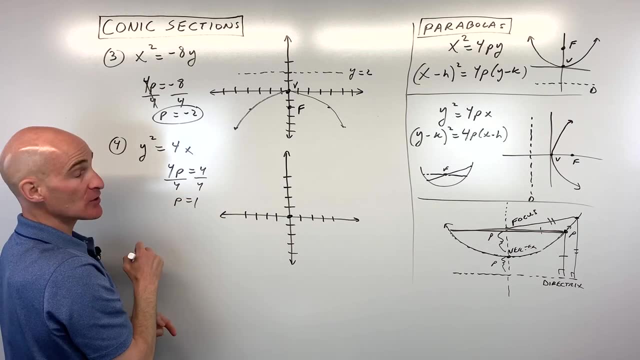 The next thing we want to figure out is what is this p value? So if we take 4p and set it equal to 4, divide both sides by 4, you can see that p is equal to 1. So from the vertex, I'm going to go right 1. That's our focus. 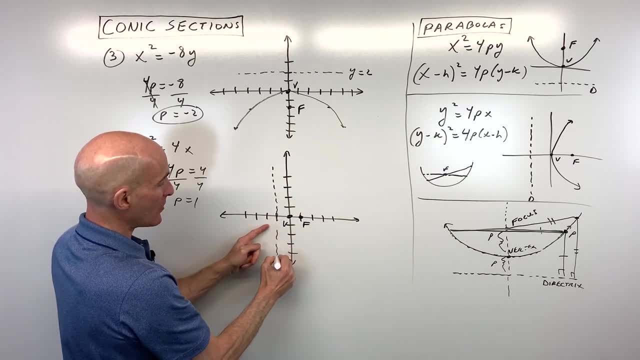 And if I go left 1, that's going to be our directrix, which in this case is x equals negative 1. Okay, vertical lines are x equals lines. So now we know the parabola is going to look something like that. 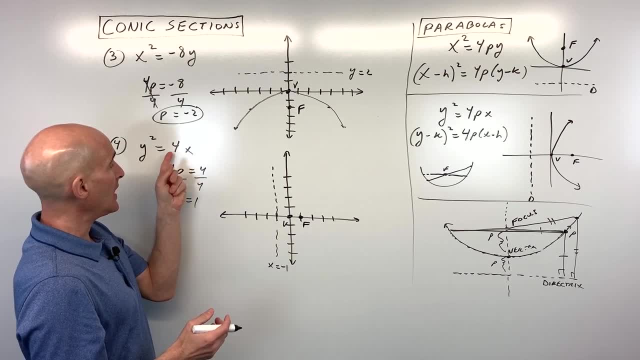 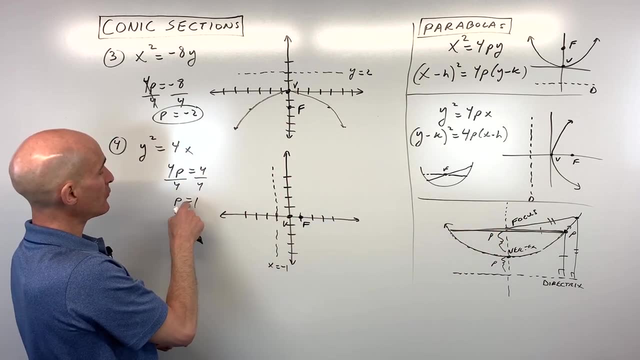 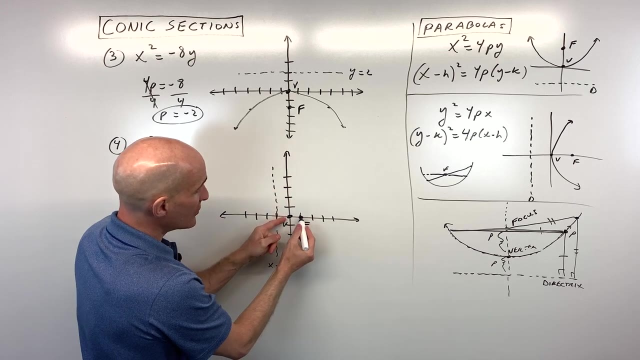 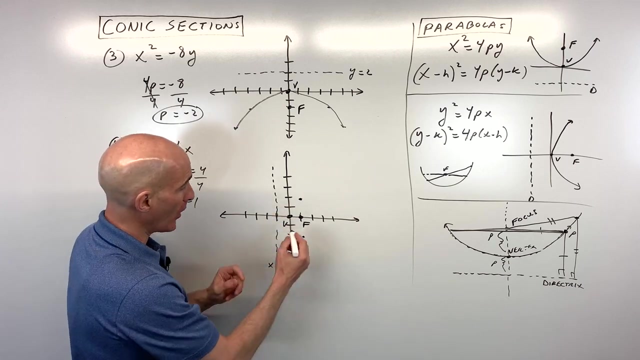 The only other thing is to get a few more points. And if we remember again that this focal chord, this special focal chord here, is going to be 4 times p. So p is 1, 4 times 1 is 4, or you can just look at this number here, 4. So at the level of the focus, it's going to be 4 units wide. If you cut that in half, that's going to be 2. So I'm going to go up 2 and I'm going to go down 2. That's going to give me a width of 4. Okay, so there's our parabola. Okay, see if we can do number 5 and 6. These ones are a little bit more challenging because of the transformations. 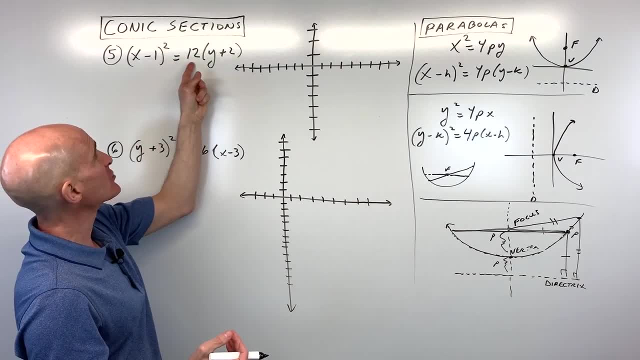 Let's start with number 5. We've got x minus 1 squared equals 12 times y plus 2. So what do you think for this one? Where is the vertex? 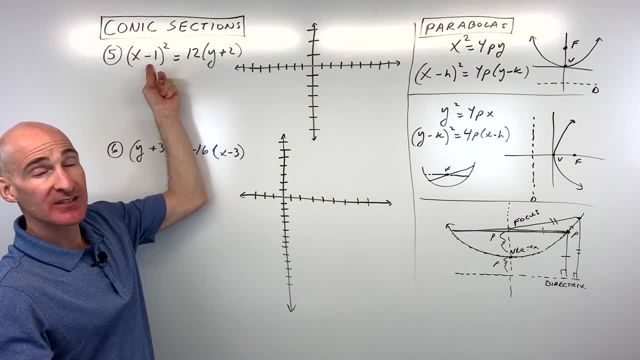 Well, an easy way to remember it is the one that's grouped with the x. It's going to be the x. It's going to be the y-coordinate of the vertex. The one that's grouped with the y is going to be the y-coordinate of the vertex. 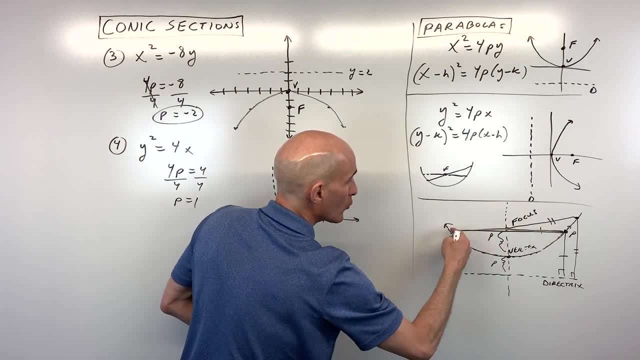 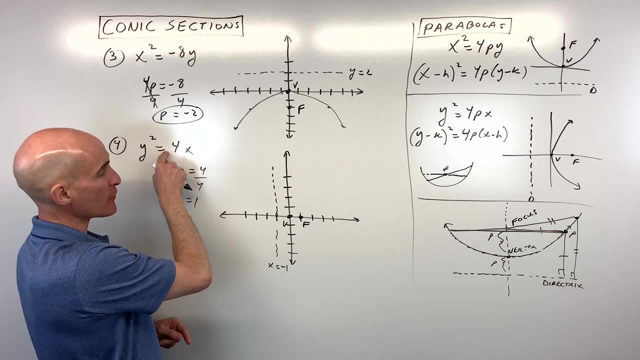 And if we remember again that this focal chord, the special focal chord here, is gonna be four times P, So P is one. four times one is four, or you can just look at this number here: four. So at the level of the focus. 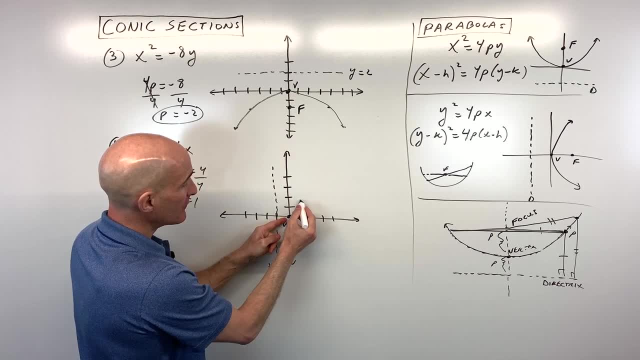 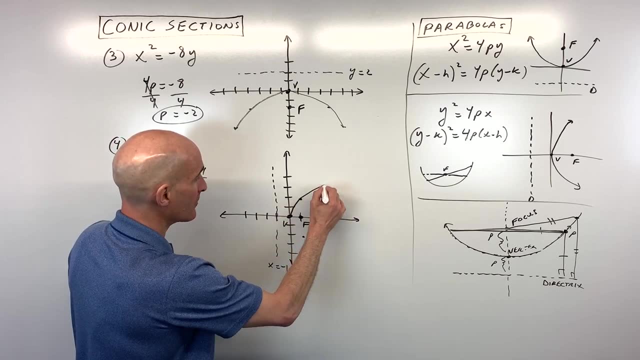 it's gonna be four units wide. If you cut that in half, that's gonna be two. So I'm gonna go up two and I'm gonna go down two. That's gonna give me a width of four. okay, So there's our parabola. 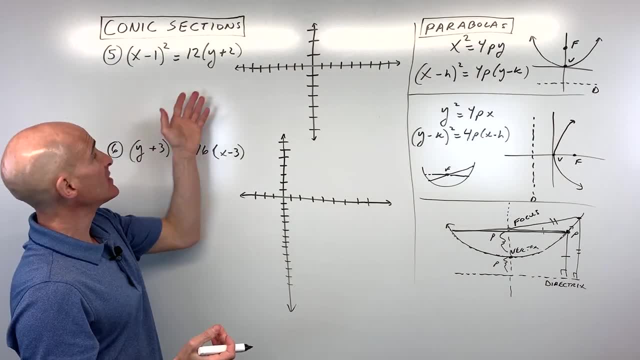 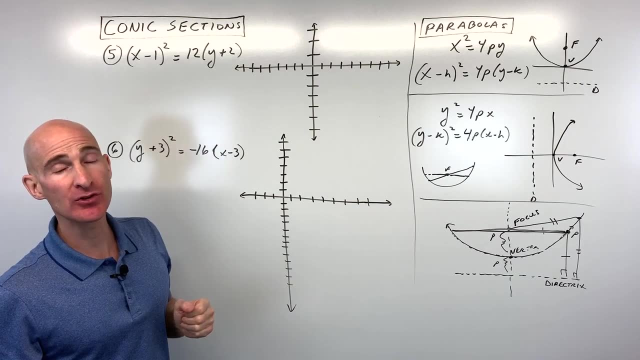 Okay, see if you can do number five and six. These ones are a little bit more challenging because of the transformations. Let's start with number five. We've got X minus one. squared equals 12 times Y plus two. So what do you think for this one? 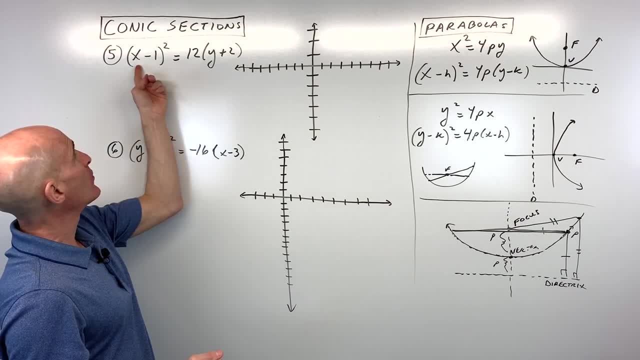 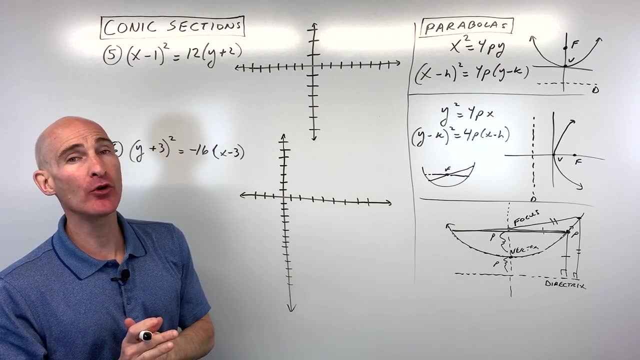 Where is the vertex? Well, easy way to remember it is: the one that's grouped with the X is gonna be the X coordinate of the vertex. The one that's grouped with the Y is gonna be the Y coordinate of the vertex. The only thing you wanna remember, though. 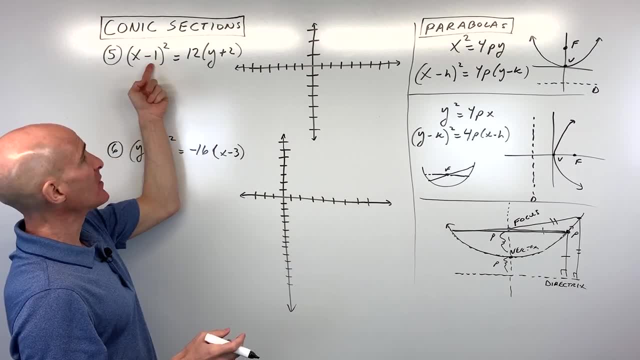 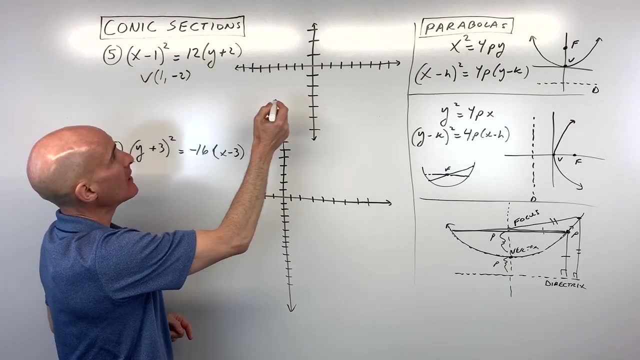 is that it's the opposite sign, right. So here, at X minus one, this is actually gonna be a vertex of positive one. Y plus two. that's gonna be negative two. So your vertex here is gonna be at one comma: negative two. 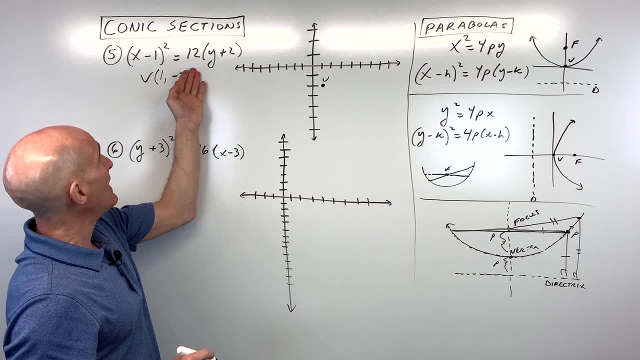 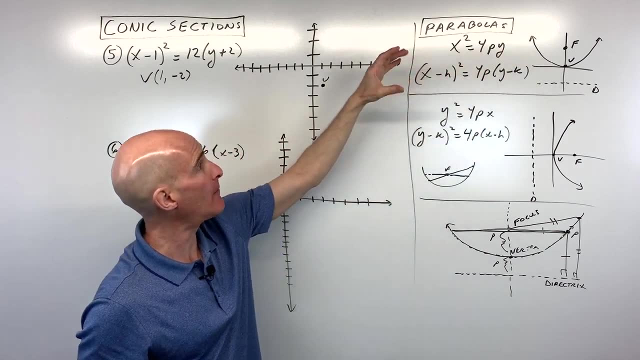 right there. Sometimes I like to put a V for vertex. And then now the question is: does it open up, down, left or right? Well, see how this is X squared. So we know that's this type here. When X is squared, it opens up or down. 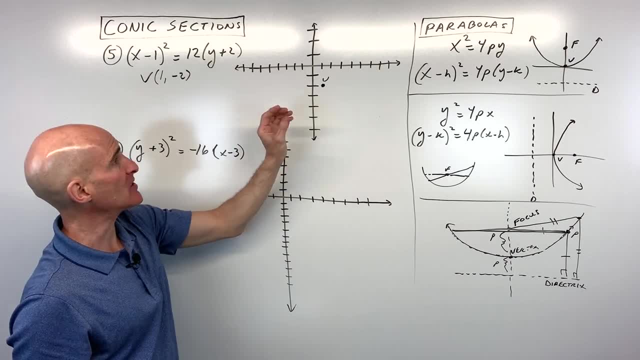 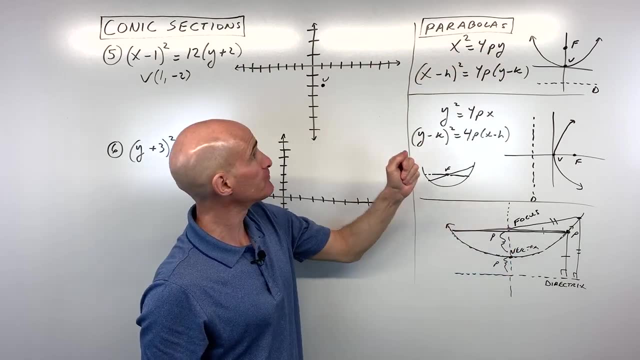 But because this coefficient is positive, it's gonna be opening up. Okay, so now we know the parabola is gonna look something like that. The next thing we wanna do is we wanna find that P value. That's like the distance from the vertex to the focus. 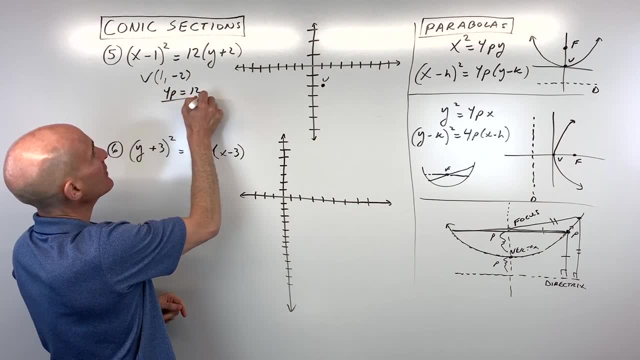 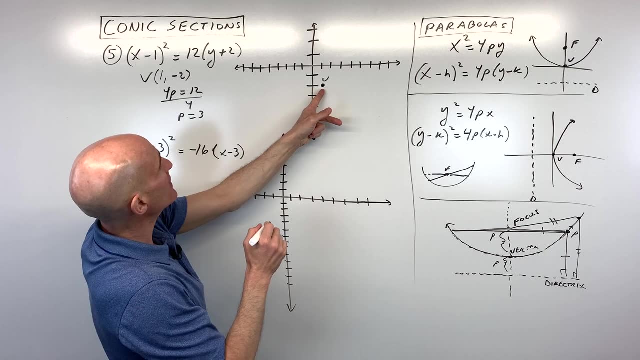 And you're gonna say: well, four P is equal to 12. divide by four and you can see that P is equal to three. So, from this point, since we know that the parabola is opening up, we're gonna go up three units. 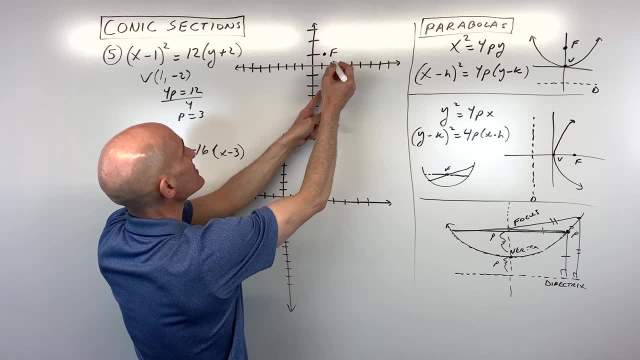 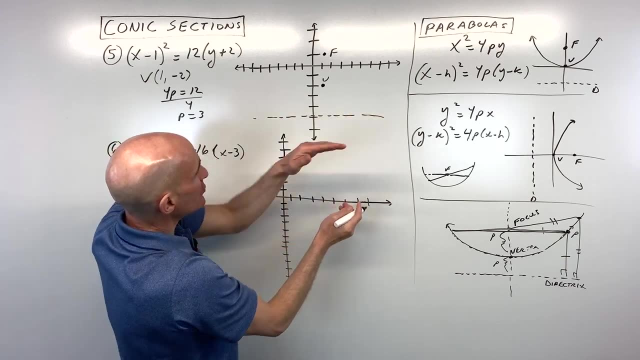 One, two, three. There's our focus. I'll just label it F, And you also wanna go down three. One, two, three. This is where our directrix is. You can kind of think of the directrix as like a deflector. 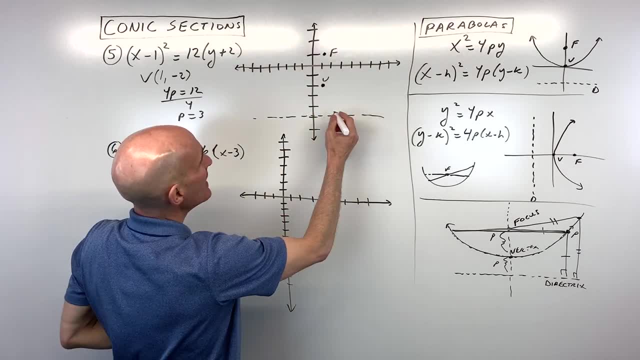 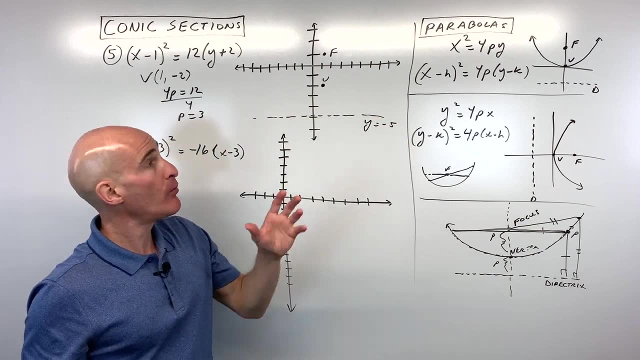 like it's opening away from the directrix towards the focus. And this line is one, two, three, four, five, That's Y equals negative five horizontal line. And then we just wanna get a couple more points here And we can use that technique of C4P. 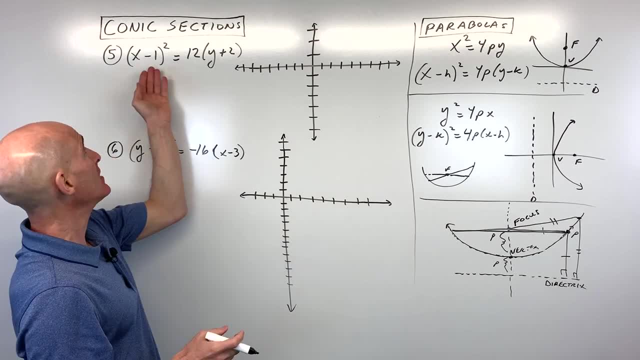 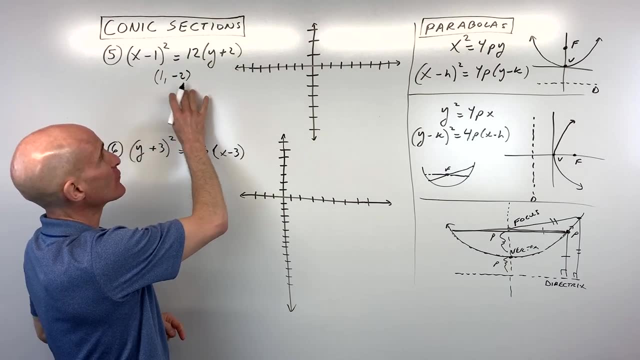 The only thing you want to remember, though, is that it's the opposite sign, right? So here, x minus 1, this is actually going to be a vertex of positive 1. y plus 2, that's going to be negative 2. So your vertex here is going to be at 1 comma negative 2, right there. Sometimes I like to put a v for vertex. 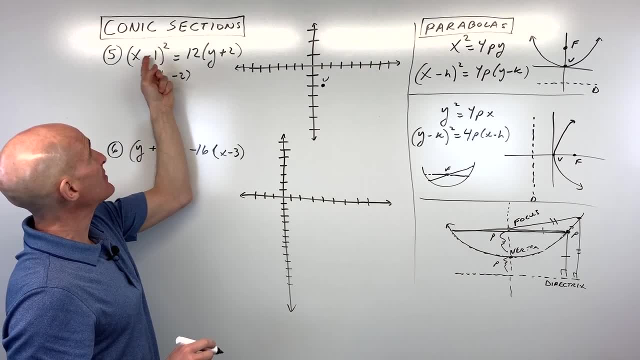 And then now the question is, does it open up, down, left, or right? Well, see how this is x squared? So we know that's this type here. When x is squared, it opens up or down. 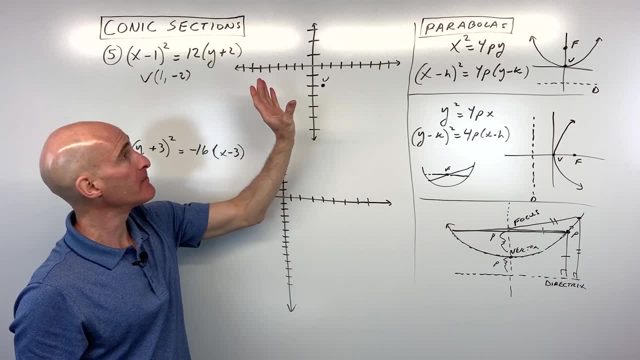 But because this coefficient is positive, it's going to be opening up. Okay, so now we know the parabola is going to look something like that. 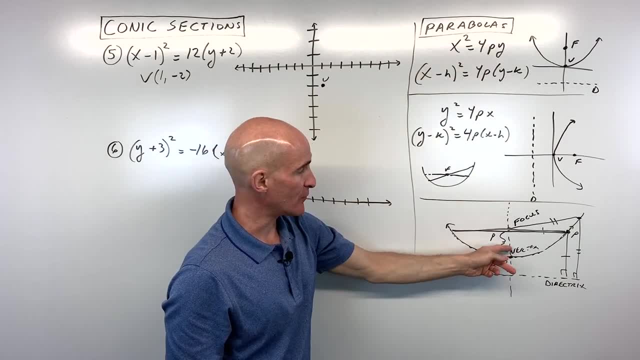 The next thing we want to do is we want to find that p-value. That's like the distance from the vertex to the focus. 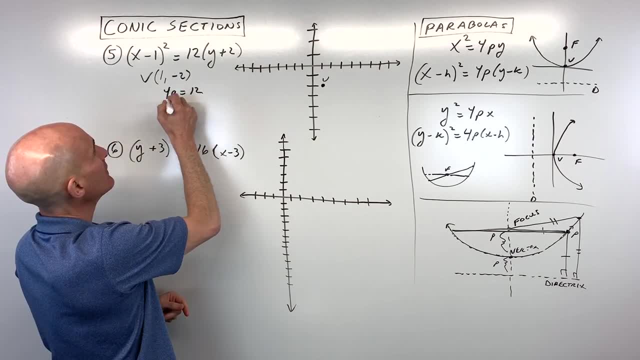 And you're going to say, well, 4p is equal to 12. Divide by 4, and you can see that p is equal to 3. 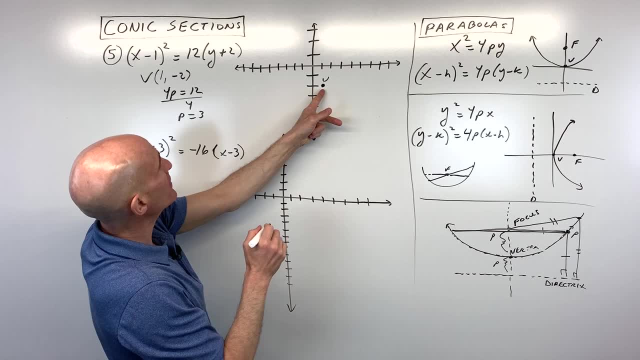 So from this point, since we know that the parabola is opening up, we're going to go up 3 units. 1, 2, 3. There's our focus. I'll just label it f. And you also want to go down 3. 1, 2, 3. 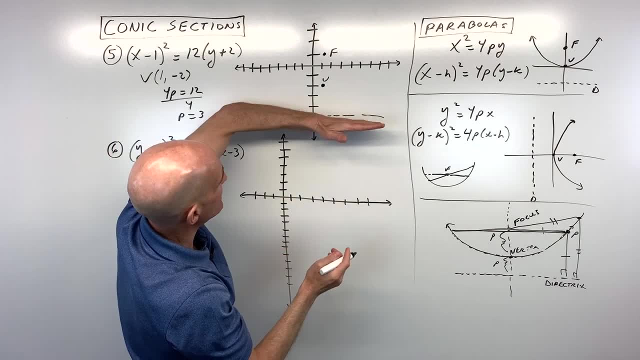 This is where our directrix is. You can kind of think of the directrix as like a deflector, 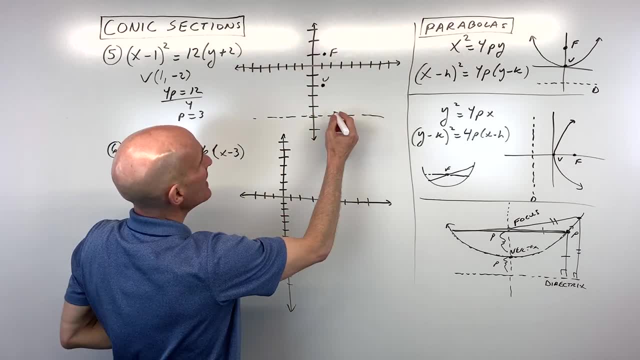 like it's opening away from the directrix towards the focus. And this line is 1, 2, 3, 4, 5. That's y equals negative 5, horizontal line. 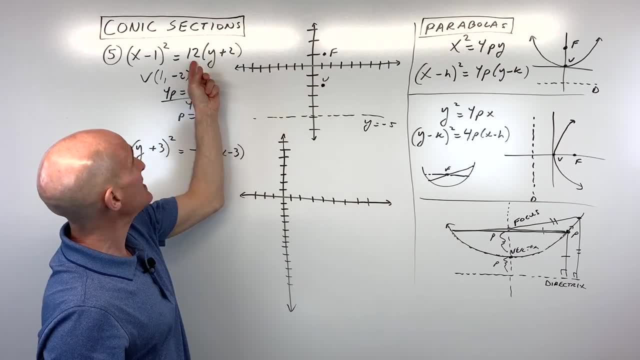 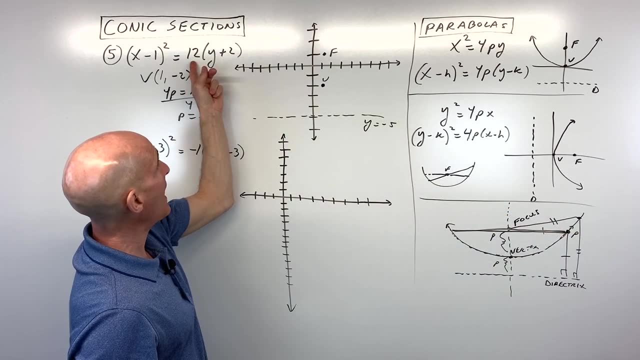 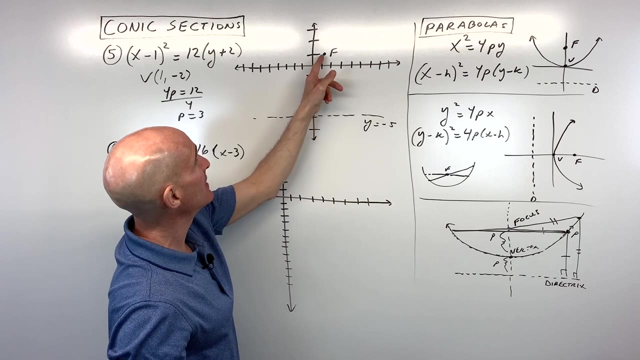 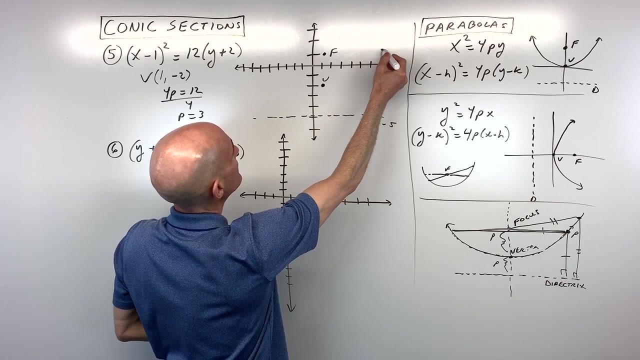 And then we just want to get a couple more points here. And we can use that technique of see 4p is this special focal cord we talked about. And so it's 12 wide at the level of the focus. Okay, not the vertex, but the focus. Of course, the parabola keeps getting wider and wider as it goes up. But at this level here, it's going to be 12 wide. So we're going to go half on each side. We're going to go right 6, 1, 2, 3, 4, 5, 6. And left 6, 1, 2, 3, 4, 5, 6. 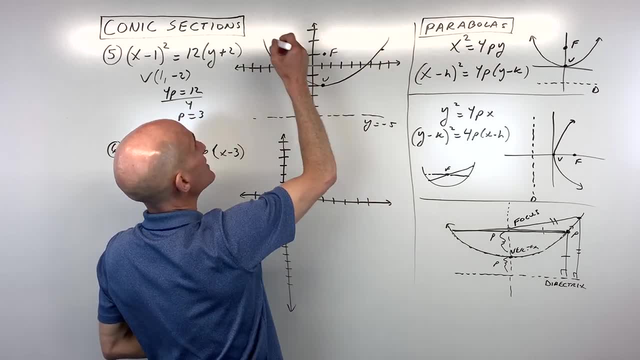 And we're just going to, you know, this is just a sketch. You could find more points if you want to be a little bit more precise, but that gives you a pretty good idea. 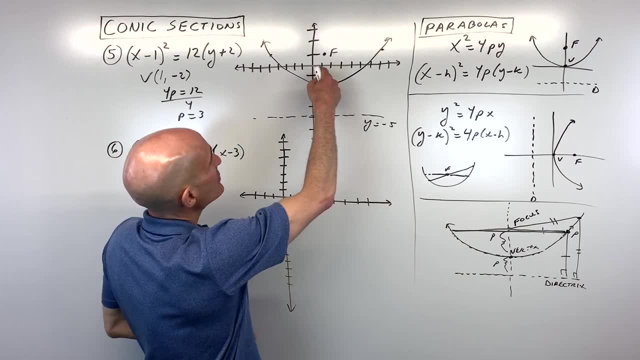 Now, sometimes I'll ask you for the equation of the axis of symmetry. And you can see here this is going to be x equals 1. Okay, so that's the... 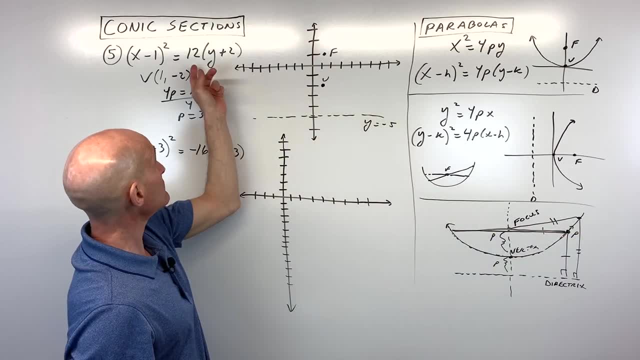 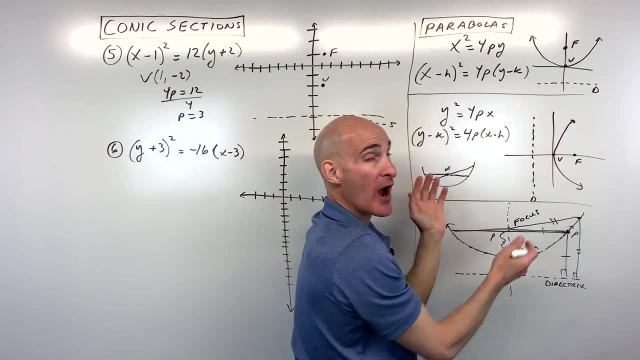 is this special focal core we talked about, And so it's 12 wide At the level of the focus. Okay, not the vertex but the focus. Of course, the parabola keeps getting wider and wider as it goes up. 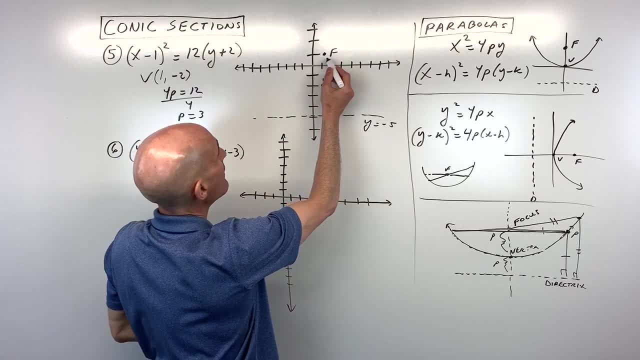 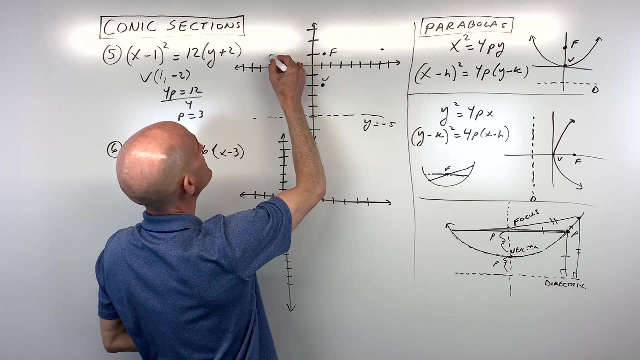 But at this level here it's gonna be 12 wide, So we're gonna go half on each side. We're gonna go right six, one, two, three, four, five, six And left: six one, two, three, four, five, six. 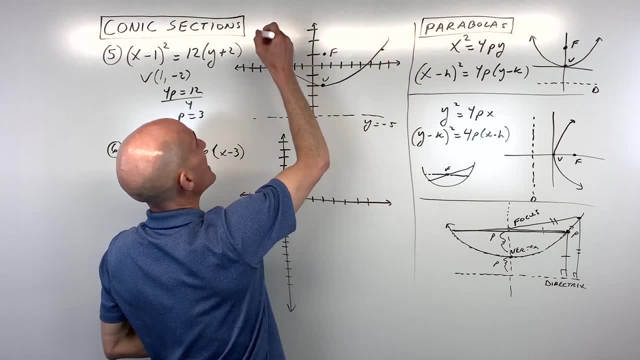 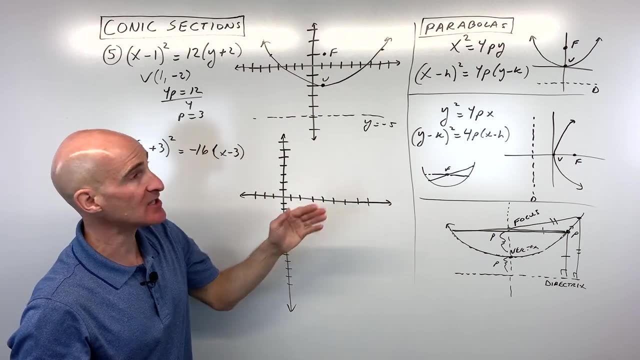 And we're just gonna. you know this is just a sketch. You could find more points if you wanna be a little bit more precise, but that gives you a pretty good idea Now. sometimes they'll ask you for the equation of the axis of symmetry. 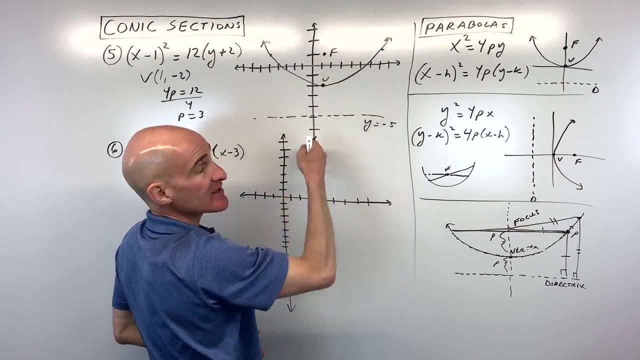 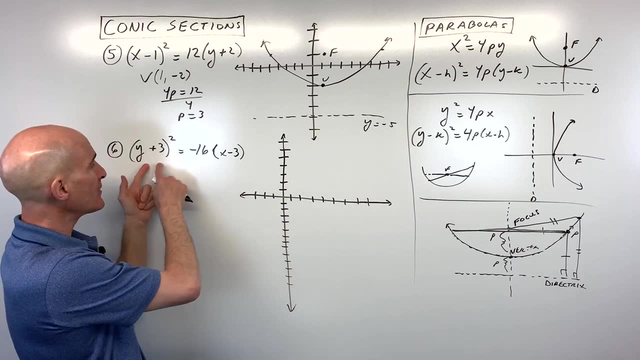 And you can see here this is gonna be: X equals one. Okay, so that's the vertical line here. If you fold it over, it matches to itself. Let's try number six. See if you can do this one. So what do you think for this one? 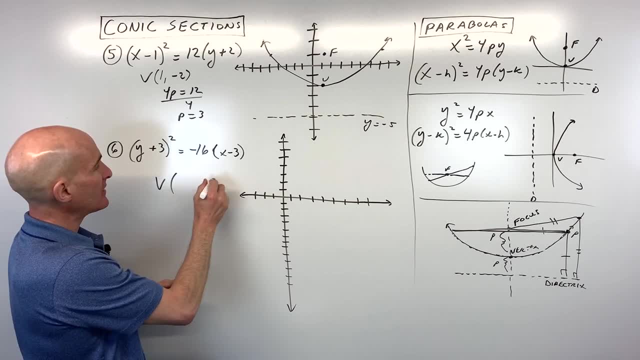 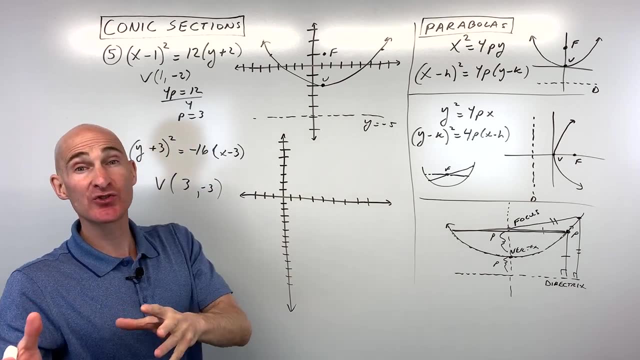 First step: what's the vertex? Well, it looks like if you said the vertex is three comma, negative three. Now, sometimes the mistakes that students make is they'll say: well, wait a second, Mario, isn't it? negative three, positive three. 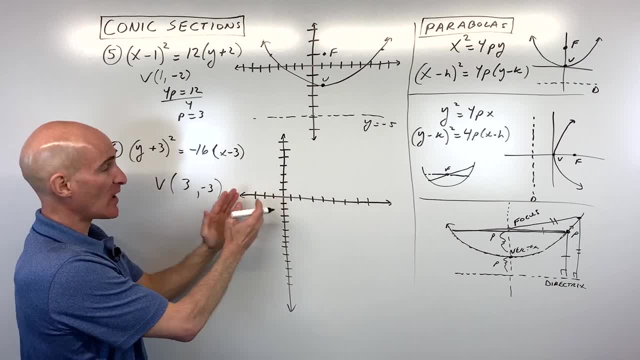 And that's because we're used to thinking of like reading, like left to right, like X, Y, Z, right, like that. But you wanna remember, the one group with the X is the X, the one group with the Y is the Y. 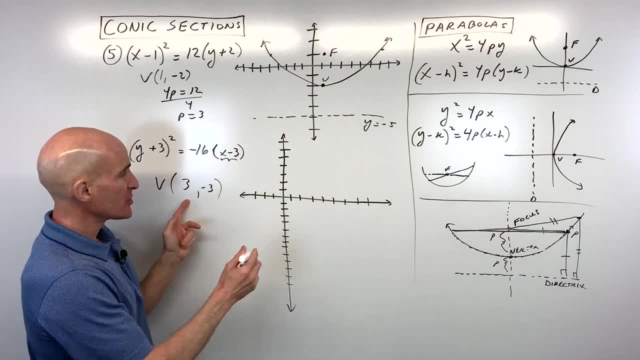 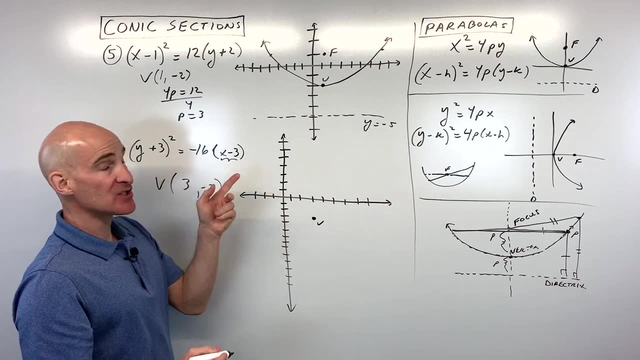 It's just that it's the opposite side from what you see here. So let's go ahead and plot that vertex, three negative three, which is gonna put you right there. V for vertex. And now the next question is: is it opening up down left or right? 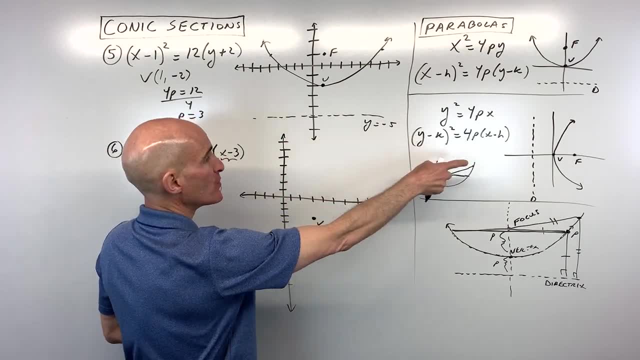 Well, you can see that it's a Y squared type. That's this type here, So it opens right or left, but because this is negative, it's gonna open to the left. So we know that it's gonna look something like this: 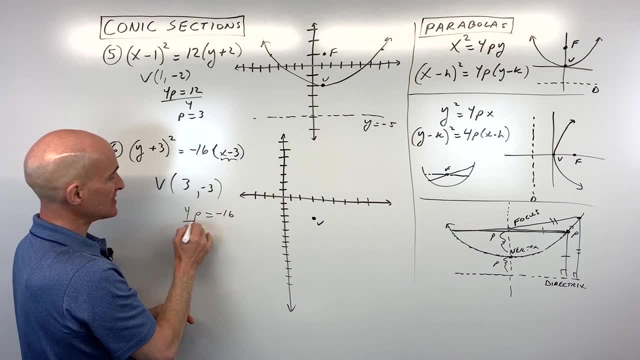 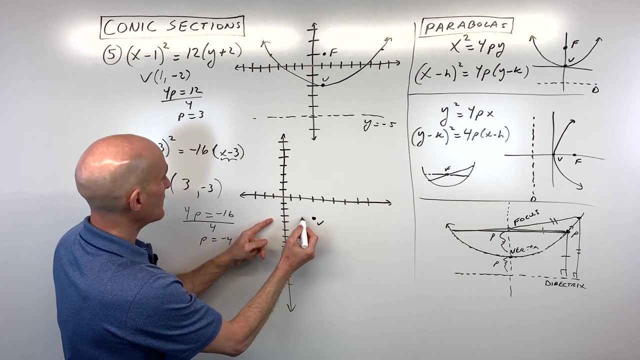 We're gonna find out what P is by setting four P equal to negative 16, divide by four, So you can see P is negative four. So from the vertex I'm gonna go, let's see: left, four, one, two, three, four, right there. 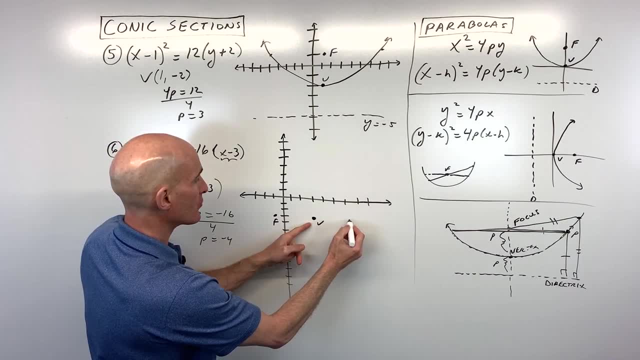 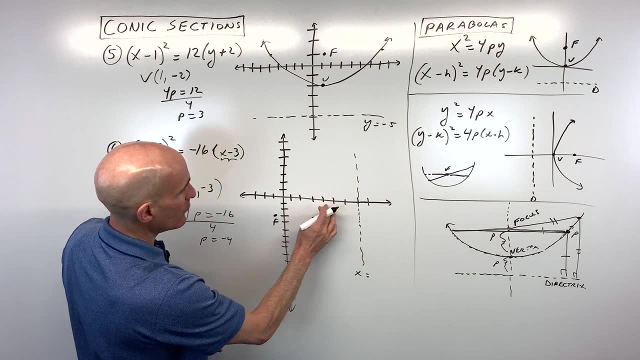 So that's gonna be our focus, And if we go the other direction, one, two, three, four- this is our directrix and that's the line X equals. let's see: one, two, three, four, five, six, seven, Vertical line here, if you fold it over, it matches to itself. Let's try number 6. See if you can do this one. So what do you think for this one? First step, what's the vertex? 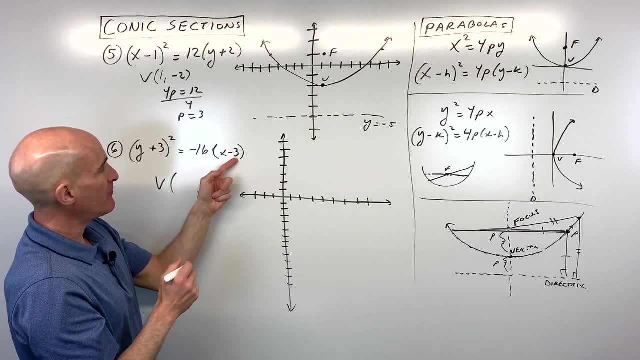 Well, it looks like if you said the vertex is 3, negative 3. 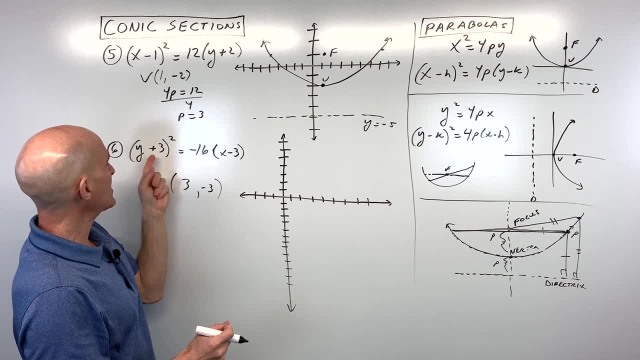 Now, sometimes the mistakes that students make is they'll say, well, wait a second, Mario, isn't it negative 3, positive 3? 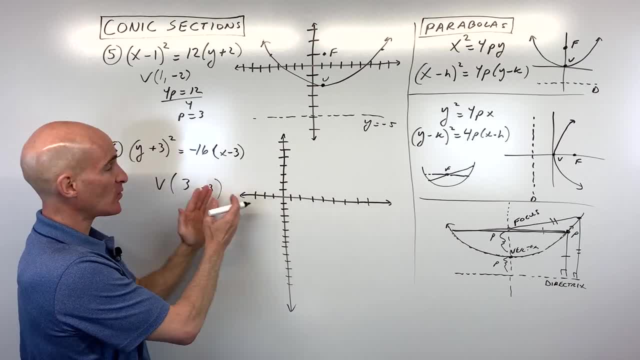 And that's because we're used to thinking of like reading like left to right, like x, y, z, right, like that. But you want to remember the one group with the x is the x. The one group... 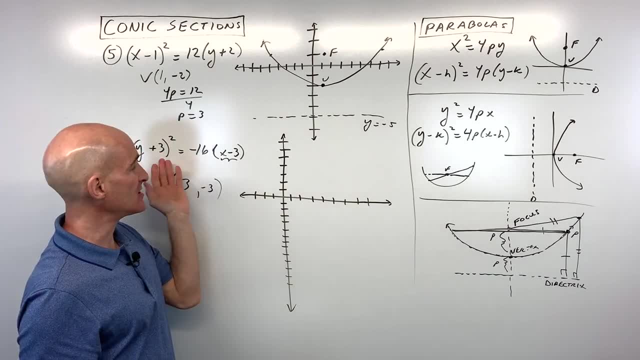 The one group with the y is the y. It's just that it's the opposite side from what you see here. 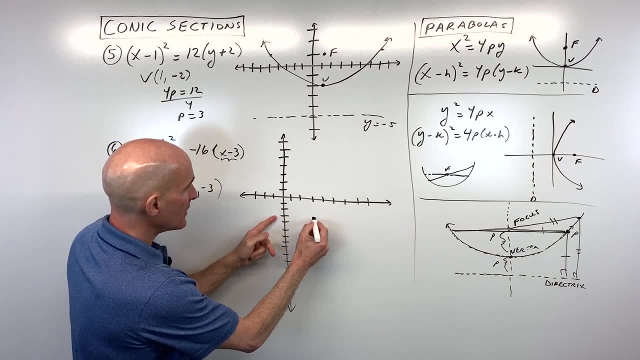 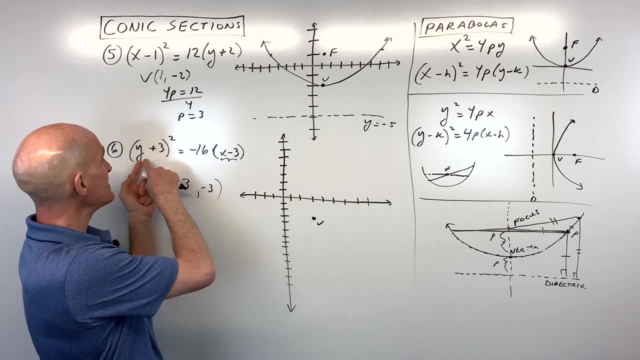 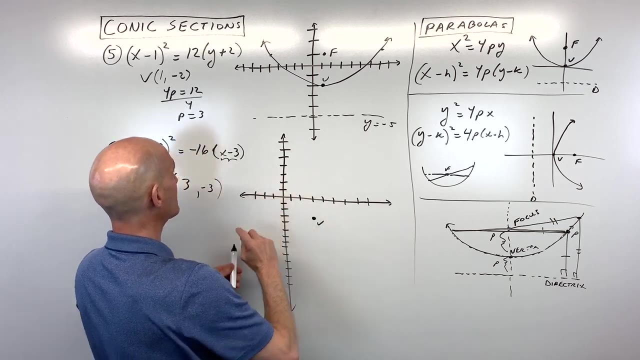 So let's go ahead and plot that vertex. 3, negative 3, which is going to put you right there, v for vertex. And now the next question is, is it opening up, down, left, or right? Well, you can see that it's a y squared type. That's this type here. So it opens right or left. But because this is negative, it's going to open to the left. 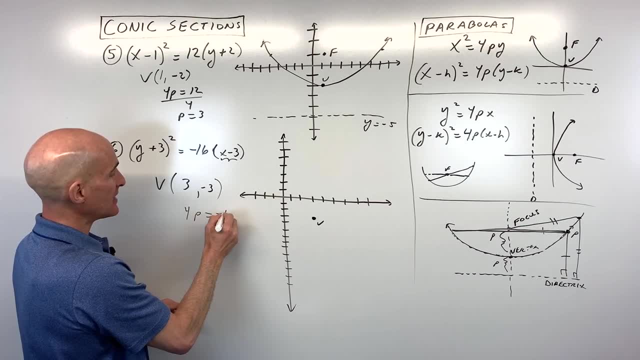 So we know that it's going to look something like this. We're going to find out what p is by setting 4p equal to negative 16, divide by 4. So you can see p is negative 4. 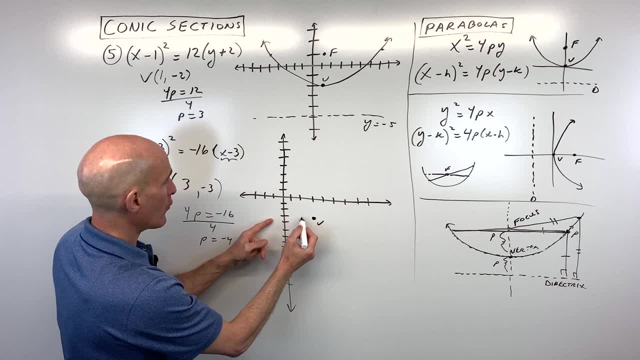 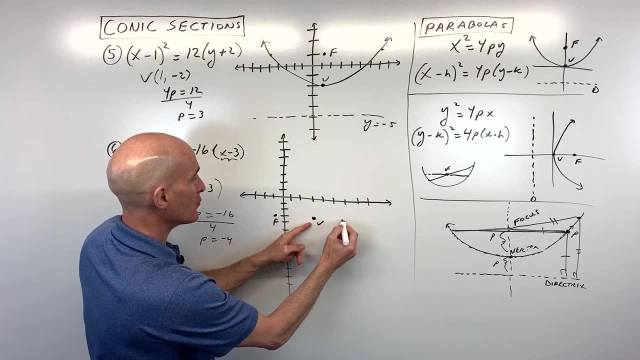 So from the vertex, I'm going to go, let's see, left 4. 1, 2, 3, 4, right there. So that's going to be our focus. And if we go the other direction, 1, 2, 3, 4, this is our directrix. 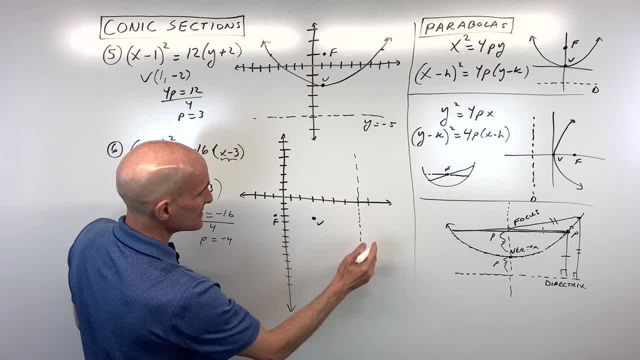 And that's the line x equals, let's see, 1, 2, 3, 4, 5, 6, 7. Okay. 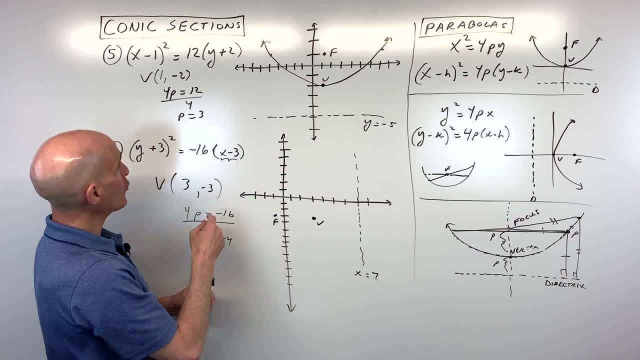 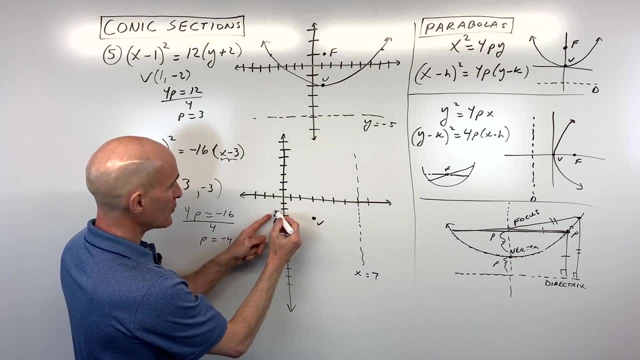 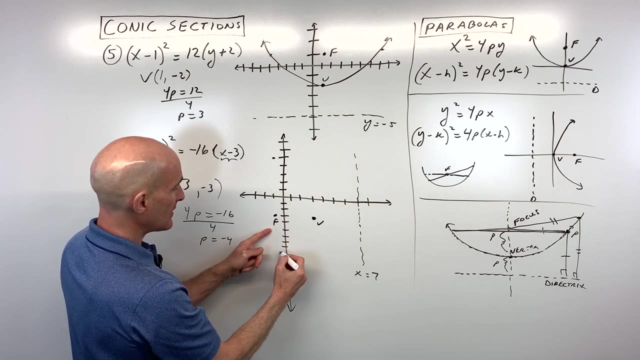 Now we just want to get a couple more points. And remember that focal chord is going to be 16 units wide at the level of the focus. So if I cut 16 and a half, that's 8. So I'm going to go from the focus. I'm going to go up 8 and down 8. 1, 2, 3, 4, 5, 6, 7, 8. And down 8. 1, 2, 3, 4, 5, 6, 7, 8. 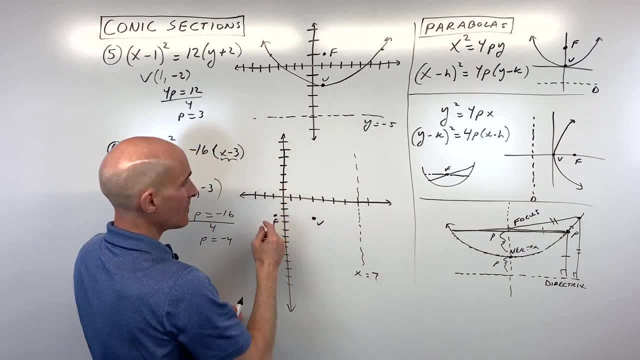 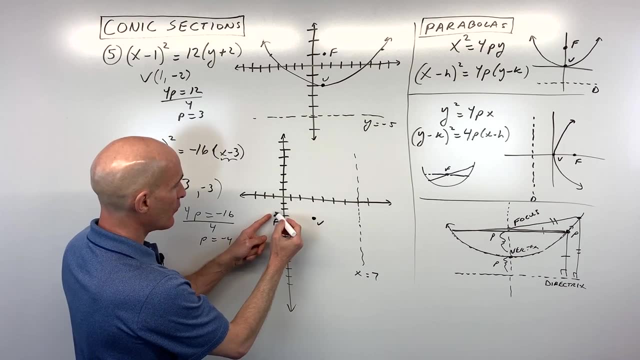 Okay, now we just wanna get a couple more points. And remember that focal chord is gonna be 16 units wide at the level of the focus. So if I cut 16 and a half that's eight. So I'm gonna go from the focus. 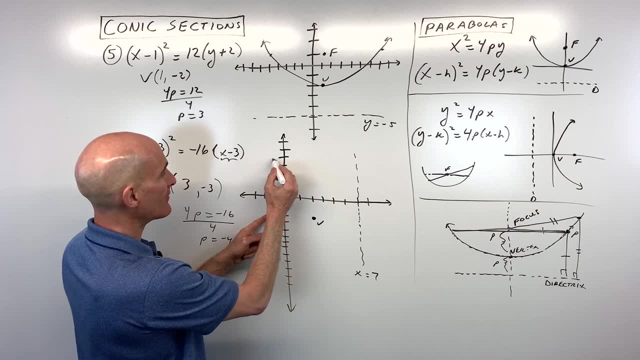 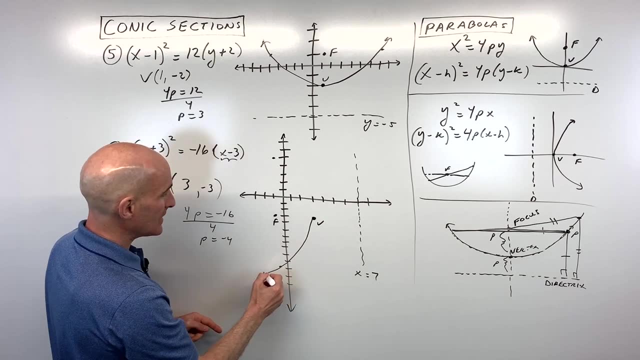 I'm gonna go up eight and down eight. one, two, three, four, five, six, seven, eight and down eight. one, two, three, four, five, six, seven, eight, and that just kind of gives you an idea. 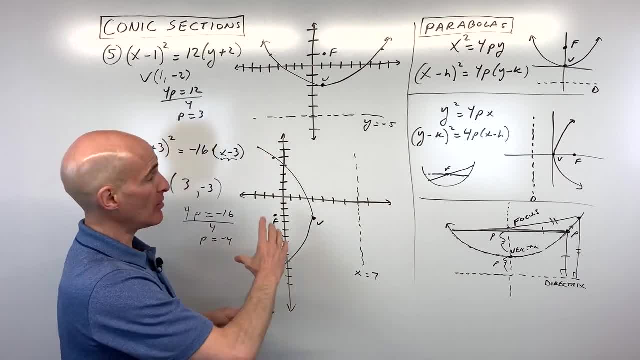 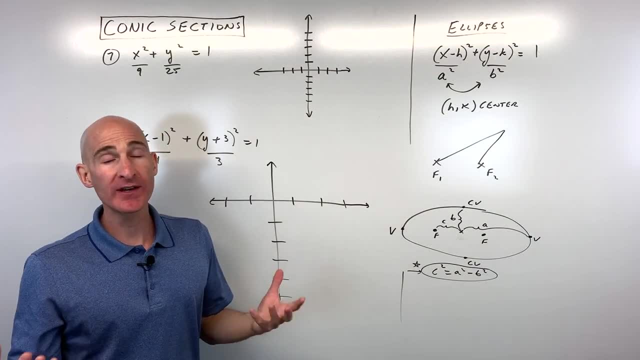 about how wide the parabola is. It could be narrow, it could be wide. So you've got a couple more points and you can plot more than that if you want. Now we're gonna start talking about ellipses. So what exactly is an ellipse? 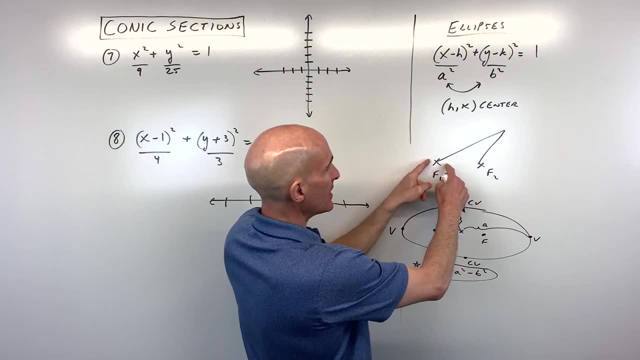 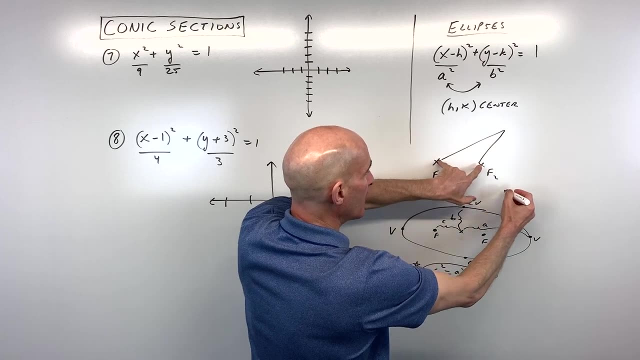 Well, an ellipse is. imagine this: if you were to take a piece of string right and you were to hold down the two ends of the string like that and you put your pencil here and you pull it, what it does is it traces out like an oval. 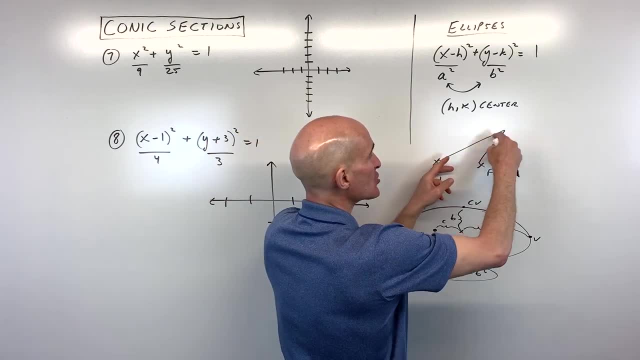 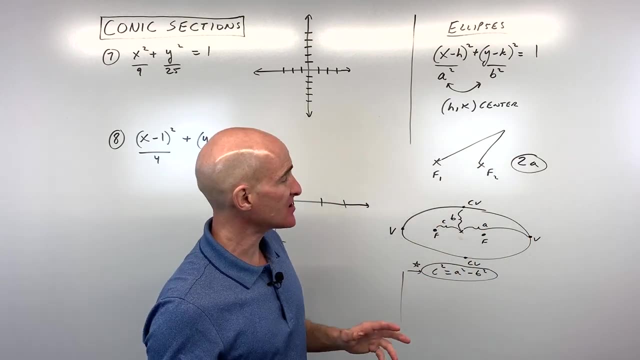 we call it an ellipse, okay. And what's interesting is this string: it doesn't stretch, it's always a fixed length, and that fixed length we call that length 2a, And you'll see why in just a second. 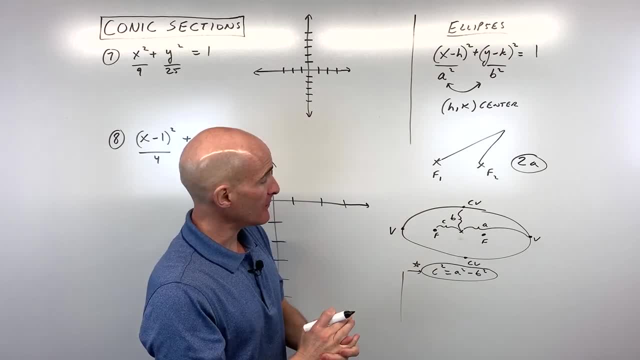 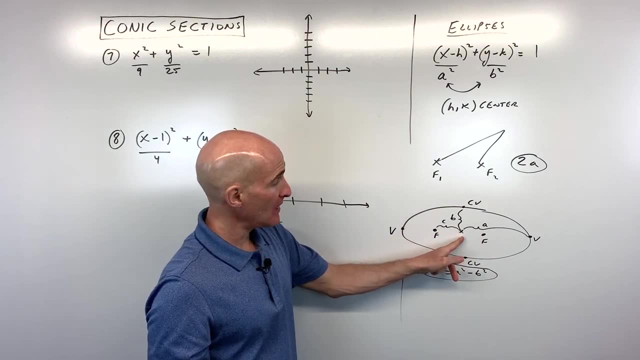 So some main important components of an ellipse are gonna be the two foci, okay, f1 and f2.. Halfway in between those foci is your center point And then these points here along this longer see how the ellipse is a little bit more elongated. 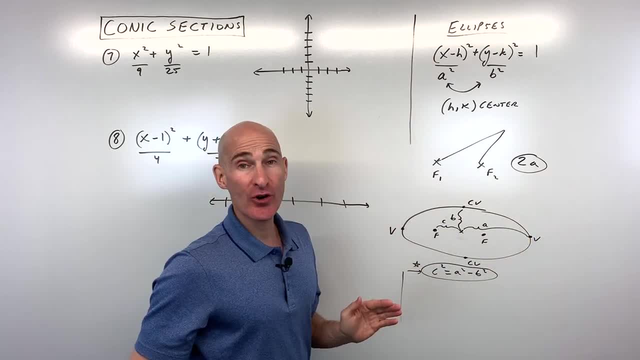 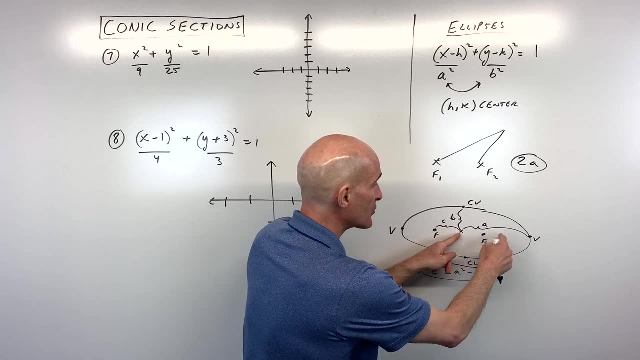 into one direction. Well, this length, here we call the major axis, okay, the longer axis, This one, here we call the minor axis, okay, it's a little bit narrower. And the distance from the center to the vertex, either vertex, the vertices, that distance we call a. 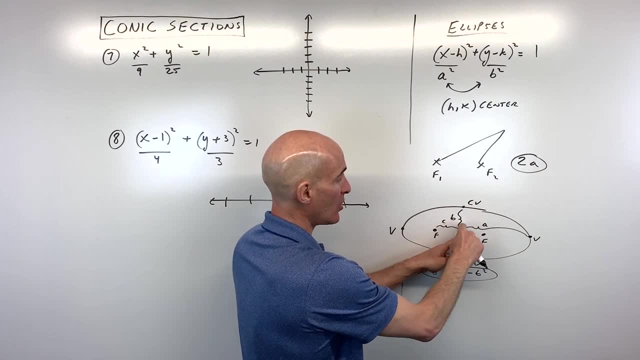 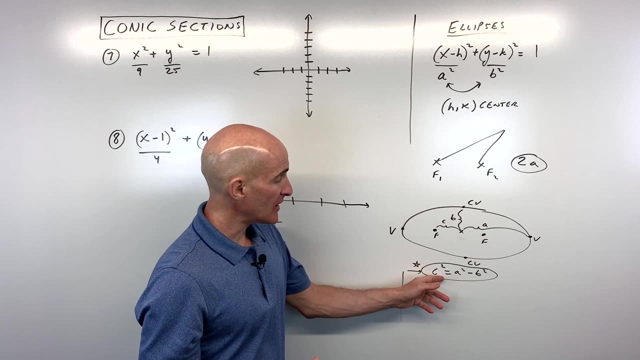 The distance from the center to the co-vertex, or minor vertex, we call that distance b, And the distance from the center to the, either the foci, we call that c, And all those values are related through this equation here. 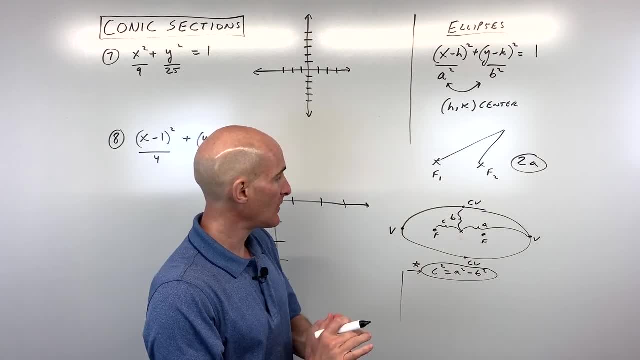 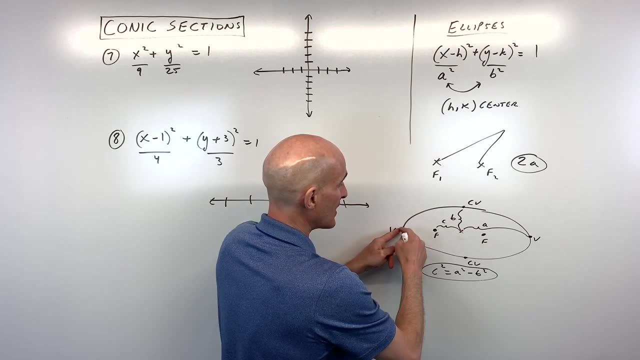 c squared equals a squared minus b squared. So you might wanna write that down and memorize that. But basically this distance here see how this is a and from here to here that's a, so that major axis is a length of 2a. 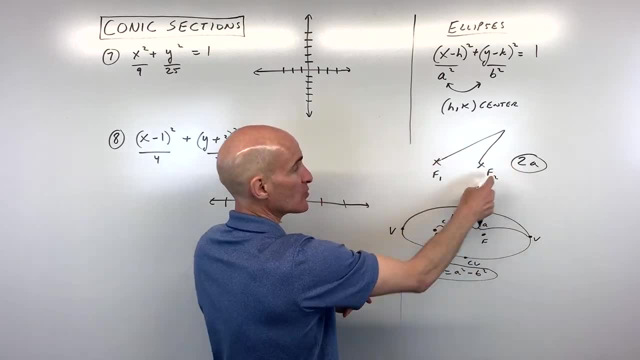 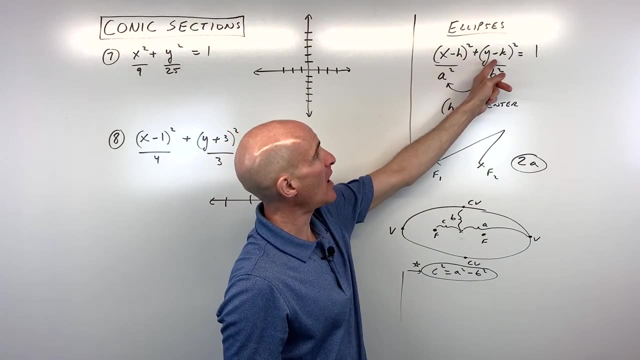 which is the same length as this string here, okay, which we've said, that's our focal length: 2a. Now the standard form of the equation of ellipse is this one here: y minus h squared, plus y minus k squared, okay. 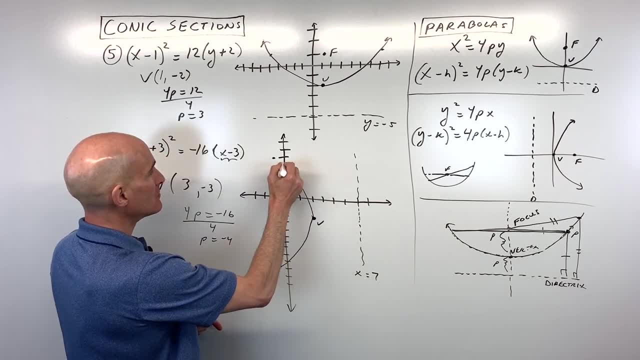 And that just kind of gives you an idea about, you know, how wide the parabola is. It could be narrow. It could be wide. So you've got a couple more points. 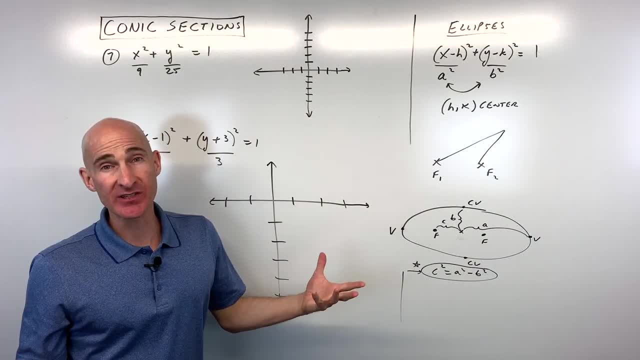 And you can plot more than that if you want. Now we're going to start talking about ellipses. 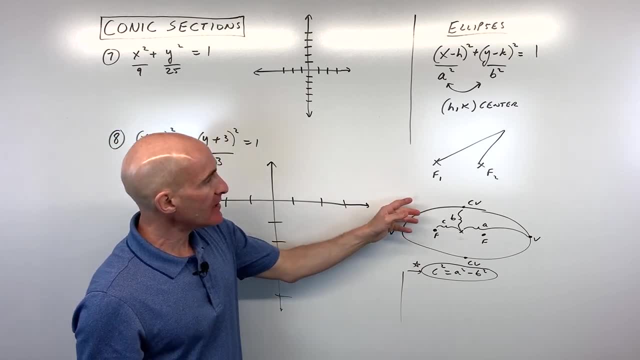 So what exactly is an ellipse? Well, an ellipse is, imagine this. If you were to take a piece of string, right? And you were to hold down the two ends of the string like that. 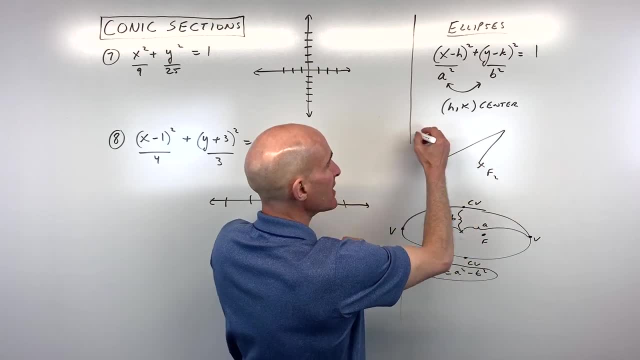 And you put your pencil here and you pull it. What it does is it traces out like an oval. We call it an ellipse. Okay. 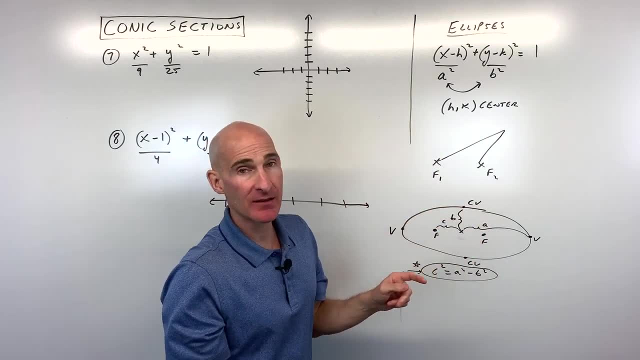 And what's interesting is this string, it doesn't stretch. It's always a fixed length. And that fixed length, we call that length 2A. And you'll see why in just a second. 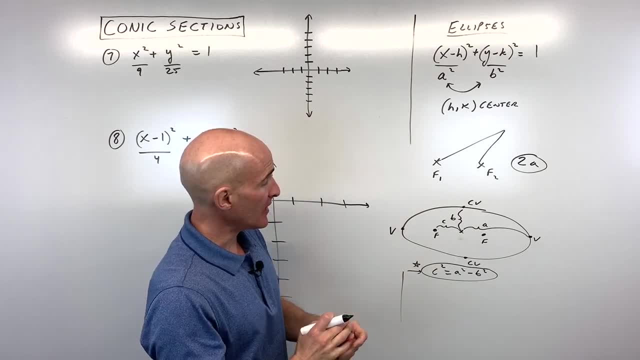 So some main important components of an ellipse are going to be the two foci. Okay. F1 and F2. Halfway in between. 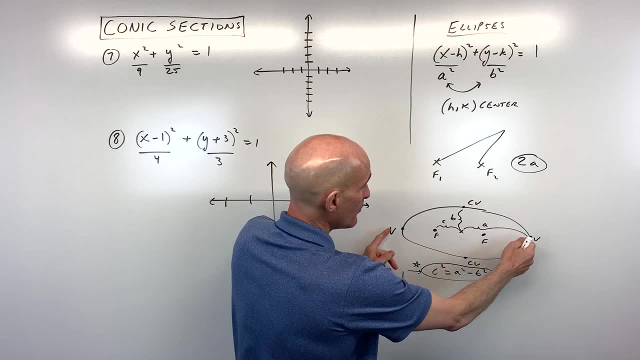 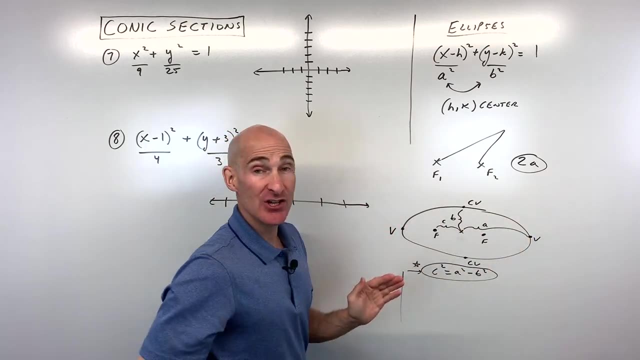 And the half way in between those foci is your center point. And then these points here along this longer, see how the ellipse is a little bit more elongated in one direction? Well, this length here we call the major axis. Okay, the longer axis. This one here we call the minor axis. Okay, it's a little bit narrower. 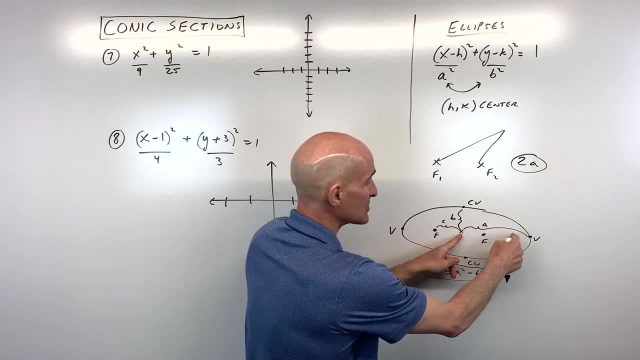 And the distance from the center to the vertex, either vertex, the vertices, that distance we call A. 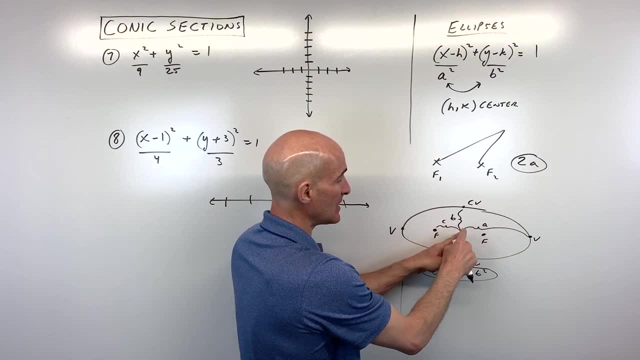 The distance from the center to the co-vertex, or minor vertex, we call that distance B. And the distance from the center to the, we call that C. 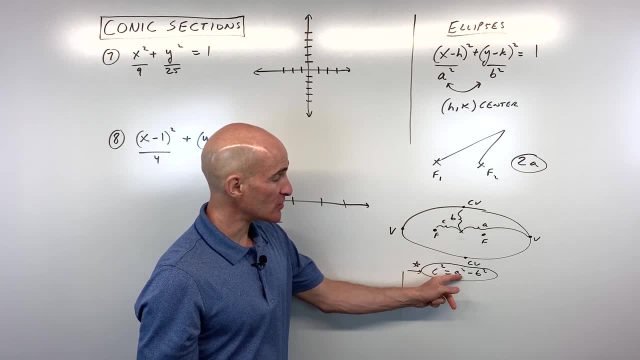 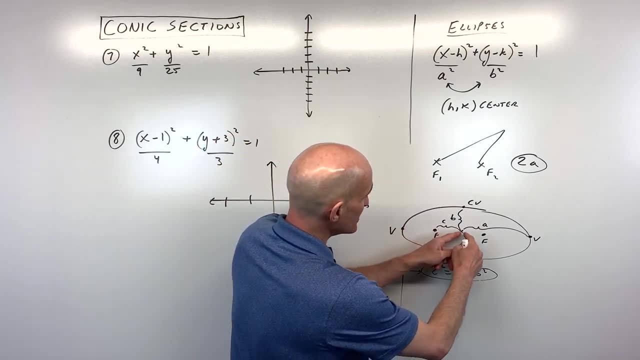 And all those values are related through this equation here. C squared equals A squared minus B squared. So you might want to write that down and memorize that. But basically, this distance here, see how this is A? And from here to here, that's A. 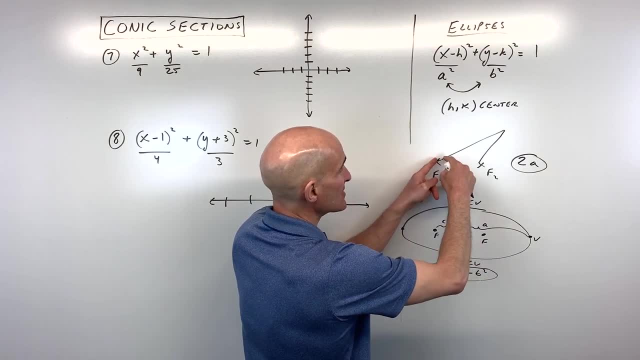 So that major axis is a length of 2A, which is the same length as this string here. Okay. Which we said that's our focal length 2A. 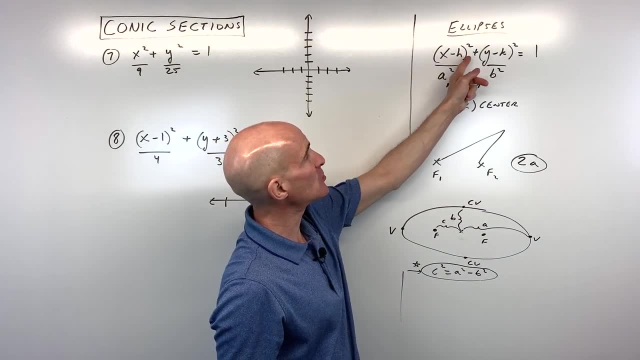 Now, the standard form of the equation of ellipse is this one here. It's X minus H squared plus Y minus K squared. Okay. Equals 1. And you see the denominator is A squared and B squared. 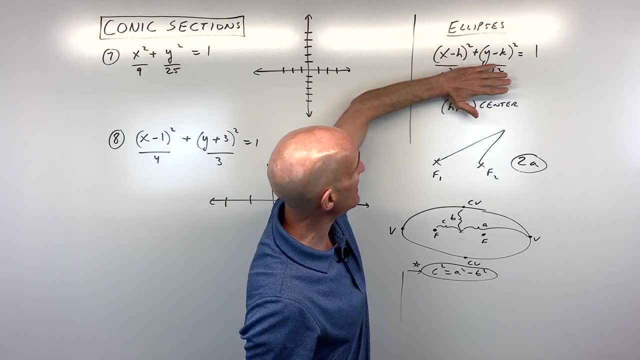 equals one and you see the denominator's: a squared and b squared. So if I was to cover up the a squared and b squared, it kinda looks like the equation of a circle, doesn't it? Now, with the a squared and b squared? 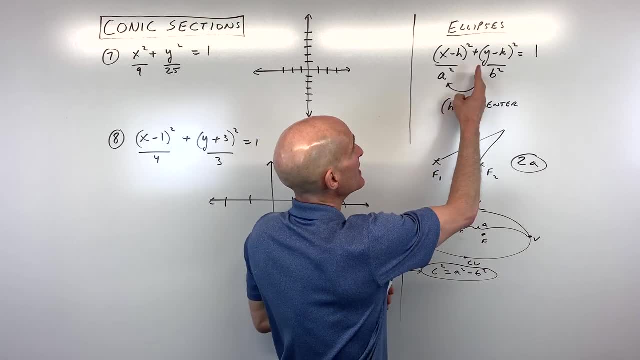 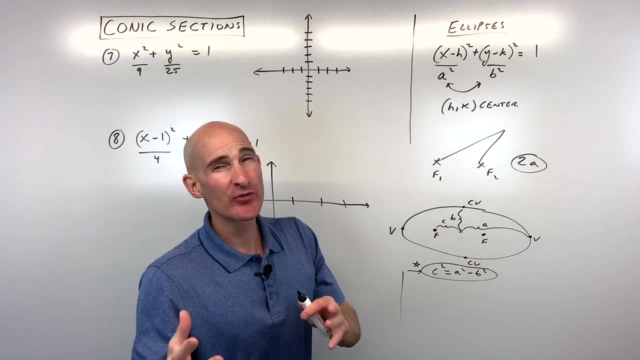 whichever denominator is larger. see, these ones can be interchanged, the denominators. Whichever denominator is larger, that's gonna be the a squared one. Whichever one's smaller, that's the b squared one. So let me show you, through some examples, how this works. 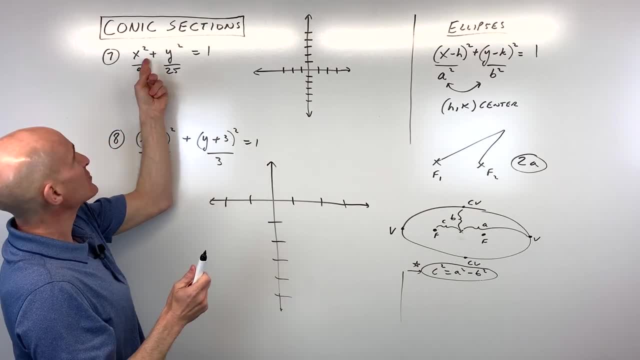 and I think it'll become a little bit clearer. So for number seven, what you'll notice is there's not an a-trig, there's not a k, So that means that the center of this ellipse is gonna be right at the origin. 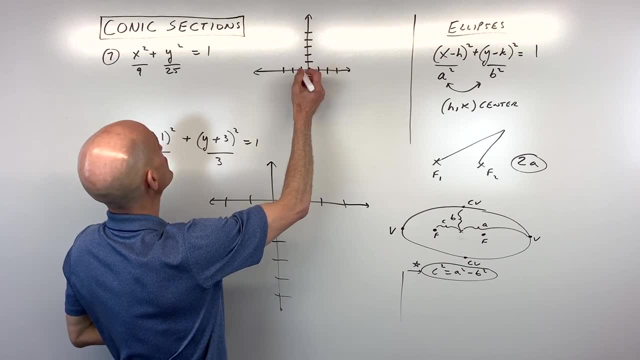 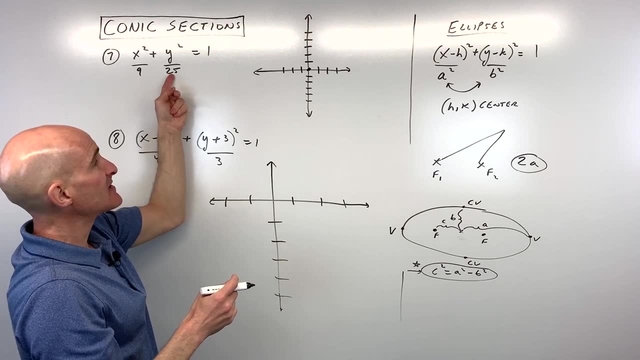 It hasn't shifted at all. So I'm just gonna put a point right here: at the origin: zero, zero. And now, when I look at the denominators, see how this denominator here, 25, is greater than nine. That means that this is gonna be our a squared right here. 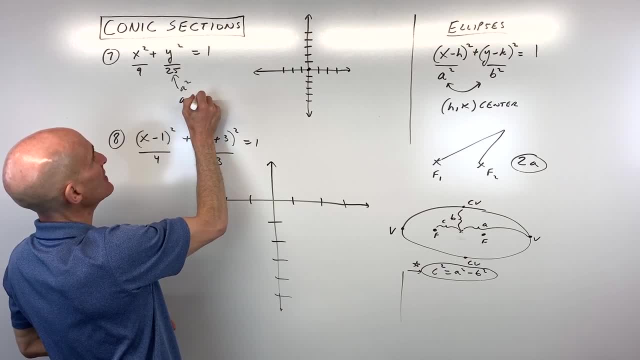 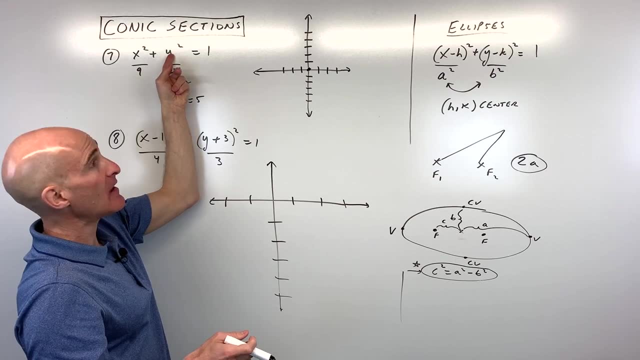 So if we take the square root of 25, that means that a is gonna be equal to five. And the other thing you wanna pay attention to is that see- whatever denominator see- this is underneath the y. that means you're gonna go in the y direction. 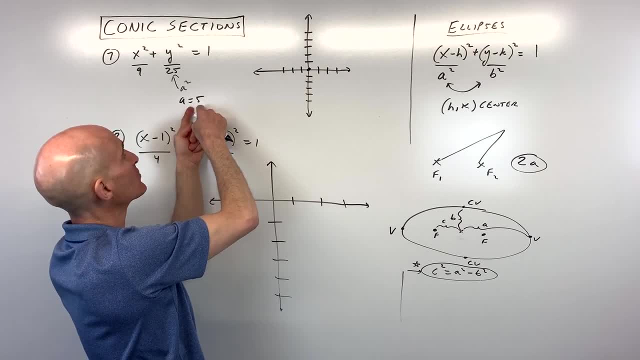 whereas this one's underneath the x. you're gonna go in the x direction, So in the y direction we're gonna be going five units: one, two, three, four, five in the y direction, up and down from the center. 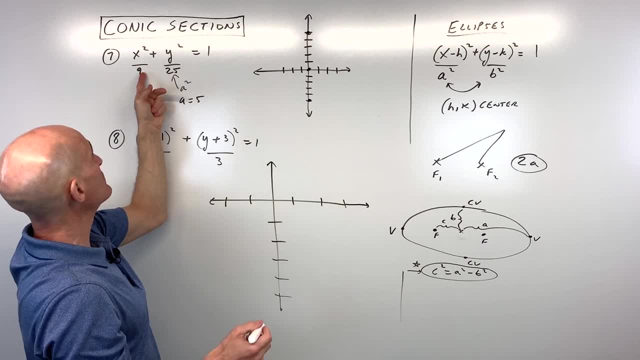 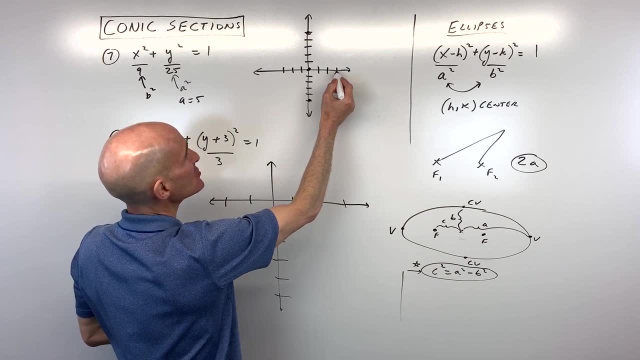 So that was our a distance. This one here is b squared because that was the smaller denominator And if we take the square root of nine, you can see we're gonna get three. We're gonna go in the horizontal or the x direction. 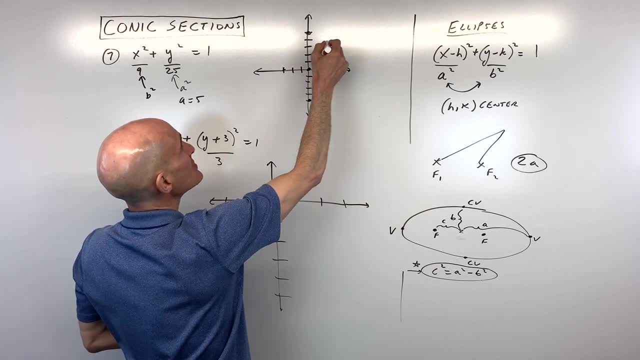 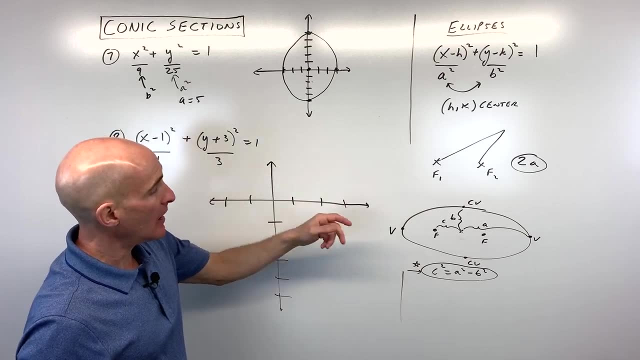 So I'm gonna go right three and left three, And that gives us a pretty good sketch of our ellipse. The only thing left to really find is the two foci, okay, these two focal points, And the way you do that is by using this formula here: 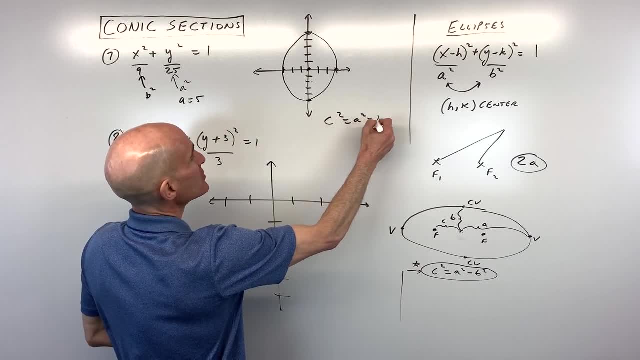 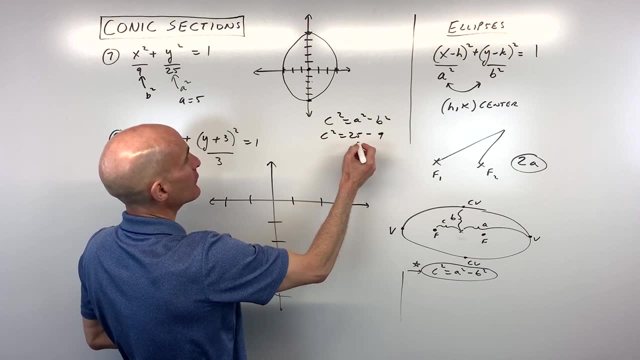 c squared equals a squared minus b squared. So let's go ahead and do that. We've got: a squared is 25, b squared is nine, And if we take this that's 16, and if we take the square root, 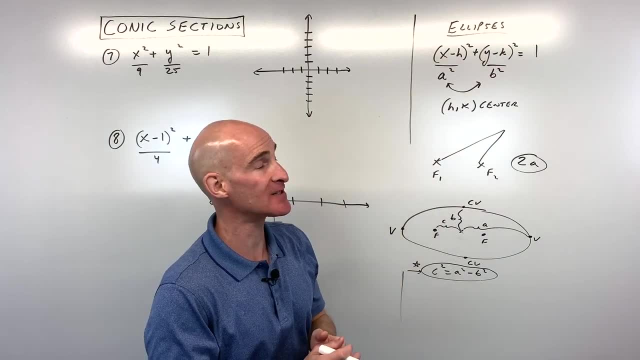 So if I was to cover up the A squared and B squared, it kind of looks like the equation of a circle, doesn't it? 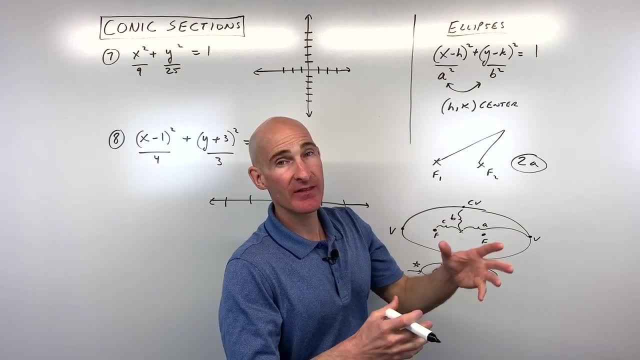 Now, with the A squared and B squared, whichever denominator is larger, that, see, these ones can be interchanged, the denominators. Whichever denominator is larger, that's going to be the A squared one. Whichever one's smaller, that's the B squared one. 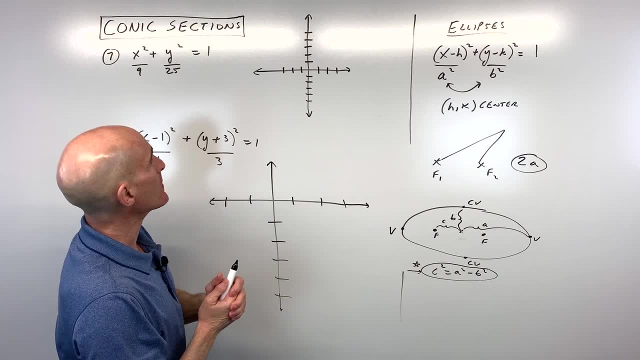 So let me show you through some examples how this works. And I think it'll become a little bit clearer. 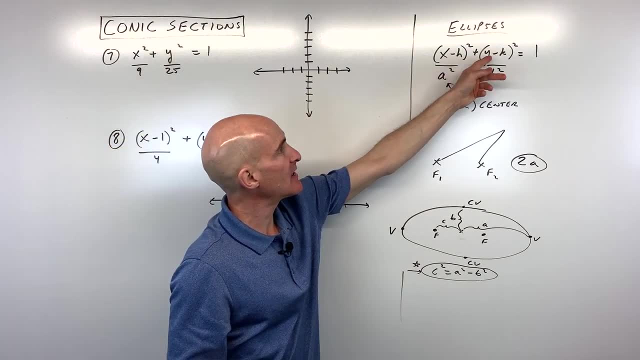 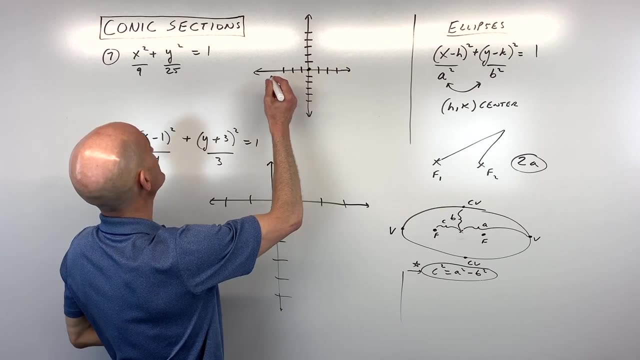 So for number 7, what you'll notice is there's not an H or a K. So that means that the center of the, this ellipse is going to be right at the origin. It hasn't shifted at all. So I'm just going to put a point right here at the origin, 0, 0. 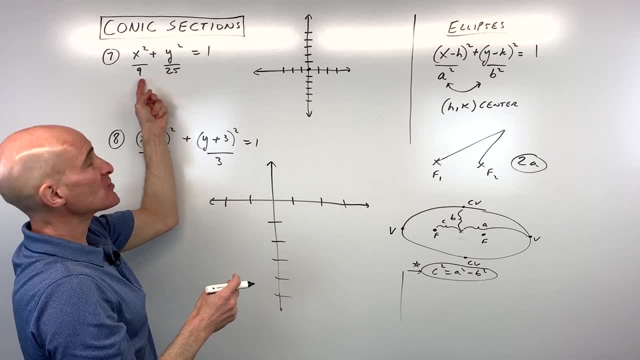 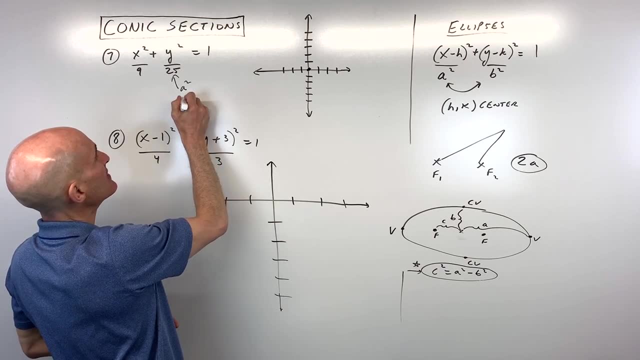 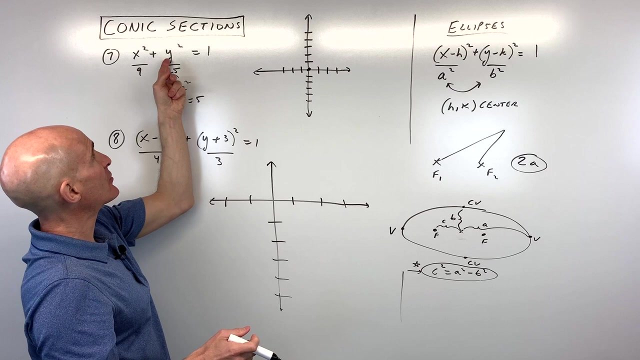 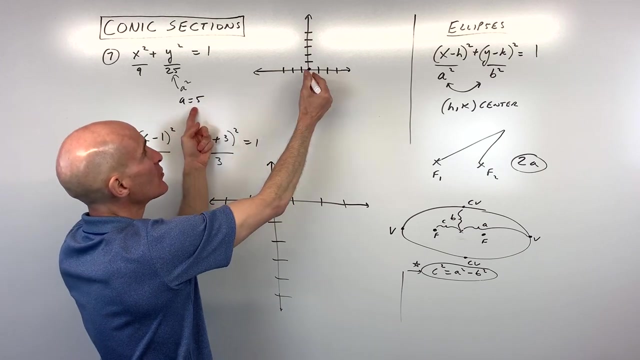 And now when I look at the denominators, see how this denominator here, 25, is greater than 9? That means that this is going to be our A squared right here. So if we take the square root of 25, that means that A is going to be equal to 5. And the other thing you want to pay attention to is that, see, whatever denominator, see, this is underneath the Y, that means you're going to go in the Y direction. Whereas this one's underneath the X, you're going to go in the X direction. So in the Y direction, we're going to be going 5 units, 1, 2, 3, 4, 5 in the Y direction, up and down from the center. So that was our A distance. 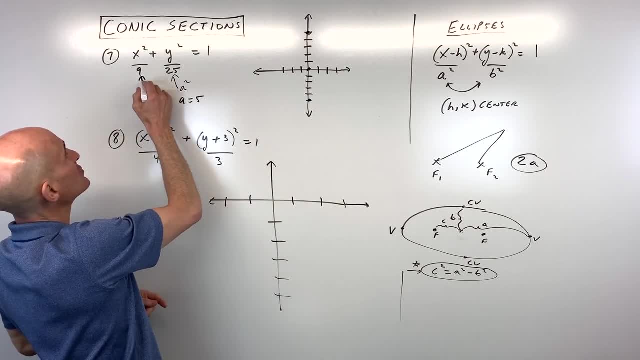 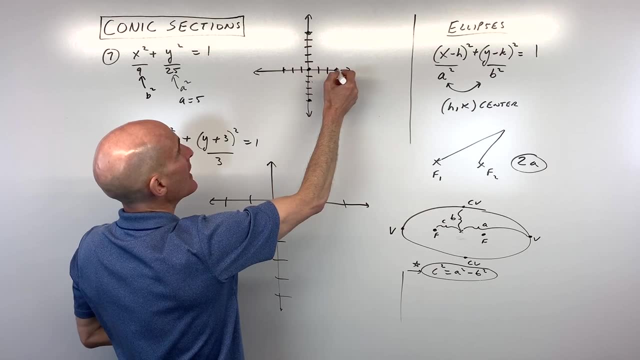 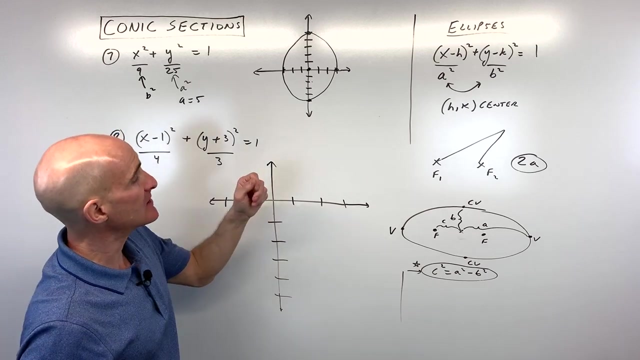 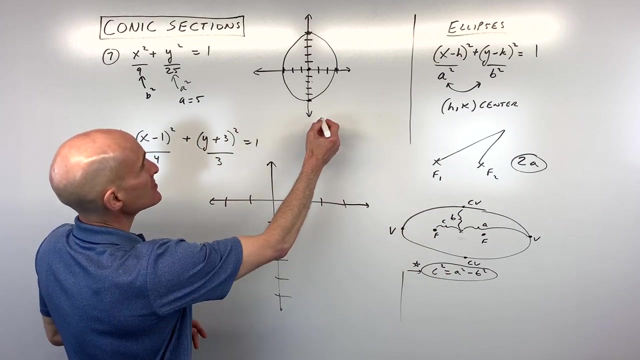 This one here is B squared because that was the smaller denominator. And if we take the square root of 9, you can see we're going to get 3. We're going to go in the horizontal or the X direction. So I'm going to go right 3 and left 3. And that gives us a pretty good sketch of our ellipse. The only thing left to really find is the two foci, these two focal points. And the way you do that is by using this formula here, C squared equals A squared minus B squared. So let's go ahead and do that. 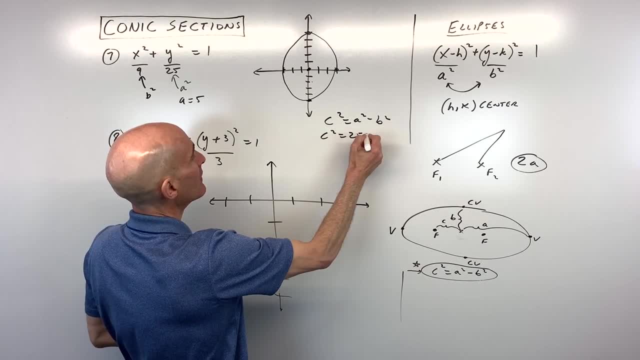 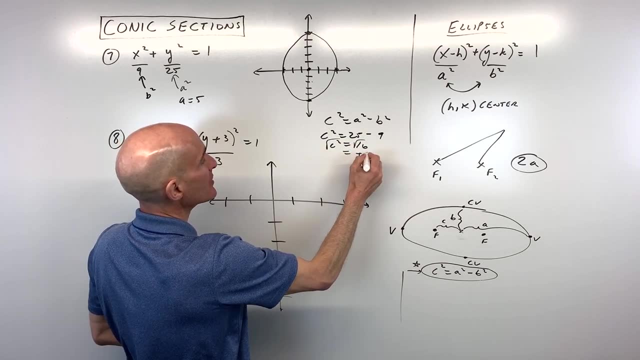 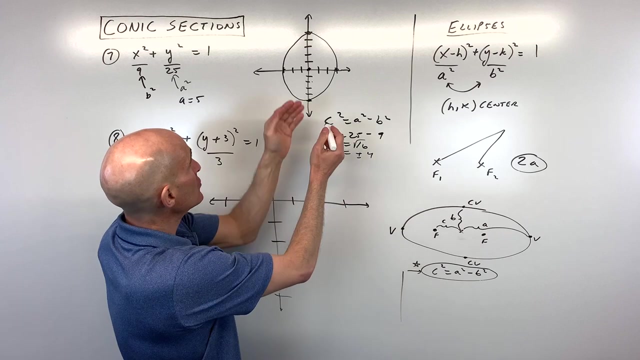 We've got A squared is 25, B squared is 9. And if we take this, that's 16. And if we take the square root, we're getting plus or minus 4. Now, the foci are always going to be along that major axis, that longer axis. So what I'm going to do, see here, this is the longer axis. I'm going to go up 4. That's one foci. And down 4, that's the other foci. 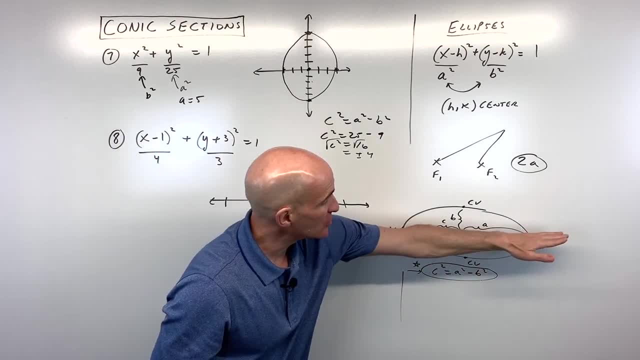 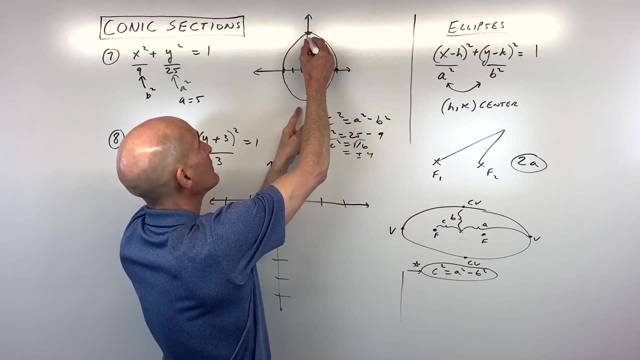 we're getting plus or minus four. Now the foci are always gonna be along that major axis, that longer axis. So what I'm gonna do, see here, this is the longer axis. I'm gonna go up four. that's one foci. 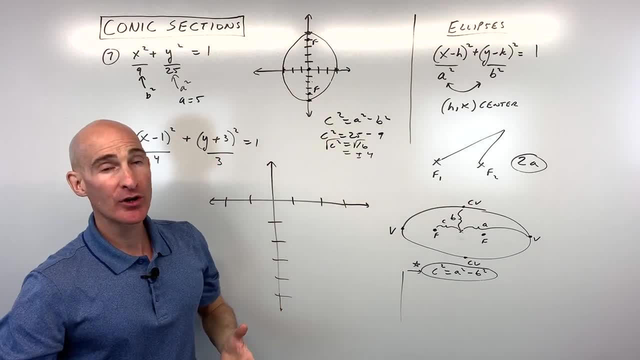 and down four. that's the other foci And you've got a pretty good sketch of your graph. Now we're gonna do number eight. but before I do that, if you're saying you know, Mario, all these problems, 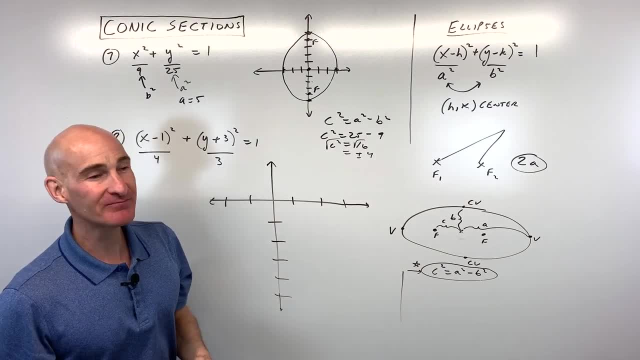 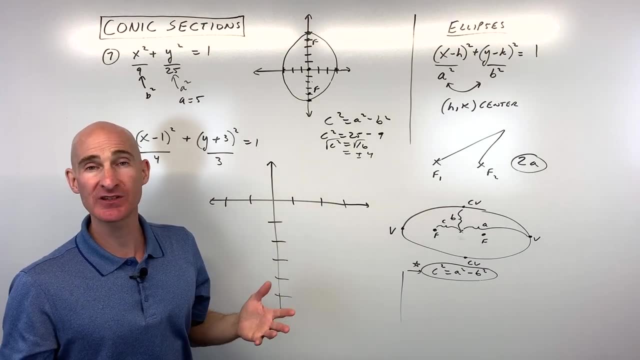 that you're doing are super easy. How about some tougher problems? right In the description I'm gonna put a link to a playlist covering all these different types of conic section problems, So parabolas, ellipses, hyperbolas, et cetera. 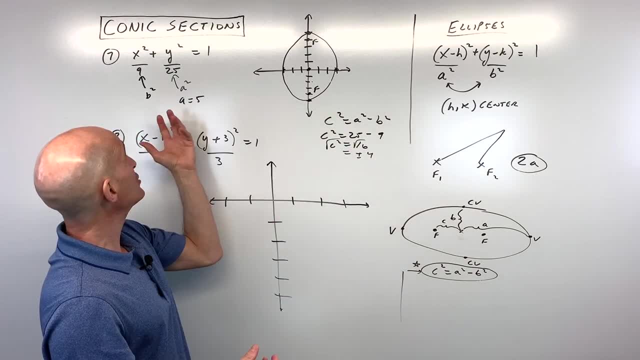 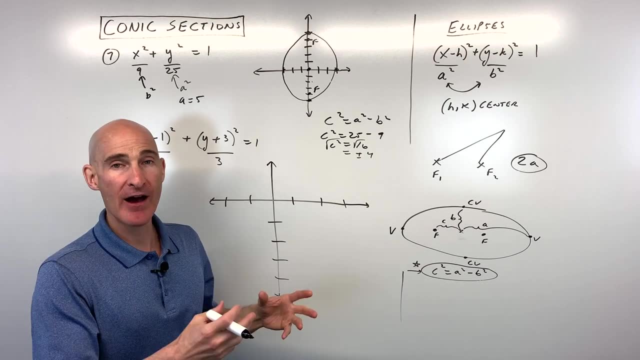 And I'm gonna have different types of problems where you have to put the equation in standard form, or maybe they're gonna give you some details about the particular ellipse, but you have to get the equation or graph it, et cetera, Completing the square, more difficult problems. 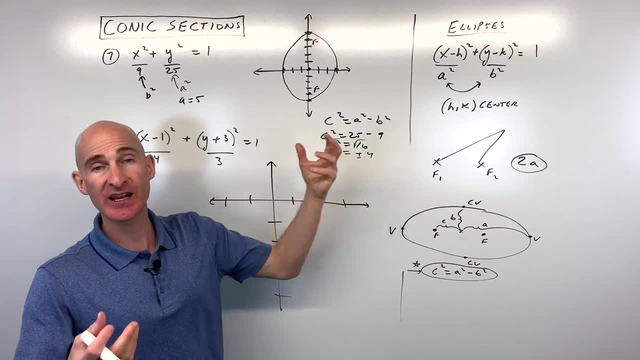 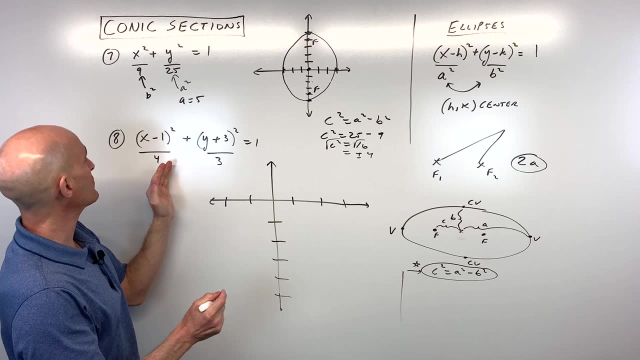 but this is just an introduction to graphing when you already have these in the standard form. So hang with me here. but if you need to see more challenging problems, go ahead and click on that link in the description. But for number eight, what do you think for this one? 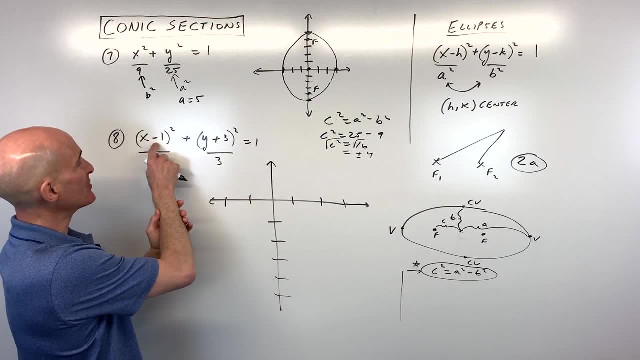 Well, it looks like the center- see, it's shifting right one, down three. or you could say the center is at positive one, negative three. It's gonna be right here. that's our center. Notice that the number underneath the X 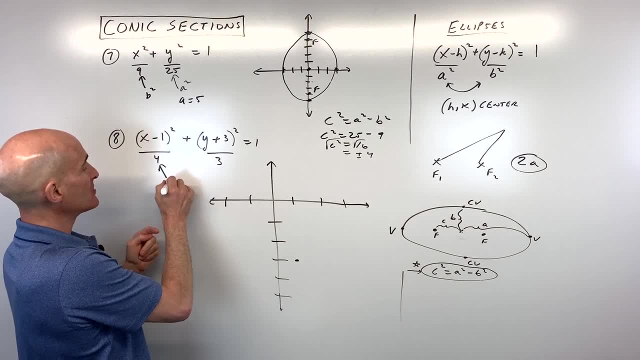 is greater than one underneath the Y. This is gonna be our A squared here. So if we take the square root of four, we get two and we're gonna go in the X direction. So we're gonna go right and left two. 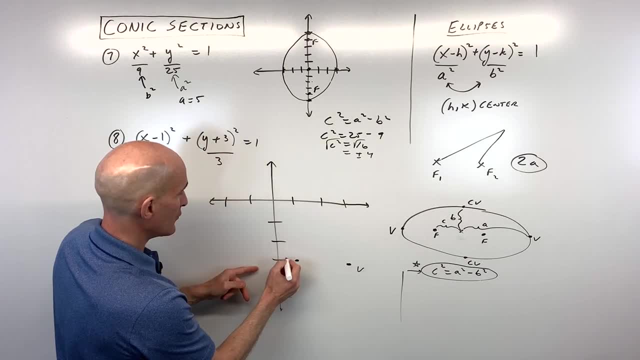 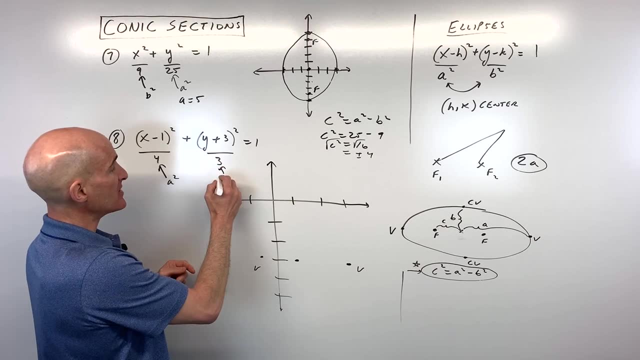 So one, two, okay, that's our vertex, And if we go left, two, that's our other vertex. Now, in the Y direction, we're gonna be going the square root of three. This is like our B squared, So the square root of three is about 1.7.. 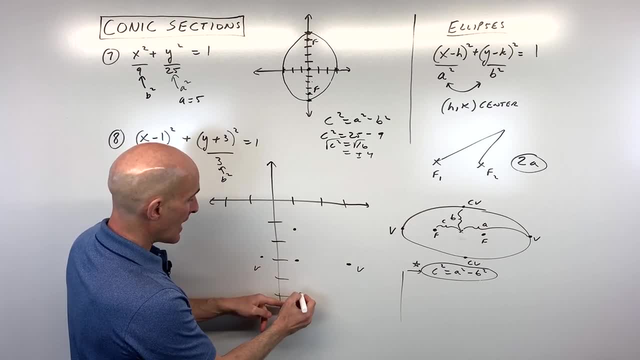 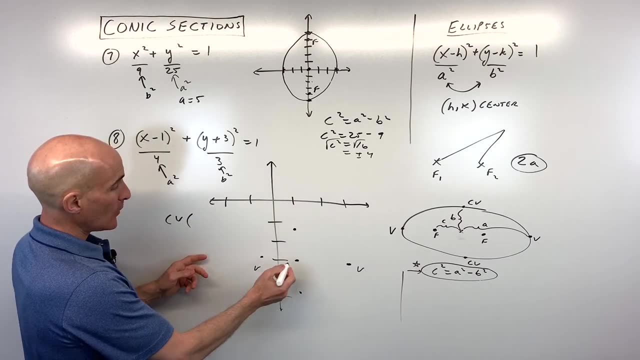 So from the center I'm gonna go up 1.7 and down 1.7.. Now you might be having to write these values. Your teacher might say: what are the coordinates of the co-vertices? Well, you could take that center point. 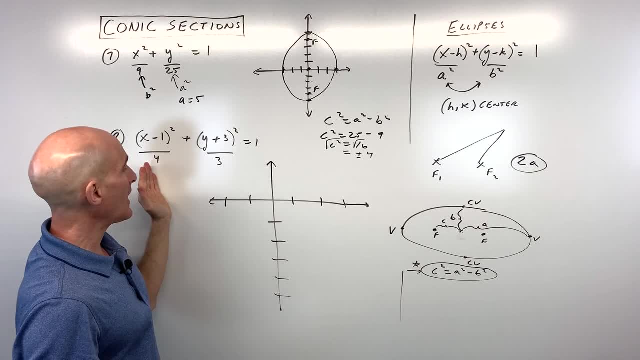 And you've got a pretty good sketch of your graph. Now, we're going to do number 8. 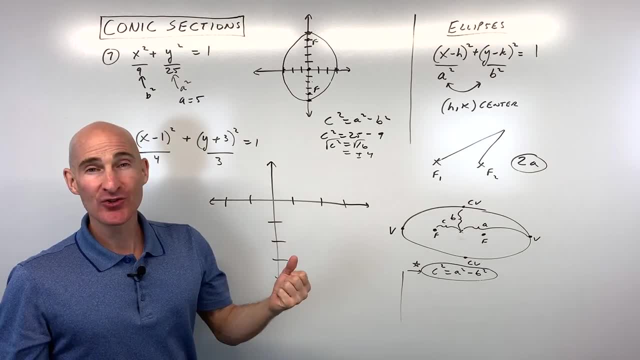 But before I do that, if you're saying, you know, Mario, all these problems that you're doing are super easy. How about some tougher problems, right? 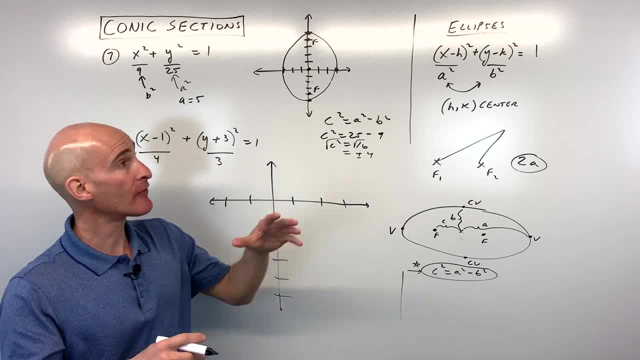 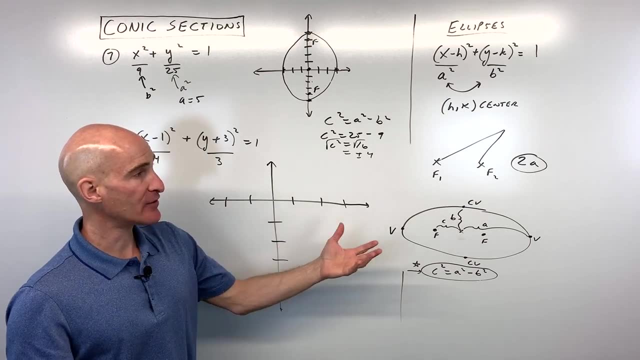 In the description, I'm going to put a link to a playlist covering all these different types of conic section problems. So parabolas, ellipses, hyperbolas, et cetera. And I'm going to have different types of problems where you have to put the equation in standard form or maybe they're going to give you some details about the particular ellipse. 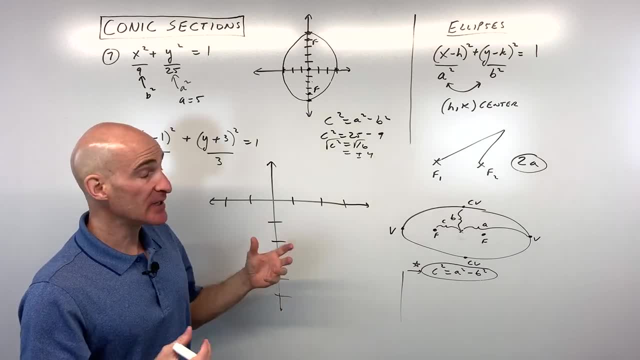 But you have to get the equation or graph it, et cetera. Completing the square, more difficult problems. But this is just an introduction to graphing 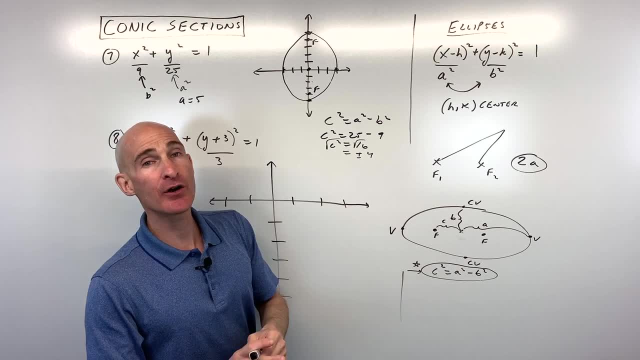 when you already have these in the standard form. So hang with me here. 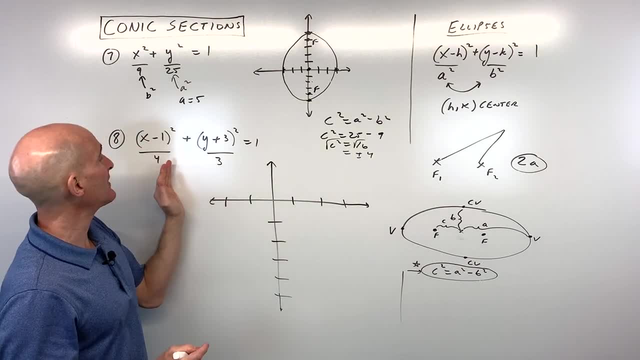 But if you need to see more challenging problems, go ahead and click on that link in the description. 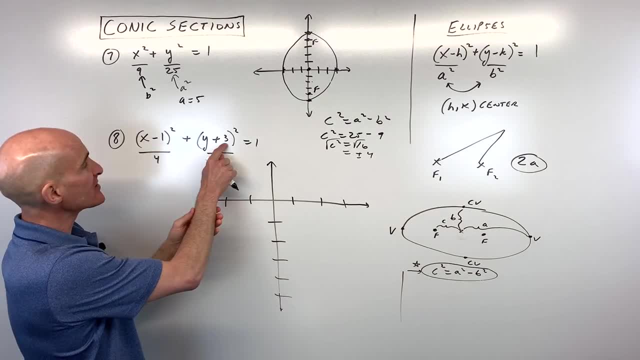 But for number 8, what do you think for this one? Well, it looks like the center, see, it's shifting right 1, down 3. 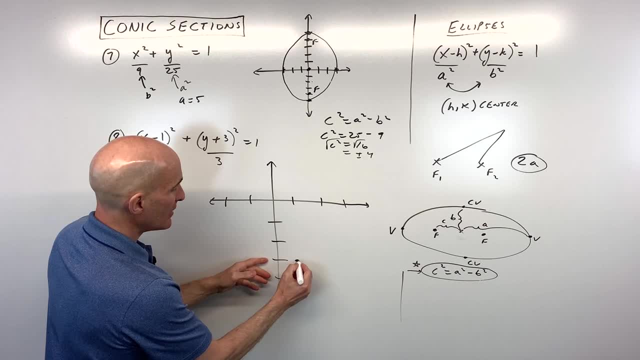 Or you could say the center is at positive 1, negative 3. So that's going to be right here. That's our center. 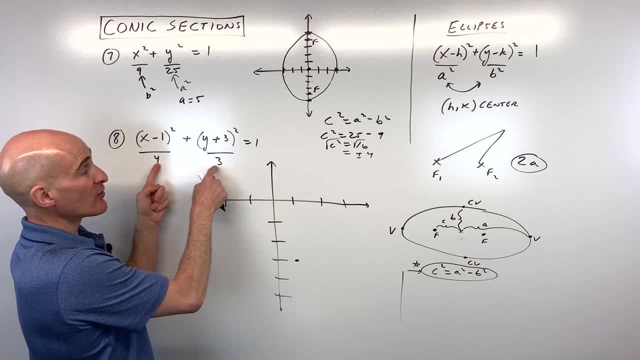 Notice that the number underneath the x is greater than the one underneath the y. This is going to be our a squared here. 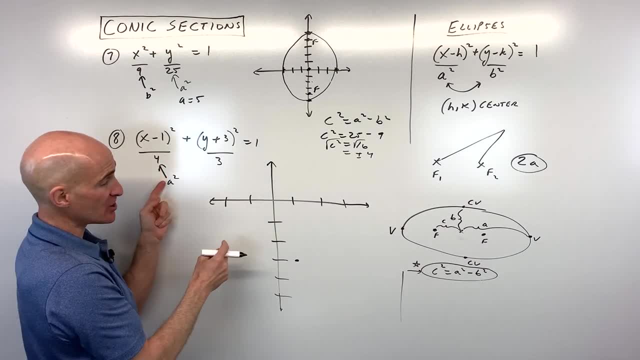 So if we take the square root of 4, we get 2. And we're going to go in the x direction. So we're going to go right and left 2. So 1, 2. OK, that's our vertex. 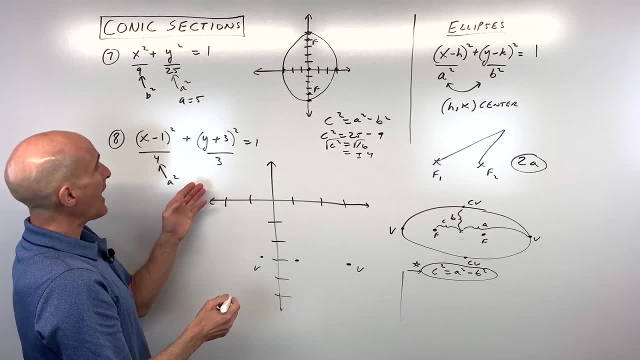 And if we go left 2, that's our other vertex. Now in the y direction, we're going to be going the square root of 3. This is like our b squared. 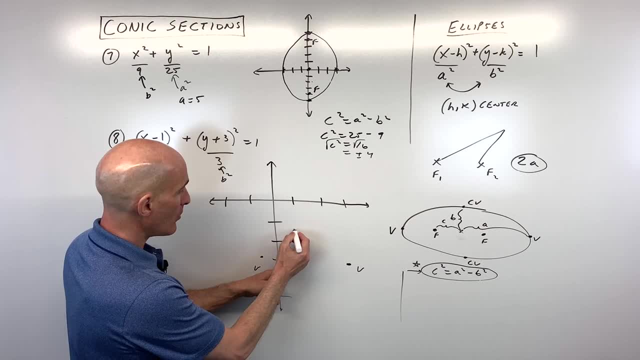 So the square root of 3 is about 1.7. So from the center, I'm going to go up 1.7. And down 1.7. 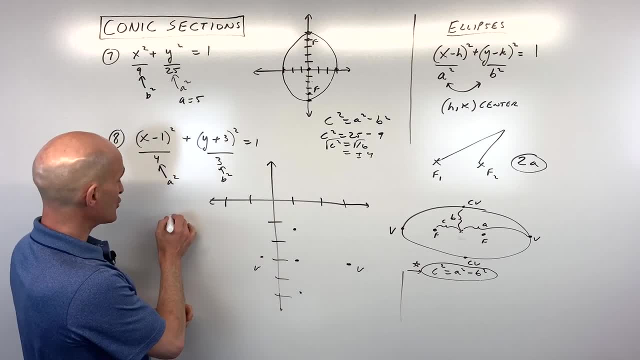 Now you might be having to write these values. Your teacher might say, what are the coordinates of the co-vertices? Well, you could take that center point, which is 1, negative 3, right? But because I'm going up square root of 3 and down square root of 3 from the center, I'm going to say from the y coordinates, we're going the y direction, I'm going to add or subtract square root of 3. 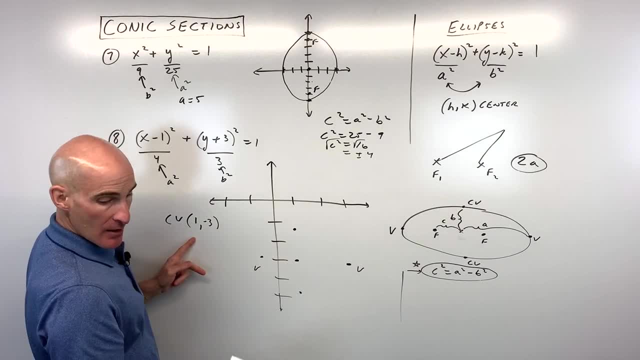 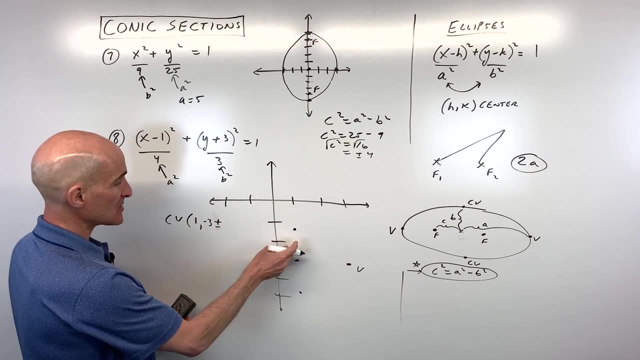 which is one negative three right. But because I'm going up square root of three and down square root of three from the center, I'm gonna say from the Y coordinates we're going the Y direction. I'm gonna add or subtract square root of three. 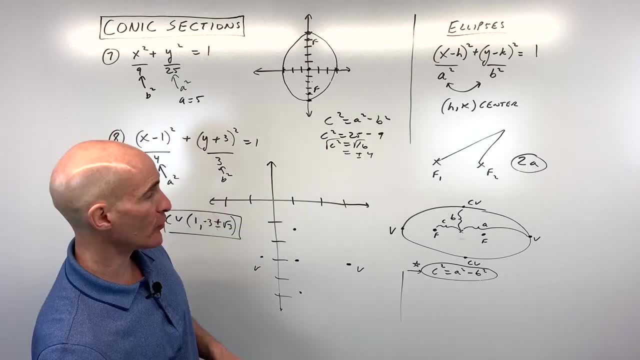 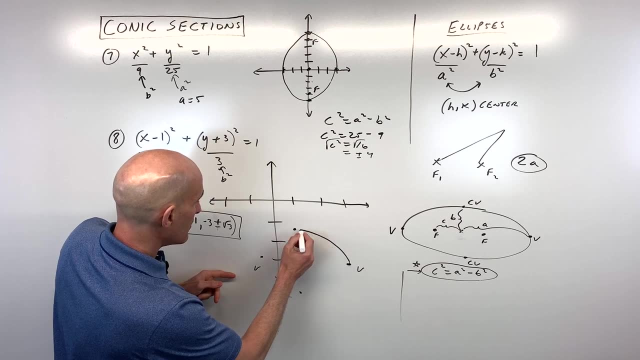 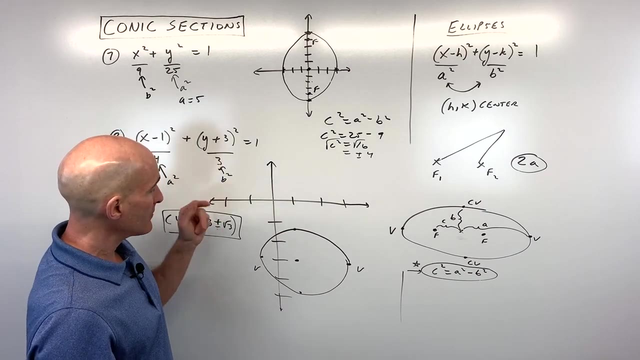 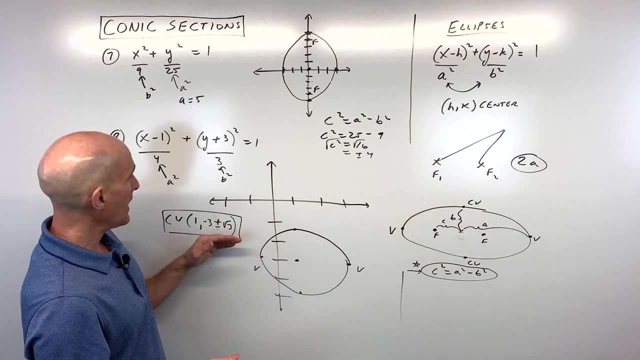 And this is going to give you an exact value of those locations of the co-vertices. But here we're just kind of practicing the scale. The sketching or the graphing. So now you can see this is our ellipse, kind of like this. It looks kind of almost like a circle because see how these values are really close to one another, 4 and 3. The last thing we want to figure out are where are the foci. Now the foci are going to be along the longer axis, the major axis. And we're going to use our formula, c squared equals a squared minus b squared. So let's go ahead and do that. 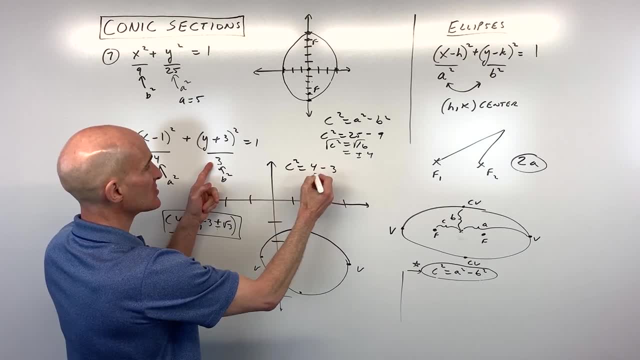 So c squared equals a squared, which is 4, minus b squared, which is 3. So that means c squared equals 1. 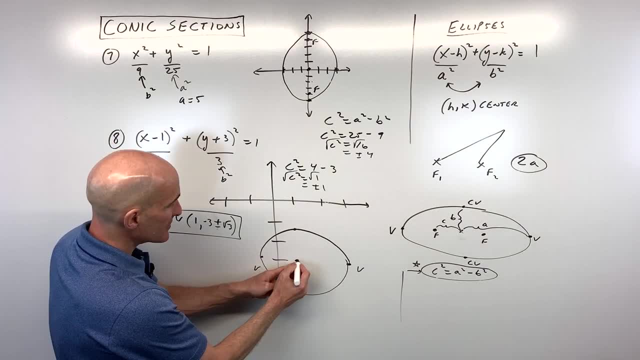 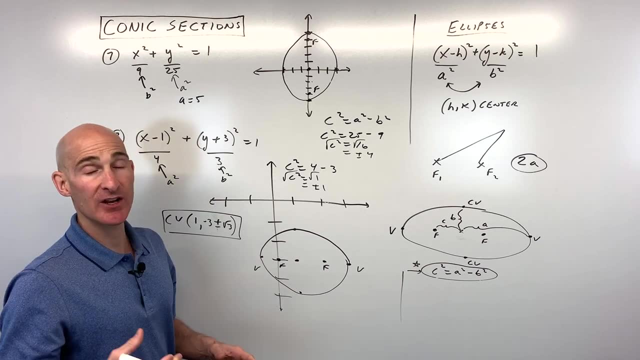 And then squared of both sides, we get plus or minus 1. So from here, the center, I'm going to go right one, which is right about there. And I'm going to go left one, which is right about there. Those are our two foci, and you got it. 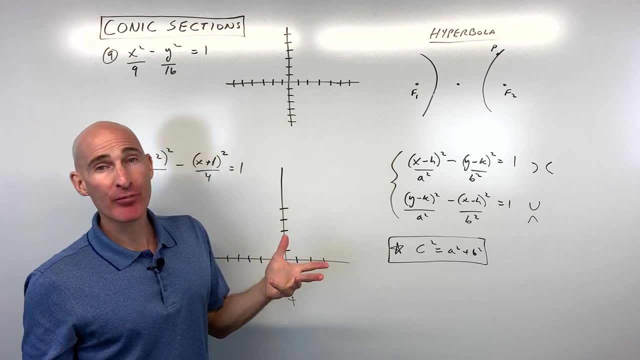 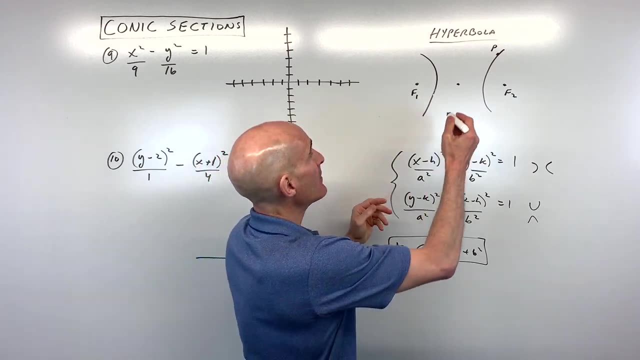 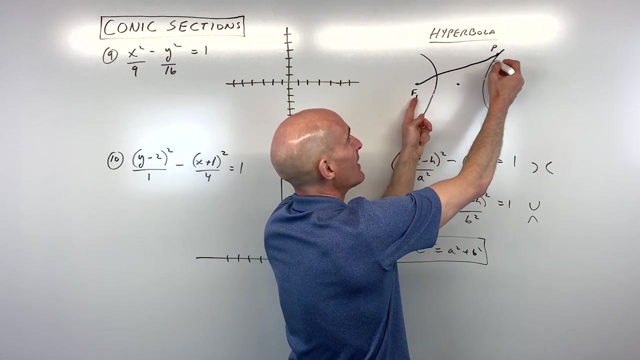 Okay, now we're going to talk about hyperbolas. And what exactly is a hyperbola? Well, technically speaking, what a hyperbola is, it's the set of points, such that when you take a point on that hyperbola, the distance to one of the foci, minus the distance from that point to the other foci, is a constant, and that constant is 2a. 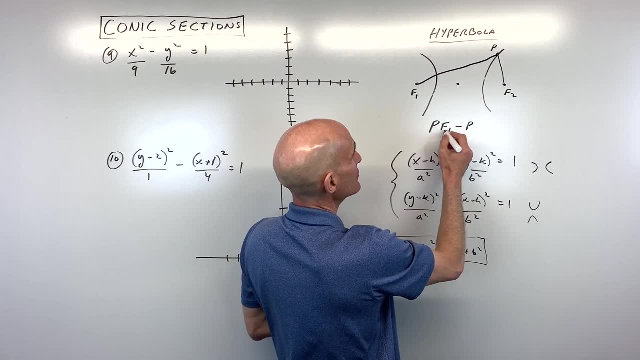 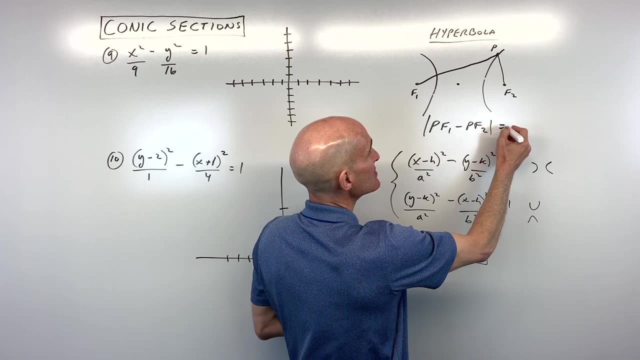 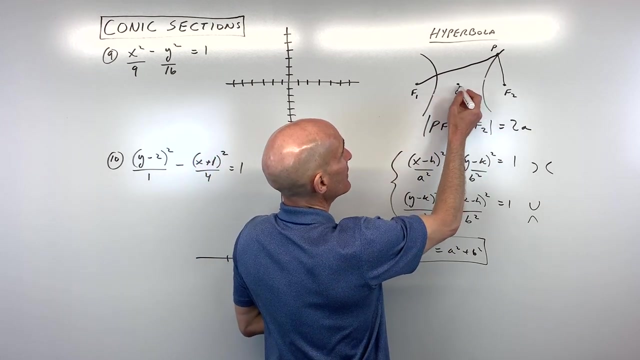 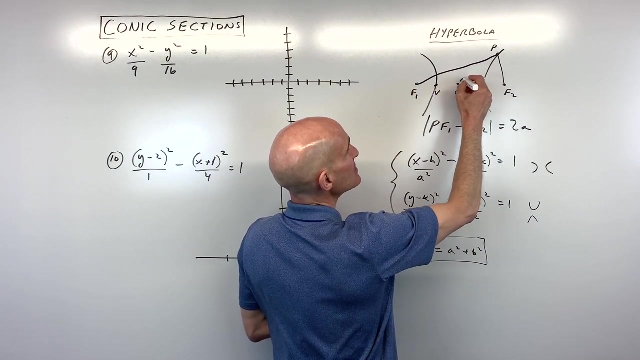 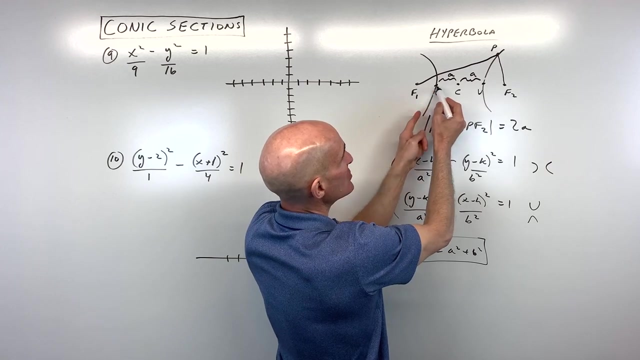 So the way this would look like is, pf1, so the distance from p to the focus 1, minus the distance from that point to focus number 2, if you take the absolute value of that distance, it's always going to equal 2a. And what exactly is this 2a? Well, the center, okay, is going to be halfway between the two foci. The distance from the center to the vertex, this point here or this point here, that distance, just like in an ellipse, we call that distance a. And you can see a plus a, that's 2a, which is the distance between the two vertices. 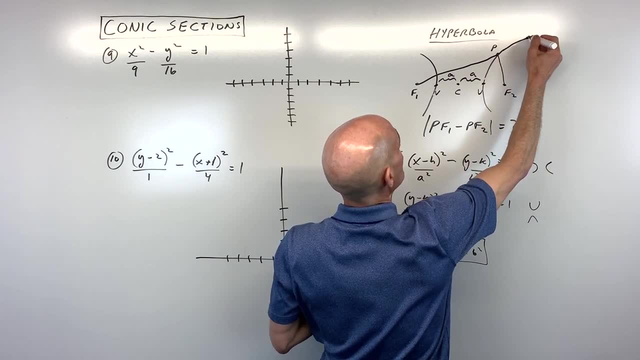 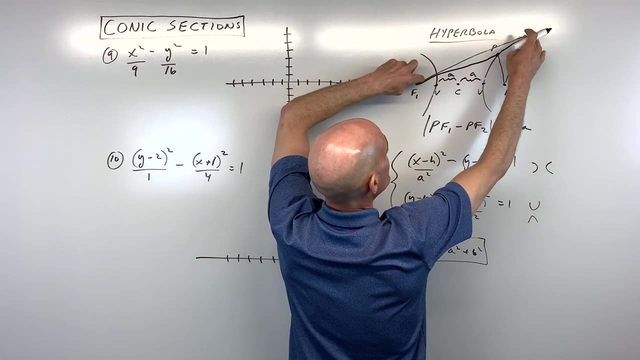 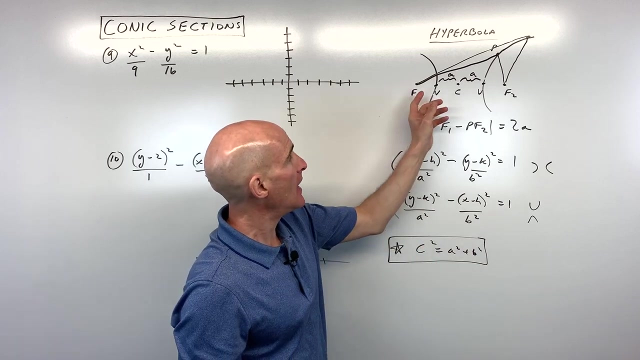 So you can kind of visualize here, if you were to go further out on this hyperbola, see how this length would get longer? See, pf1 would get longer, and then pf2 would also get longer, but when you take that distance minus that distance, it's always going to be a fixed length of 2a, which is the same as the distance between the closest that the hyperbolas come to one another, the distance between the two vertices. 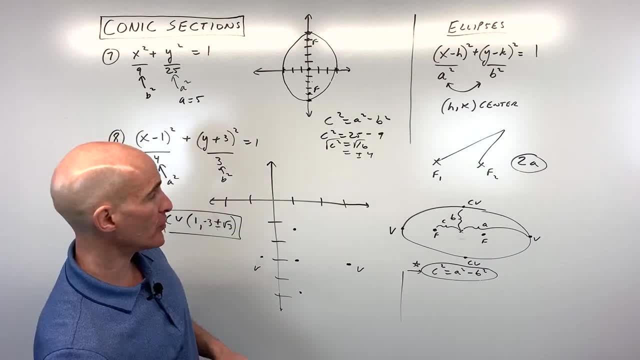 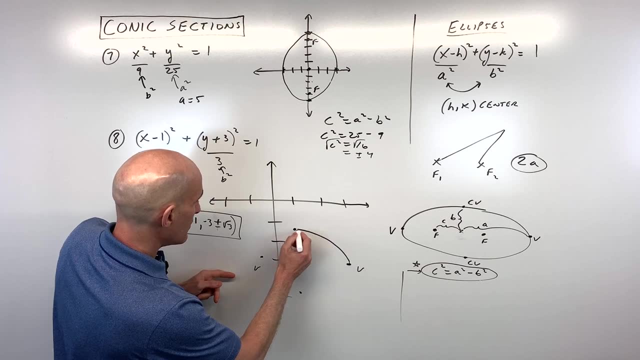 And this is gonna give you an exact value of those locations of the co-vertices. But here we're just kind of practicing the sketching or the graphing. So now you can see, this is our ellipse, kind of like this. It looks kind of almost like a circle. 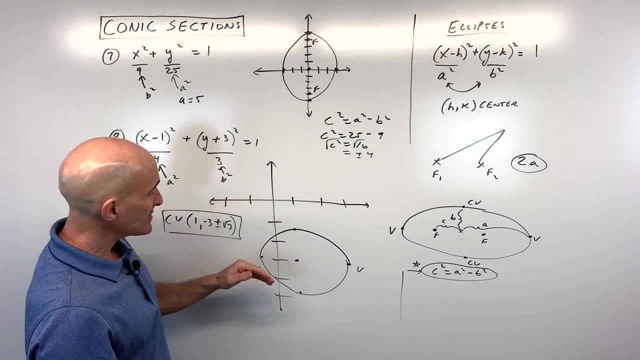 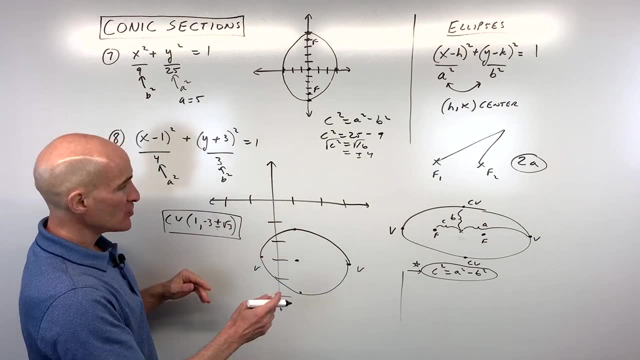 because see how these values are really close to one another. four and three. The last thing we wanna figure out are: where are the foci? Now, the foci are gonna be along the longer axis, the major axis, And we're gonna use our formula. 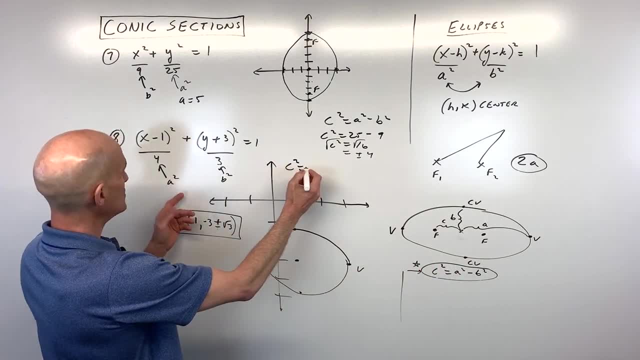 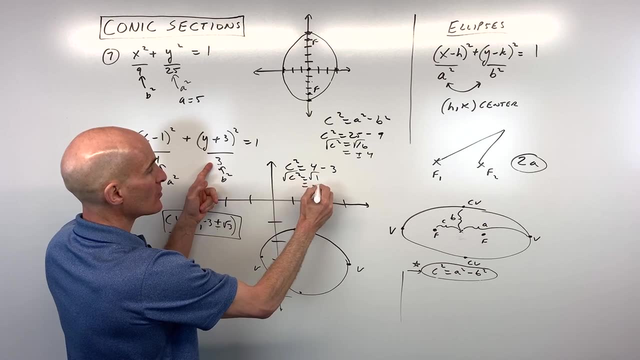 C squared equals A squared minus B squared. So let's go ahead and do that. So C squared equals A squared, which is four, minus B squared, which is three. So that means C squared equals one. And if we take the square root of both sides, 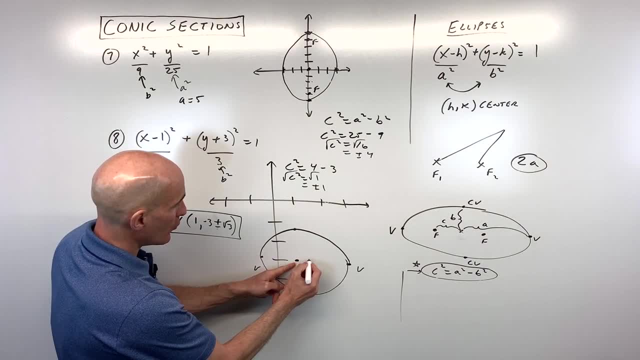 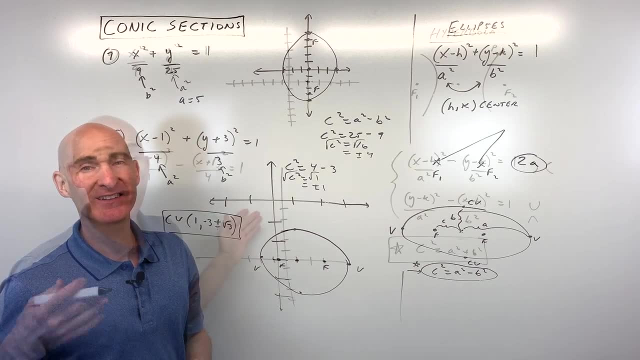 we get plus or minus one. So from here, the center, I'm gonna go right- one which is right about there, And I'm gonna go left one which is right about there. Those are our two foci, and you got it. 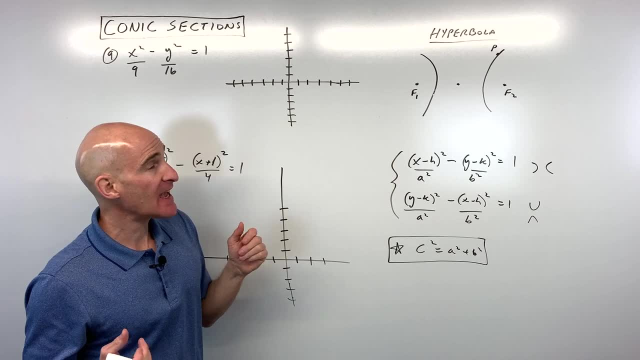 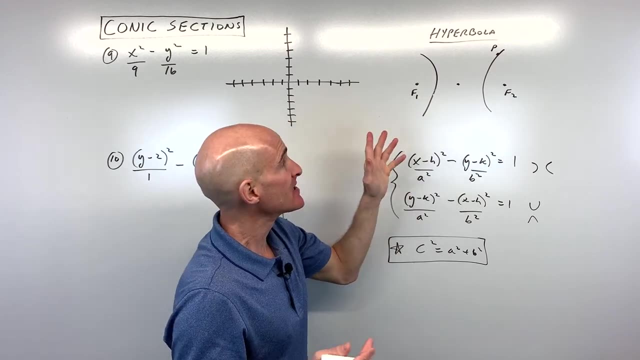 Okay, now we're gonna talk about hyperbolas. And what exactly is a hyperbola? Well, technically speaking, what a hyperbola is? it's the set of points. okay, such that when you take a point on that hyperbola- 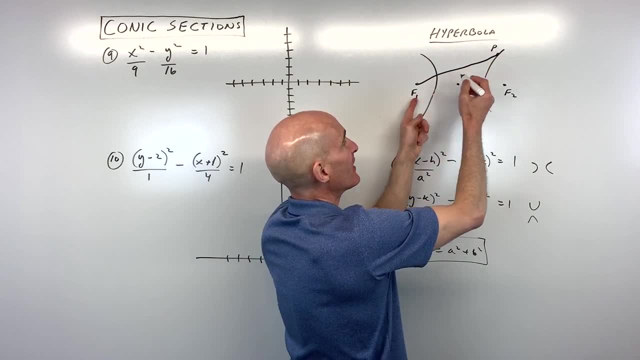 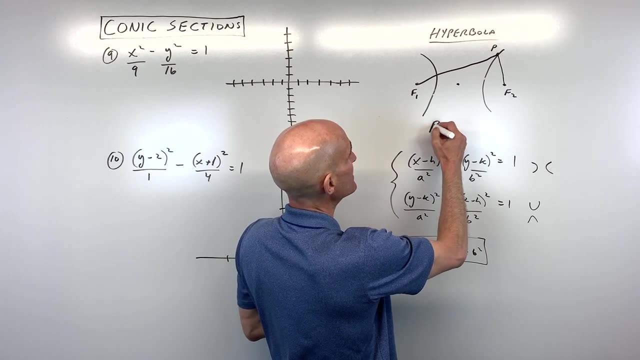 the distance to the distance to one of the foci, okay, minus the distance from that point to the other foci is a constant, and that constant is two A. So the way this would look like is P- F- one. so the distance from P to the focus: one. 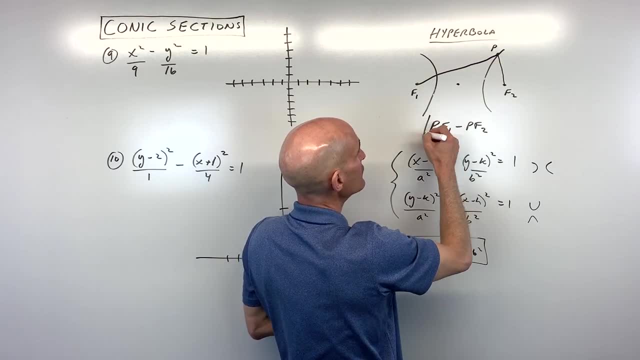 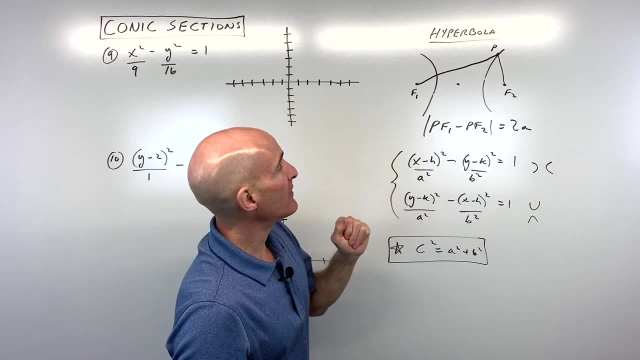 minus the distance from that point to focus number two, If you take the absolute value of that distance, it's always gonna equal two A. And what exactly is this two A? Well, the center, okay, is gonna be halfway between the two foci's. 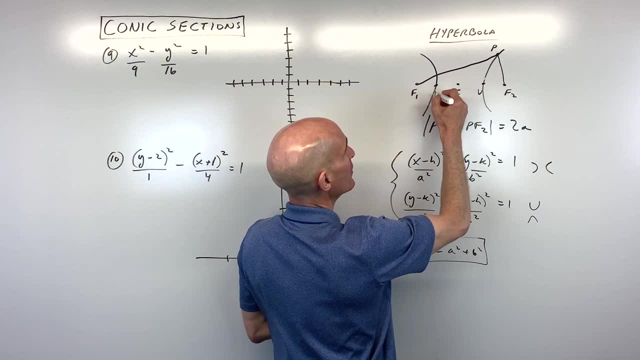 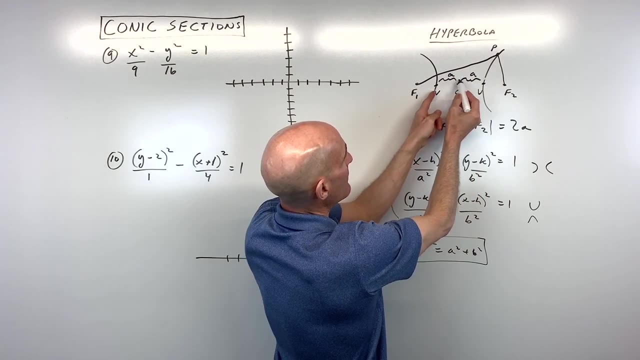 The distance from the center to the vertex, this point here or this point here, that distance, just like in an ellipse, we call that distance A, And you can see: A plus A, that's two A, which is the distance between the two vertices. 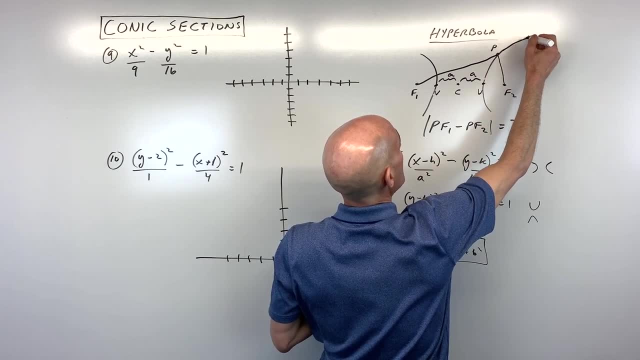 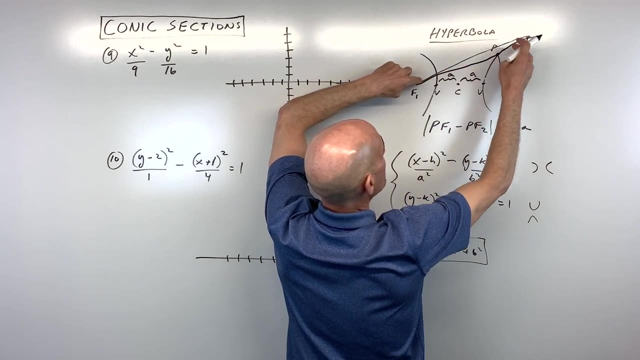 So you can kind of visualize here, if you were to go further out on this hyperbola, see how this length would get longer. See P F one would get longer and then P F two would also get longer. but when you take that distance minus that distance, 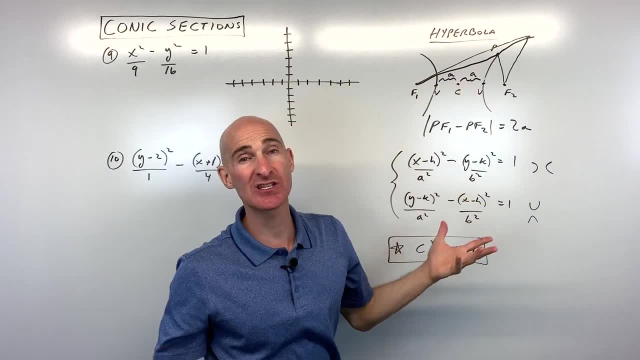 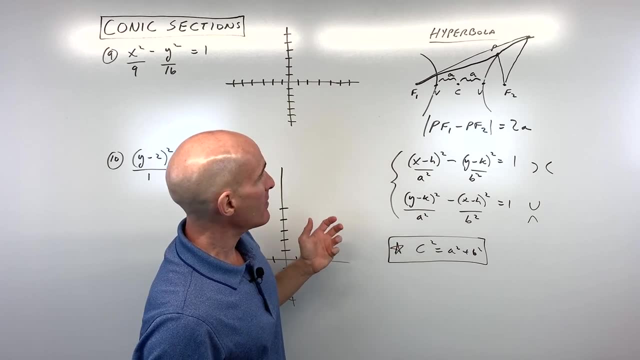 it's always gonna be a fixed length of two A, which is the same as the distance between the closest that the hyperbolas come to one another, the distance between the two vertices. So the other thing you wanna pay attention to here are the two different standard forms. 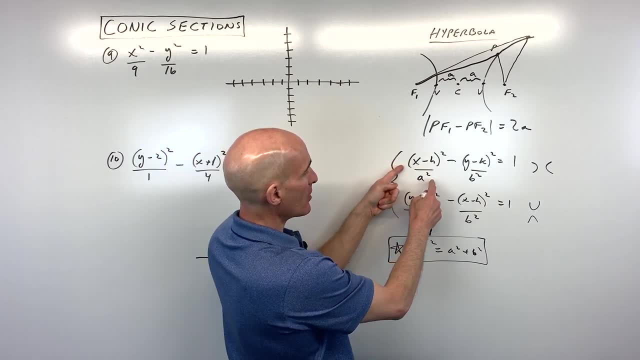 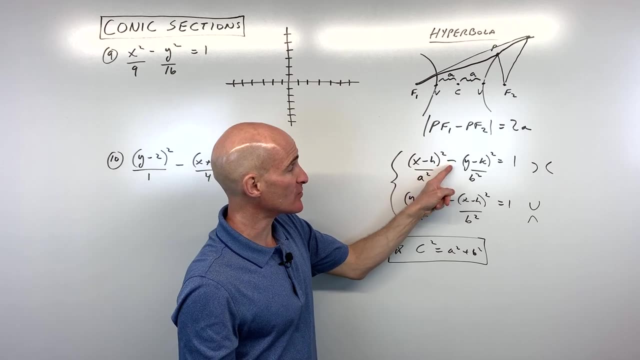 of the equation of a hyperbola, We have this one: X minus H squared, okay. minus Y minus K squared. Notice that it almost looks like the formula of an ellipse. The only difference is that we're subtracting here instead of adding. 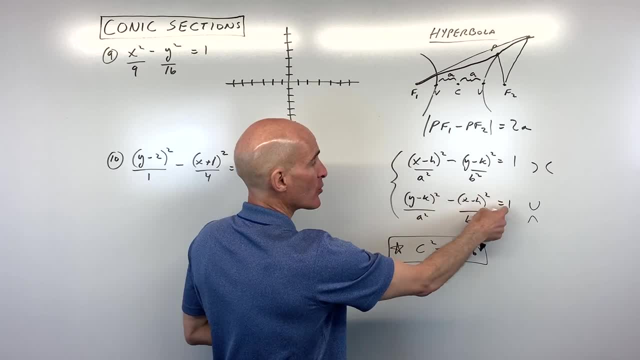 With ellipses, we're adding: Also with ellipses they're equal one, just like hyperbola is equal one. But the key difference here is that the subtraction and you wanna pay attention to whatever term and you wanna pay attention to whatever term. 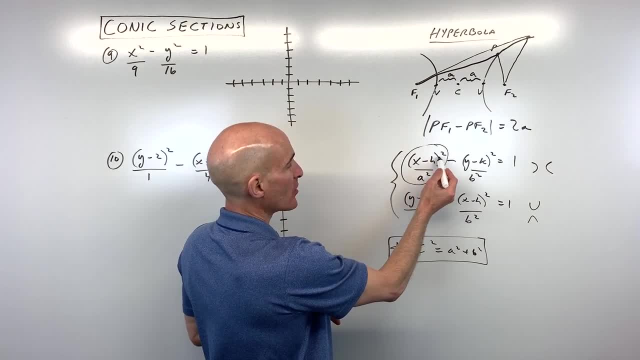 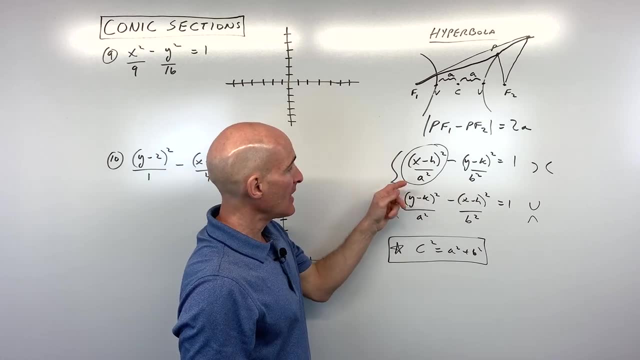 is positive. See how this is. X squared term is positive. That means it's gonna be opening in the X direction, like the horizontal direction left and right, And whatever number is the positive one, the denominator. that denominator is gonna be the A squared. 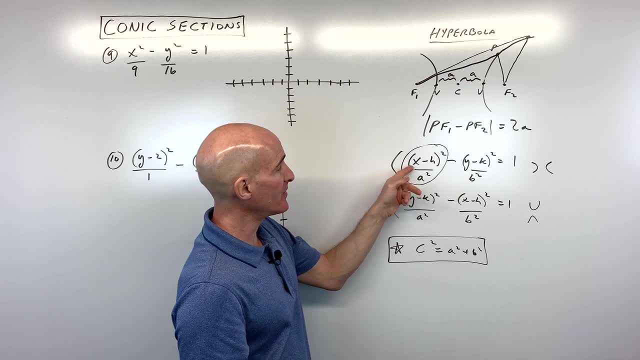 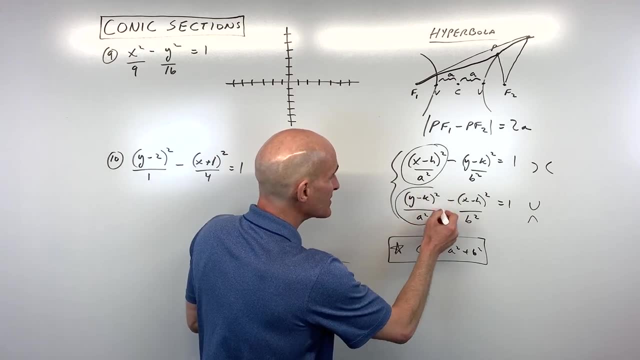 Whereas within ellipses, remember, the larger denominator was the A squared, Here it's the one that's underneath the positive one, That's the first term, which is the positive one, which is gonna be your A squared. So this one, see how this is Y minus K squared. 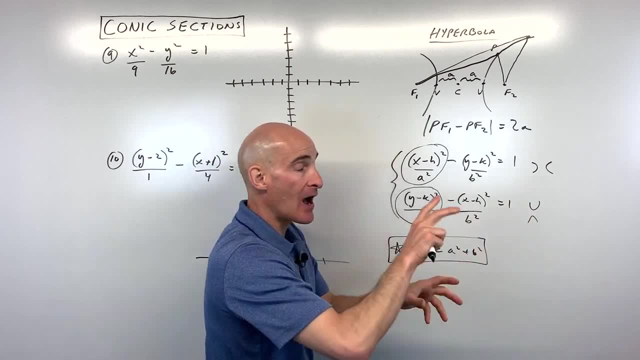 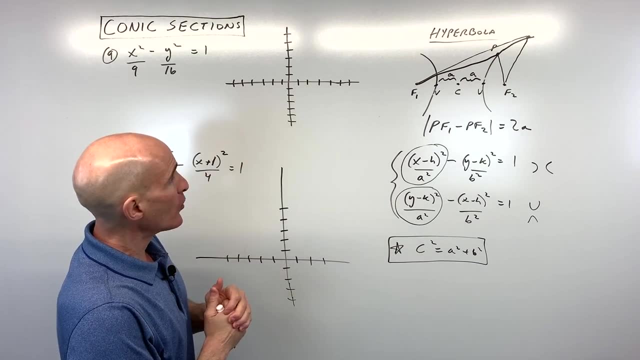 is our positive term or our first term. This is gonna open up and down, like in the Y direction. We're gonna go through a couple examples and I'll talk about it as we go through The only other thing we wanna pay attention to here. 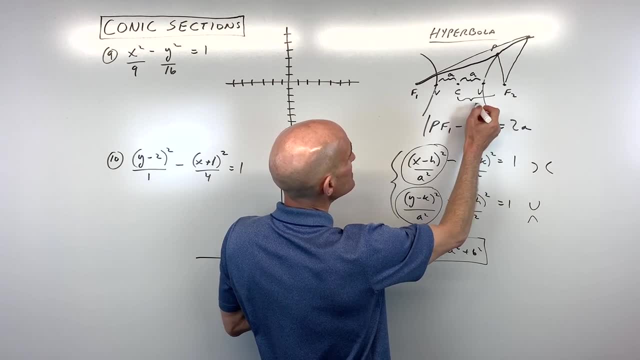 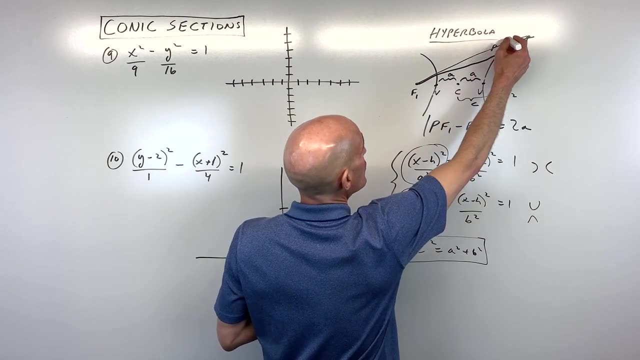 is the distance from the center to the focus. That distance we call C. just like in an ellipse, that distance was C And then B. we're gonna use that to get the equations of our asymptotes And what the asymptotes are. 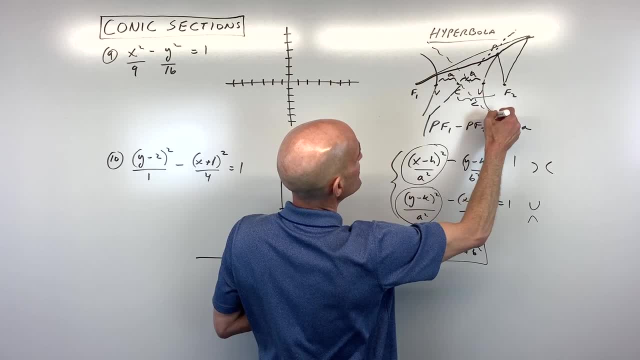 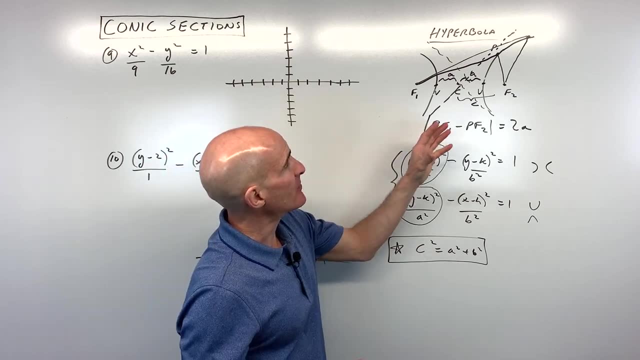 they're like these invisible dashed or dotted lines. They go through the center And the hyperbola's gonna gradually get closer and closer and approach those asymptotes, but not touch them or cross them. So it kinda gives you an idea about how wide the hyperbola is. 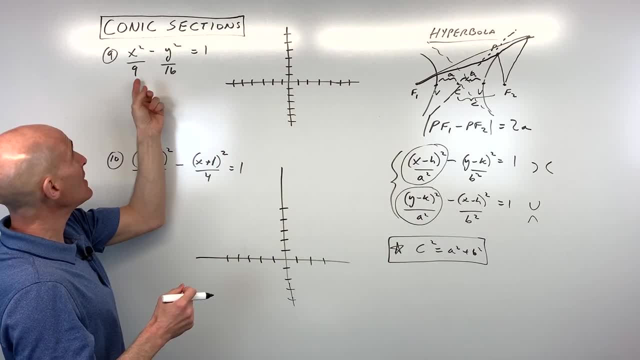 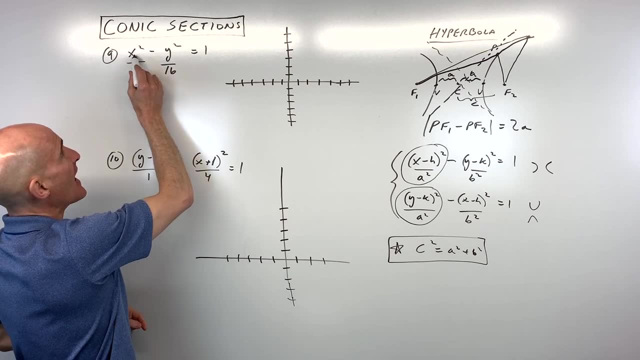 So we'll talk about that in these two examples. So number nine: we notice that this hasn't shifted at all, So we know our center point's gonna be right at the origin. here We can see that this is an X squared type. 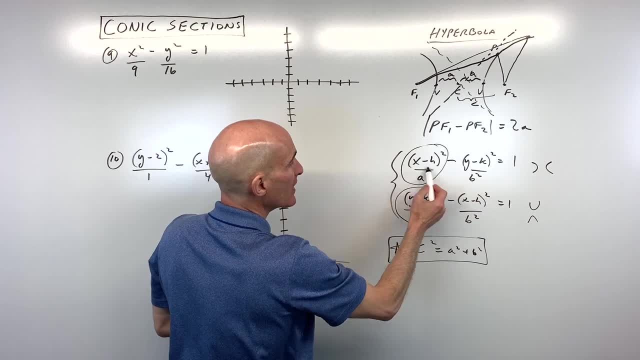 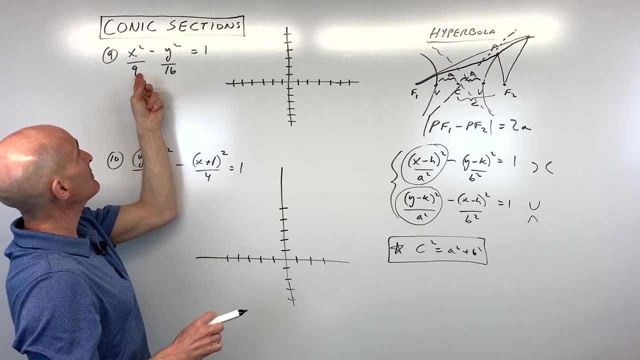 See, this is the positive term: X squared. That tells us it's gonna be in this form right here. It's gonna be opening in the X direction, left and right. So now what I do is I look at this number underneath the X squared. 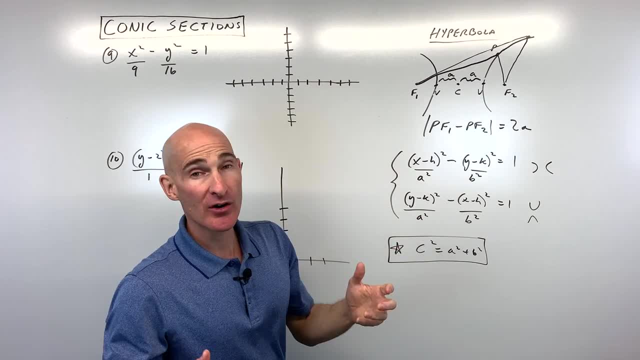 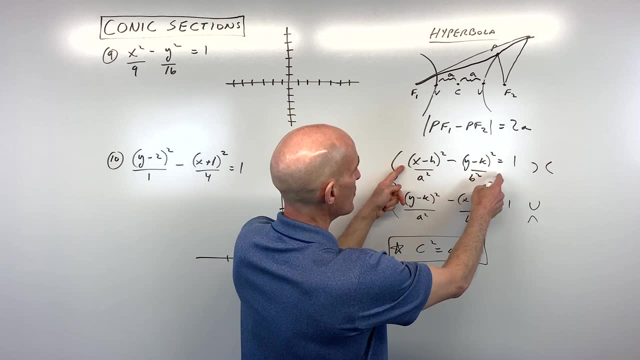 So the other thing you want to pay attention to here are the two different standard forms of the equation of a hyperbola. We have this one, x minus h squared, okay, minus y minus k squared. Notice that it almost looks like the formula of an ellipse. 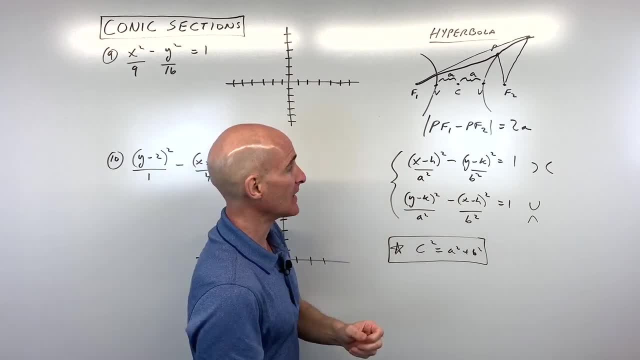 The only difference is that we're subtracting here instead of adding. With ellipses, we're adding. Also with ellipses, they're equal 1, just like hyperbola is equal 1. 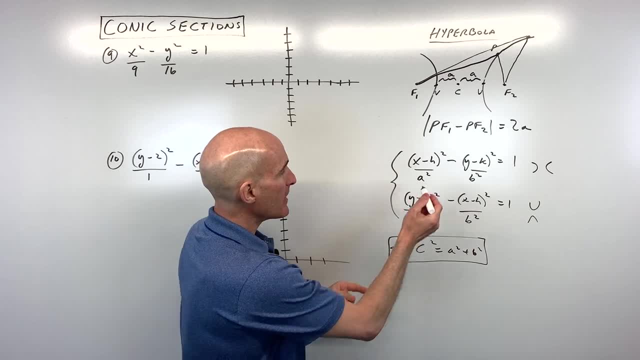 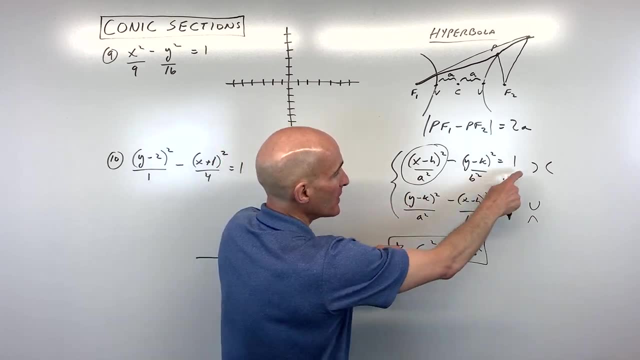 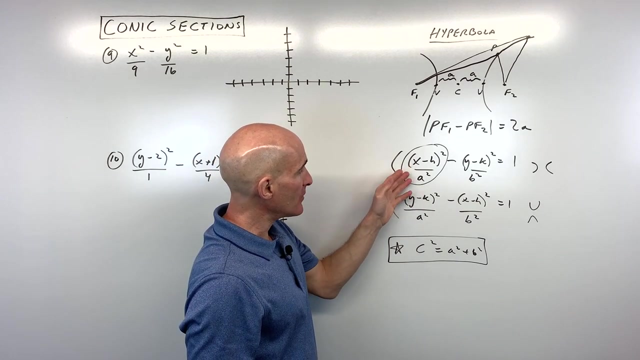 But the key difference here is the subtraction. And you want to pay attention to whatever term is positive. See how this x squared term is positive? That means it's going to be opening in the x direction, like the horizontal direction, left and right. And whatever number is the positive one, the denominator, that denominator is going to be the a squared. Whereas within ellipses, remember the larger denominator was the a squared? Here it's the one that's underneath the positive one. 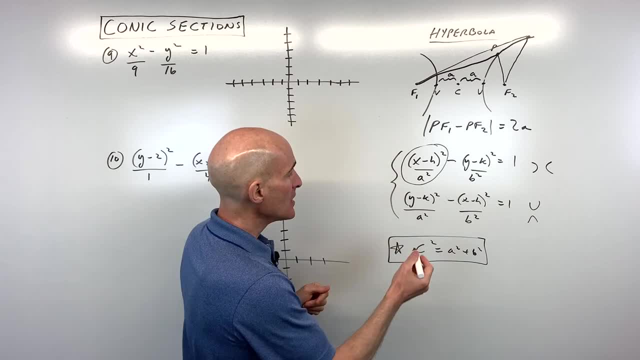 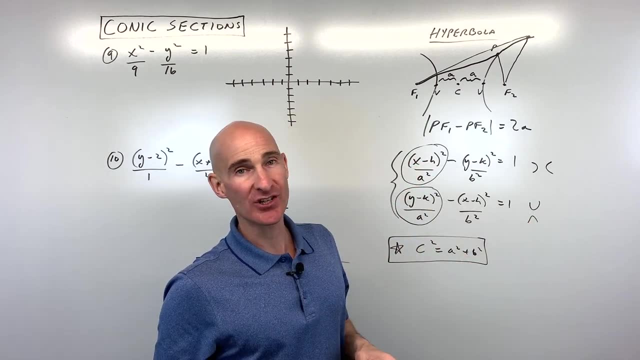 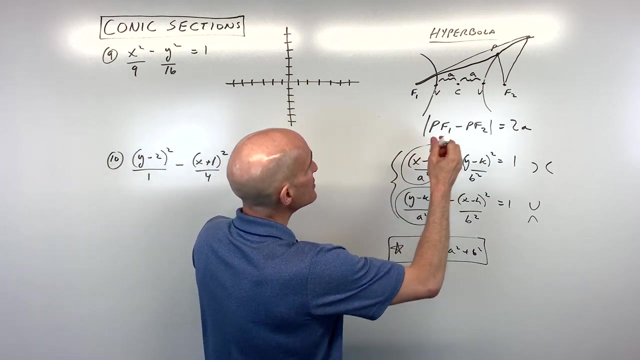 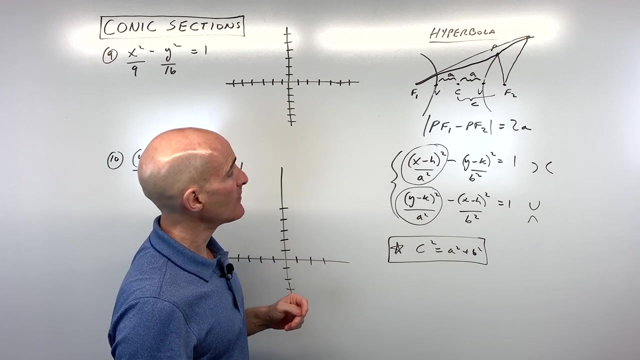 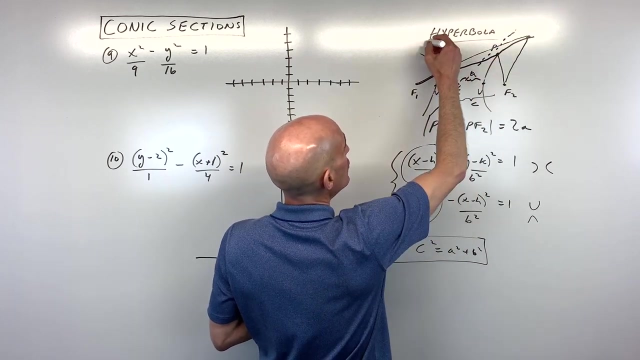 That's the first term, which is the positive one, which is going to be your a squared. So this one, see how this is y minus k squared is our positive term, the first term? This is going to open up and down, like in the y direction. We're going to go through a couple of examples, and I'll talk about it as we go through. The only other thing we want to pay attention to here is the distance from the center to the focus. That distance we call c, just like in an ellipse, that distance was c. And then b, we're going to use that to get the equations of our asymptotes. And what the asymptotes are, they're like these invisible dashed or dotted lines. They go through the center. 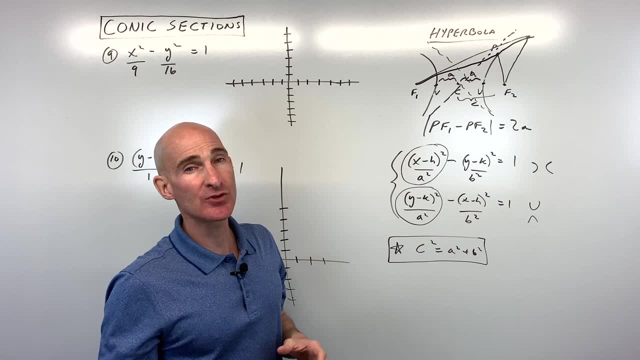 The hyperbola is going to gradually get closer and closer and approach those asymptotes, but not touch them or cross them. So it kind of gives you an idea about how wide the hyperbola is. So we'll talk about that in these two examples. 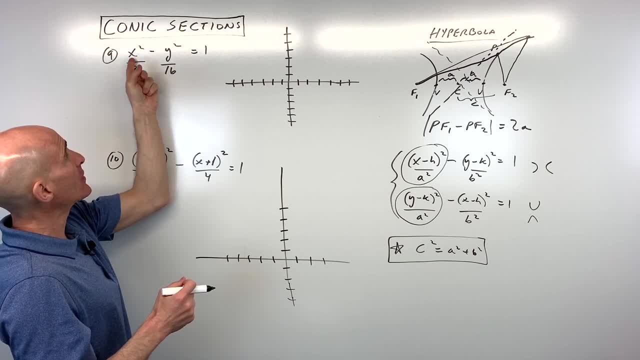 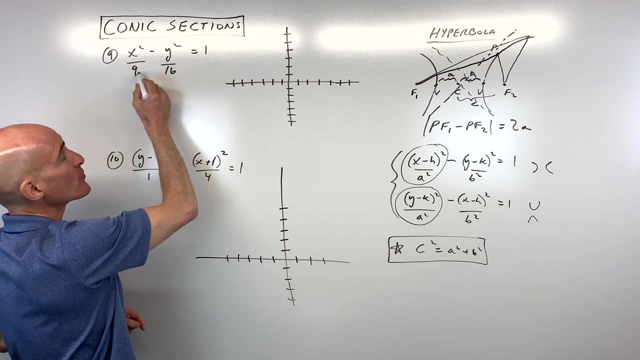 So number nine, we notice that this hasn't shifted at all. So we know our center point is going to be right at the origin here. We can see that this is an x squared type. See, this is the positive term, x squared. That tells us it's going to be in this form right here. 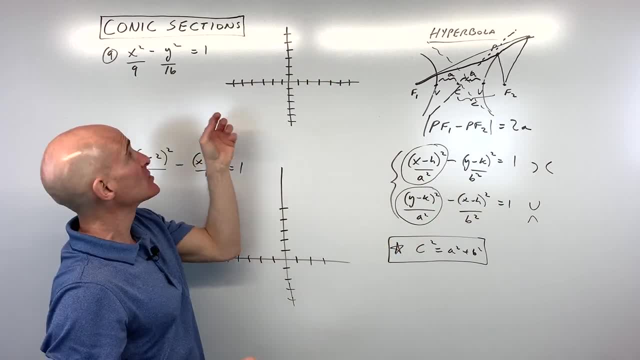 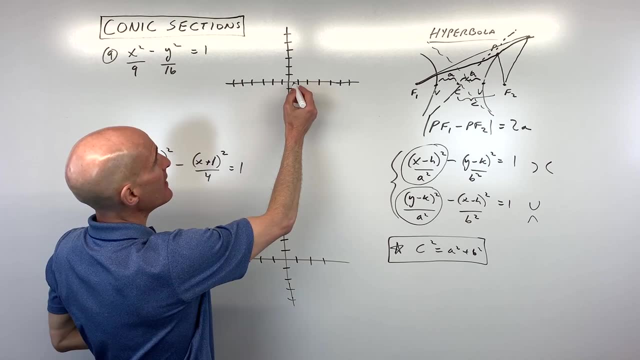 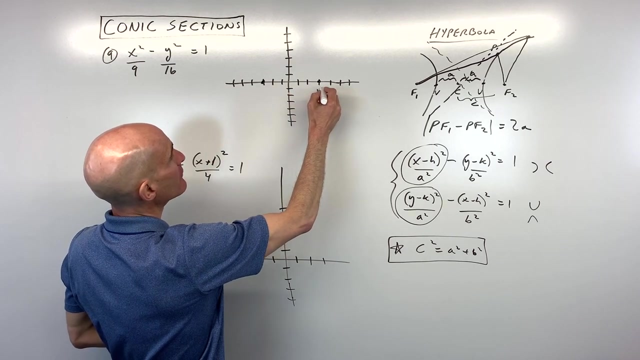 It's going to be opening in the x direction, left and right. So now what I do is I look at this. This number underneath the x squared, this is nine. If I take the square root of nine, that's three. That's our a value. I'm going to go right three, and I'm going to go left three from the center. And that's going to be where our vertices are, okay? 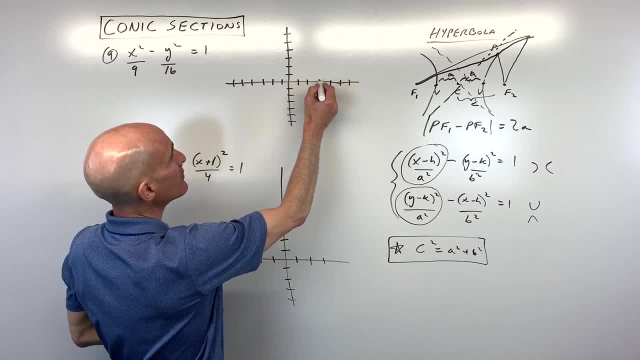 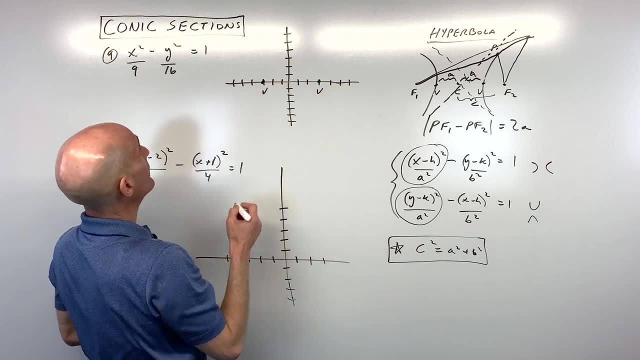 And if I take the square root of nine, that's three. That's our A value. I'm gonna go right- three- and I'm gonna go left three, from the center, And that's gonna be where our vertices are. okay, Now, this number here, this is our B squared. 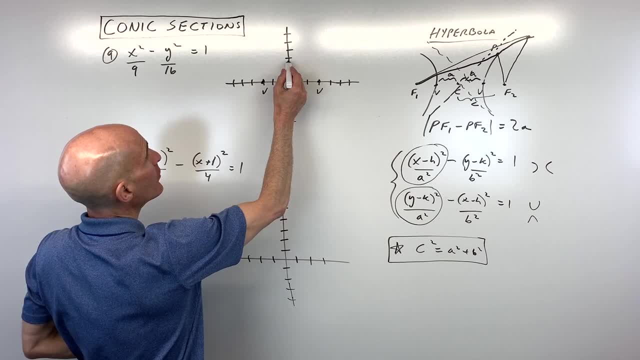 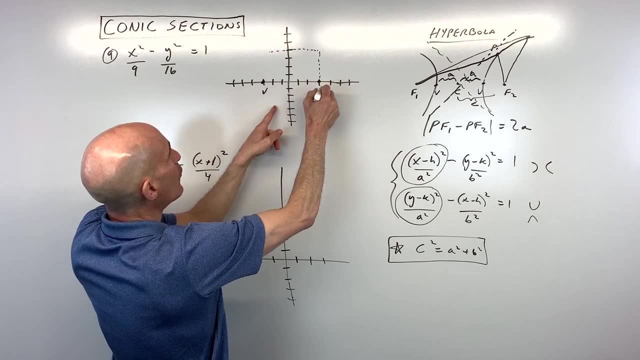 If I take the square root of 16, that's four. I'm gonna go up four and down four And what I'm gonna do is I'm gonna draw a rectangle through these four points. okay, Dashed or dotted rectangle, It's not gonna be part of your graph. 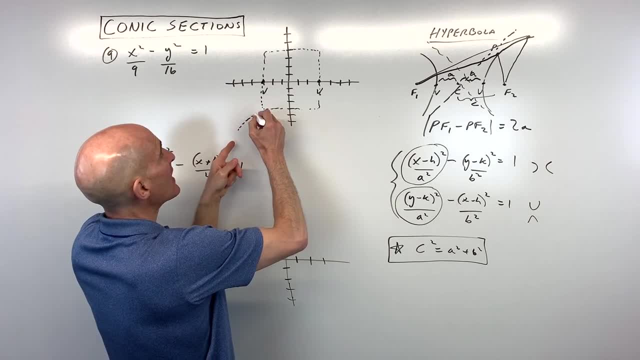 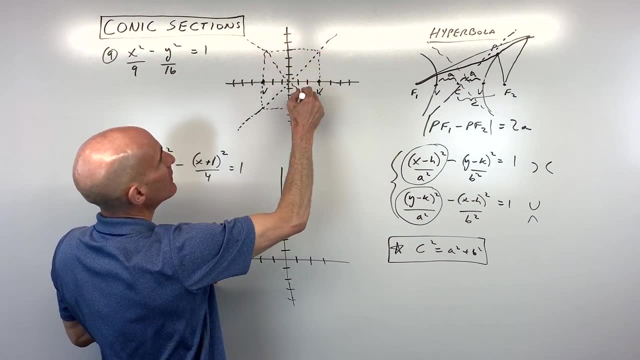 You're just gonna use it as a guide. Then what you do is you draw these dashed or dotted lines- okay, these are our asymptotes- through the corners of the rectangle also goes through the center point. Those are our asymptotes. 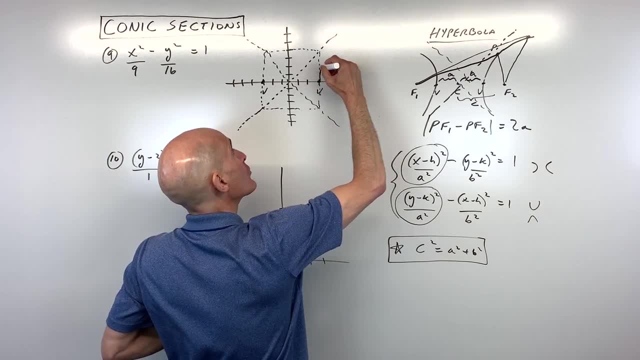 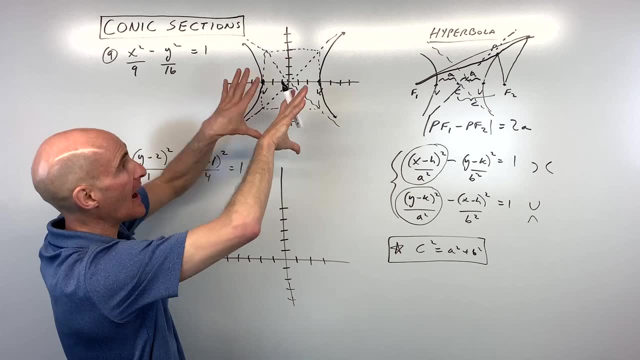 So we're gonna use those asymptotes as a guide to graph our hyperbola. The hyperbola's gonna get closer and closer to those lines, but not touch, not cross. So again, it gives us an idea of how wide the hyperbola is. 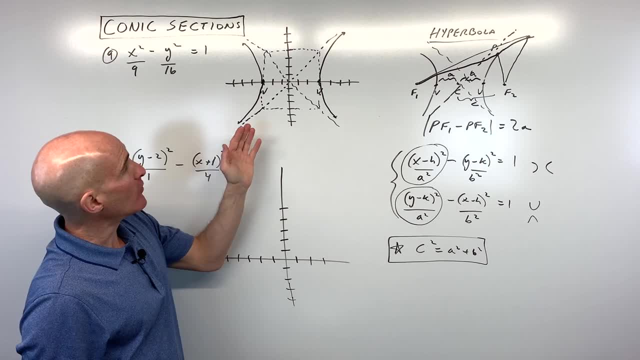 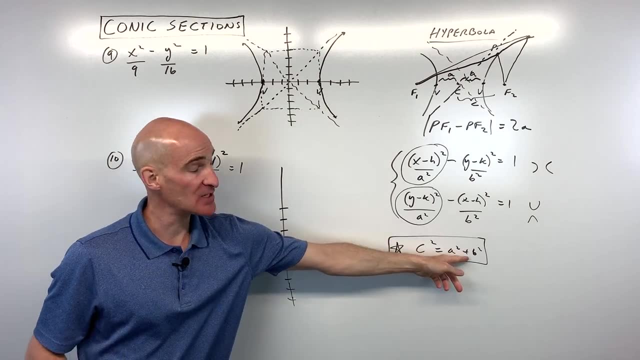 or how narrow depending. The only other thing that we need to figure out are, well, the equations of the asymptotes, as well as the locations of these focal points, these foci, And we use this formula here: C squared equals A squared plus B squared. 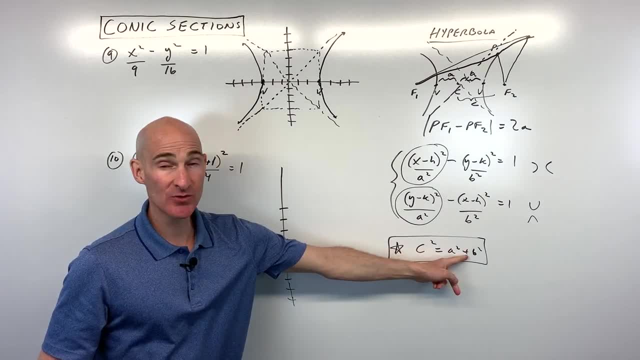 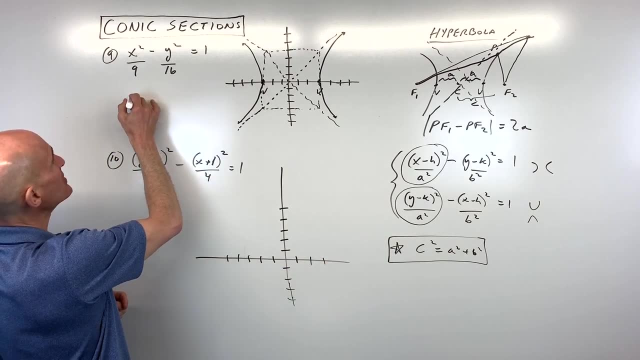 just like Pythagorean theorem. Remember when we were working with ellipses it was C squared equals A squared minus B squared. So very similar, but here we're adding. So, in this case, this is our A squared, this is our B squared. 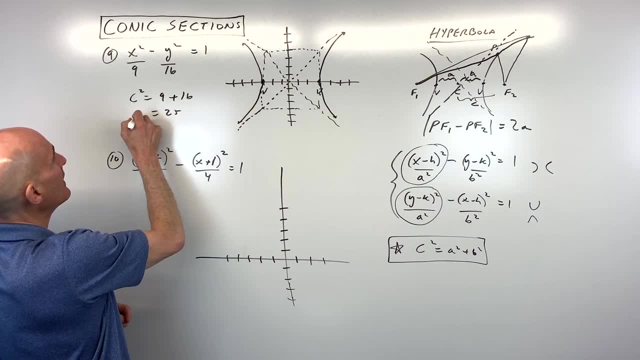 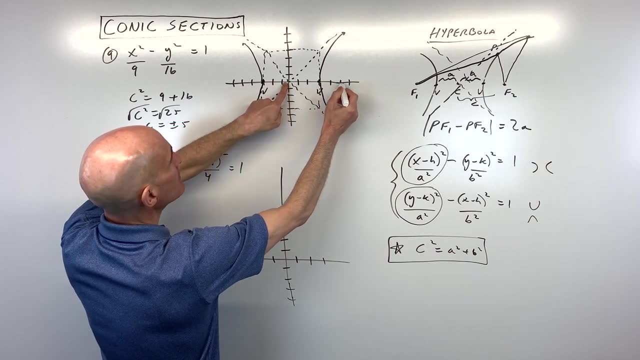 So we have C squared equals nine plus 16.. And if we take the square root, you can see that C is gonna be plus or minus five. So from the center I'm gonna go right five. That's one of the foci. 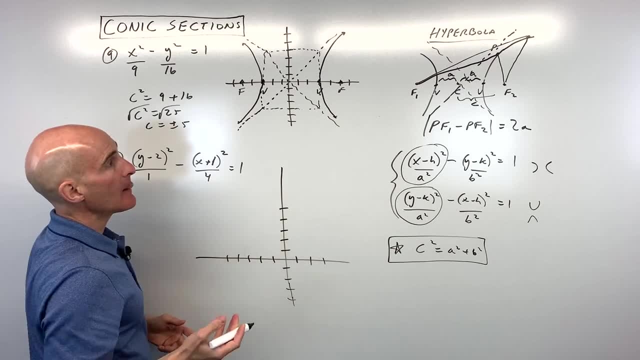 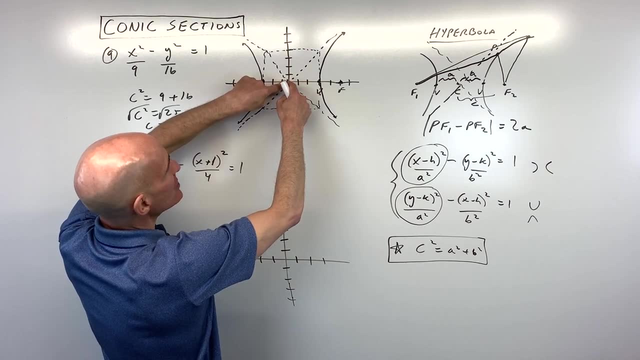 I'm gonna go left. five. That's the other foci, And then the equations of the asymptotes. I'm sorry you can see that this is going through the origin and the rise is four, the run is three, So this one's gonna have a slope of positive 4. 3rds. 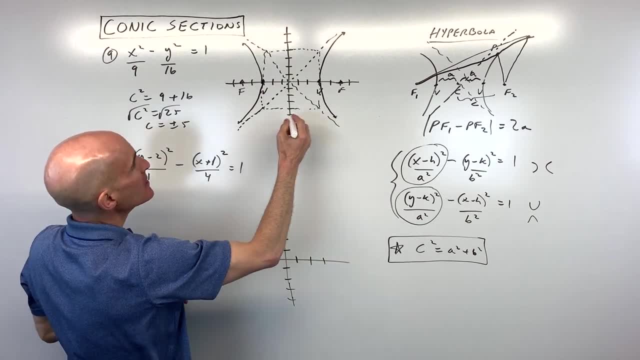 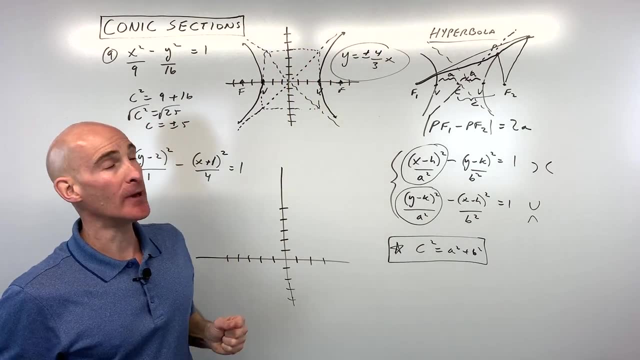 This one, you're going down four over three. This is gonna be negative 4 3rds. So our asymptotes here are gonna be: Y equals plus or minus 4 3rds. Now just a quick note here to kind of help you a little bit. 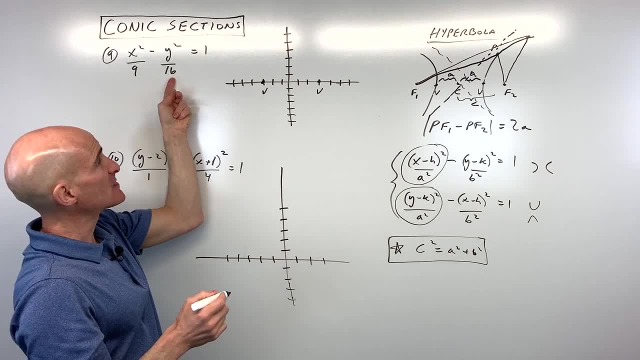 Now this number here, this is our b squared. If I take the square root of 16, that's four. 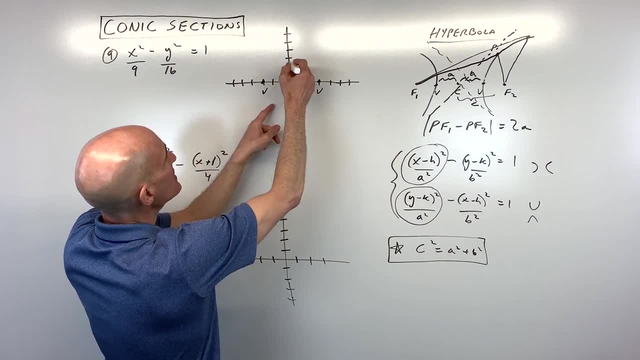 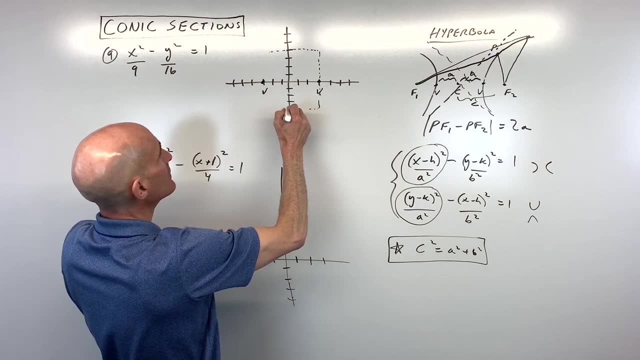 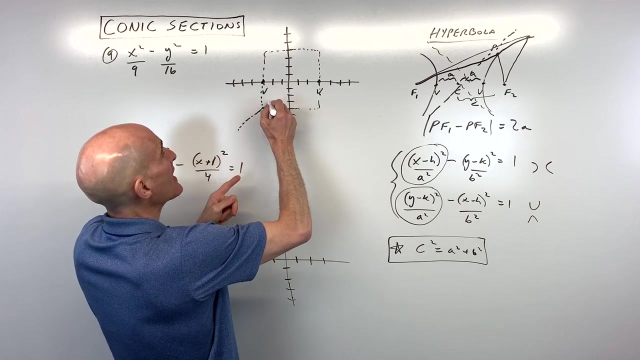 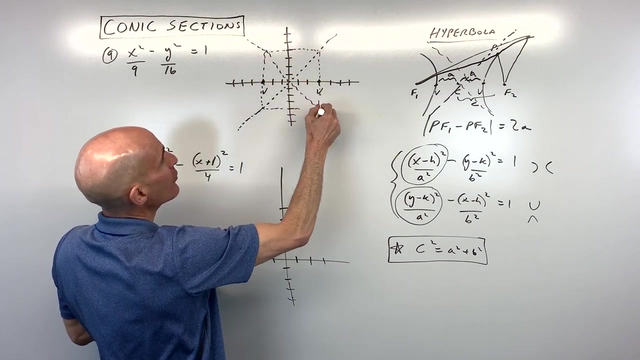 I'm going to go up four and down four. And what I'm going to do is I'm going to draw a rectangle through these four points, okay? I'm going to draw a dashed or dotted rectangle. It's not going to be part of your graph. You're just going to use it as a guide. Then what you do is you draw these dashed or dotted lines, okay? These are our asymptotes, through the corners of the rectangle. Also goes through the center point. Those are our asymptotes. 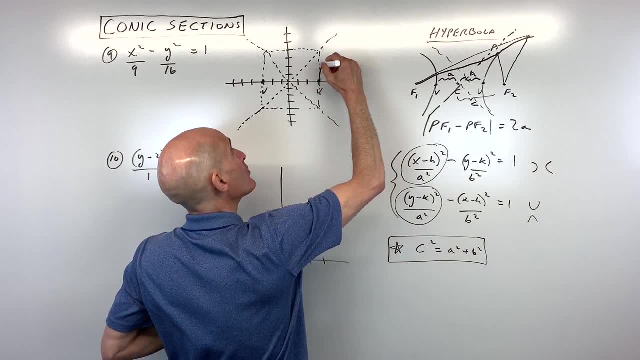 And we're going to use those asymptotes as a guide to graph our hyperbola. The hyperbola is going to get closer and closer to those lines, but not touch, not cross. 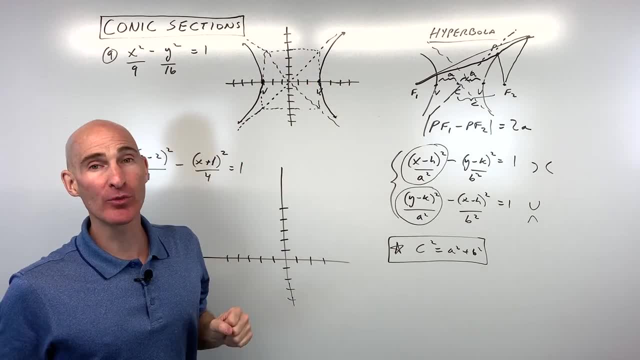 So again, it gives us an idea of how wide the hyperbola is or how narrow, depending. 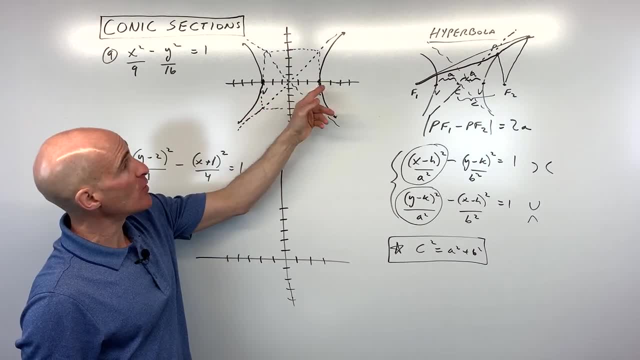 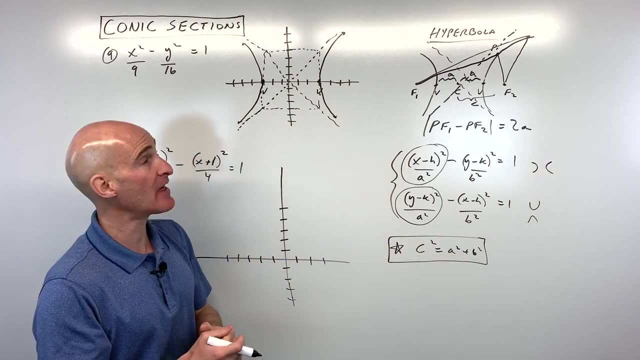 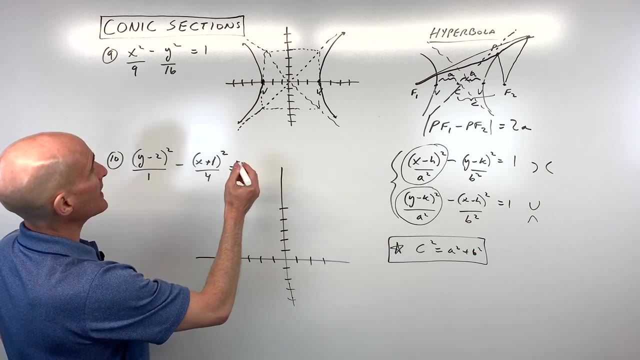 The only other thing that we need to figure out are, well, the equations of the asymptotes, as well as the locations of these focal points, these foci. And we use this formula here, c squared equals a squared plus b squared, just like Pythagorean theorem. Remember when we were working with ellipses, it was c squared equals a squared minus b squared. So very similar, but here we're adding. So in this case, this is our a squared, this is our b squared. 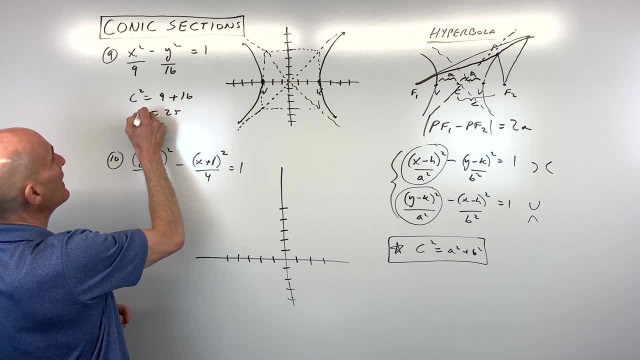 So we have c squared equals nine plus 16. And if we take the square root, you can see that c is going to be plus or minus five. 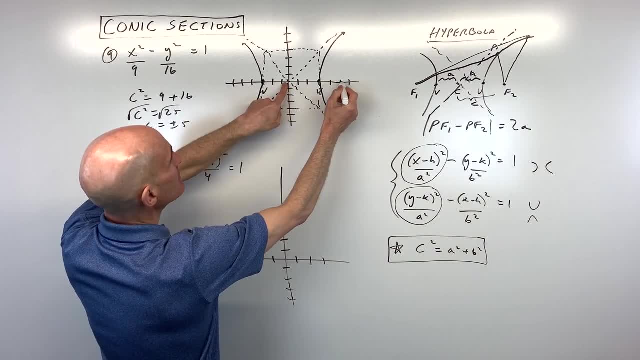 So from the center, I'm going to go right five, that's one of the foci. I'm going to go left five, that's the other foci. 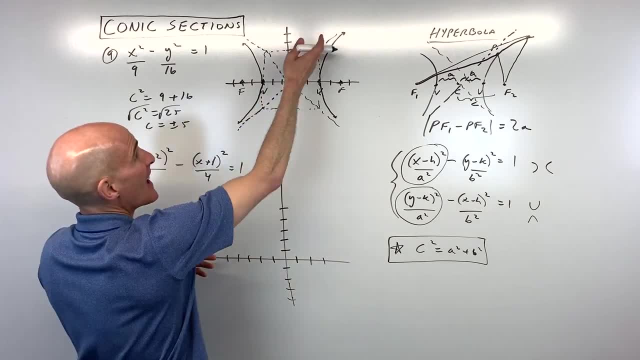 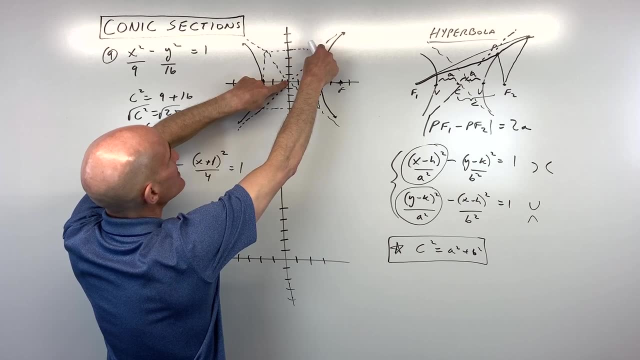 And then the equations of the asymptotes, you can see that this is going through the origin. And the rise is four, the run is three. So this one's going to have a slope of positive four thirds. This one, you're going down four over three. 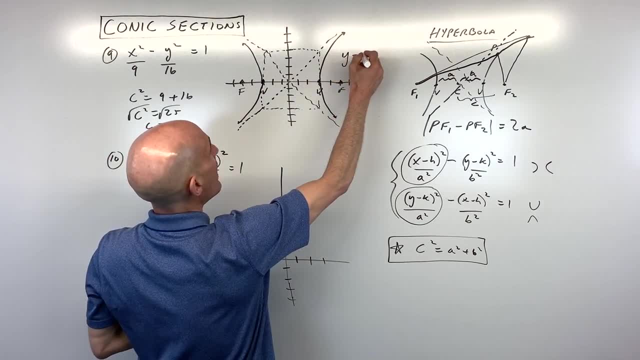 This is going to be negative four thirds. So our asymptotes here are going to be y equals plus or minus four thirds. 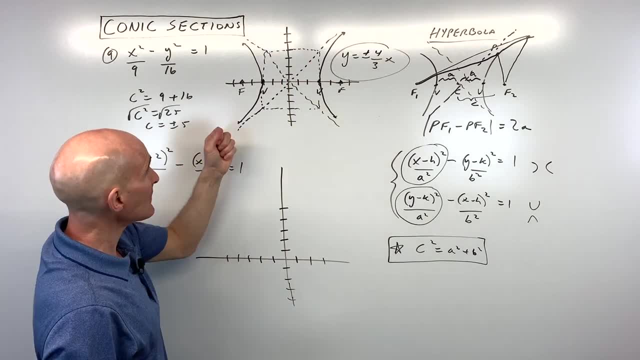 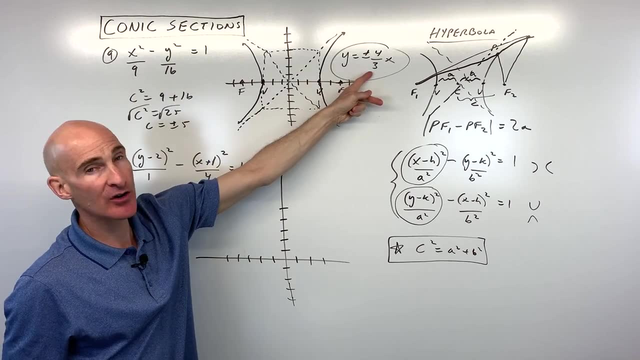 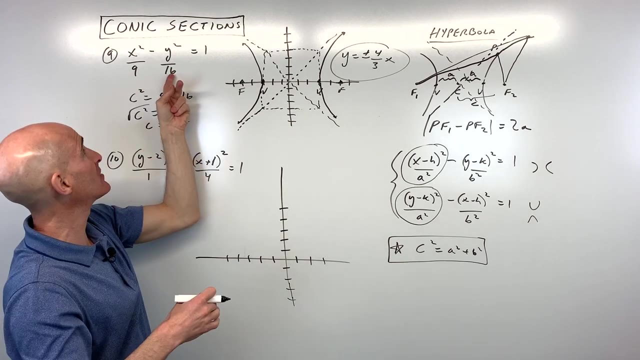 Now, just a quick note here. To kind of help you a little bit. You see how this was square root of 16 is four. And see how the square root of nine is three. You know how the slope is like the rise over the run. Like the change in y over the change in x. The number underneath the y is going to be like your rise. 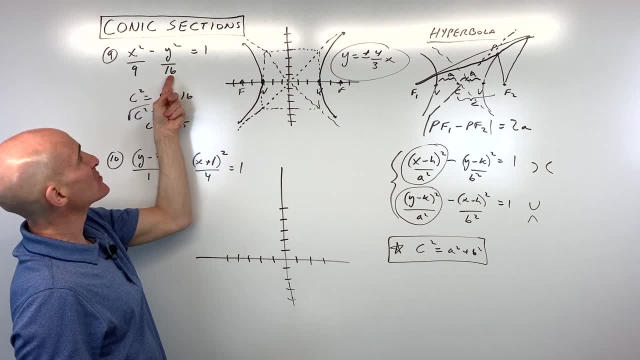 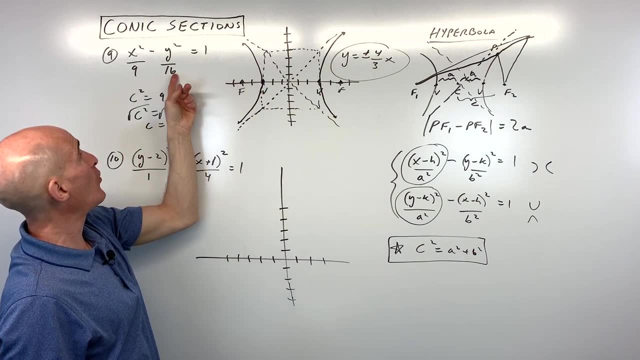 You see how this was: square root of 16 is four. and see how the square root of nine is three. You know how the slope is like the rise over the run, like the change in Y over the change in X. The number underneath the Y is gonna be like your rise. 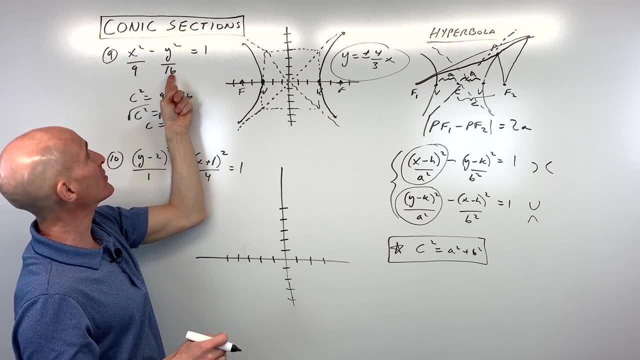 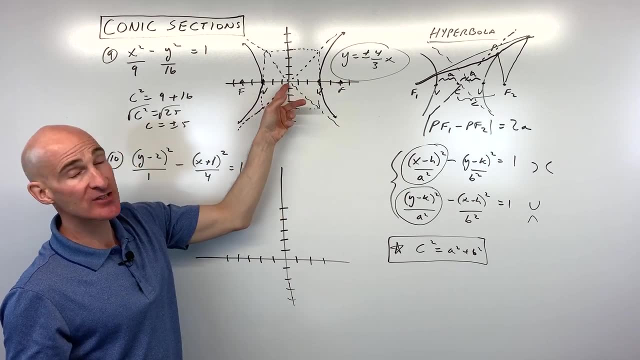 The number underneath the X is gonna be like your run, So you can kind of use that as a guide here. Square root of 16 over square root of nine gives you your slope positive or negative. Now in the next problem, the center is not at the origin. 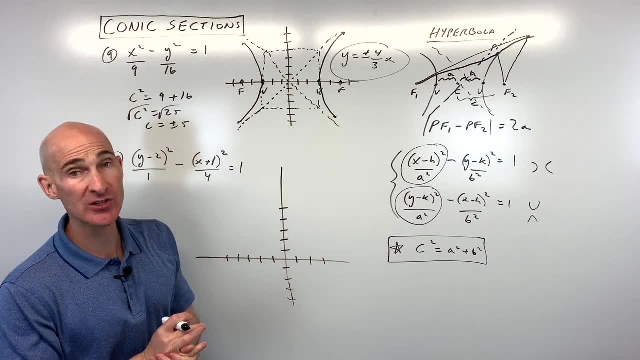 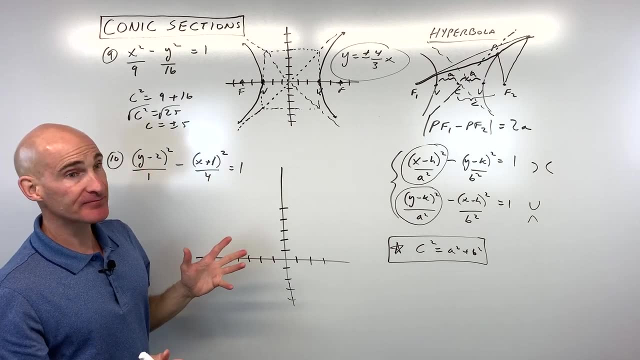 So it's gonna be a little bit more challenging to find the asymptotes, And I'll show you how to do that using point slope form. But let's go on to number 10.. So for number 10 now, where is the center of this hyperbola? 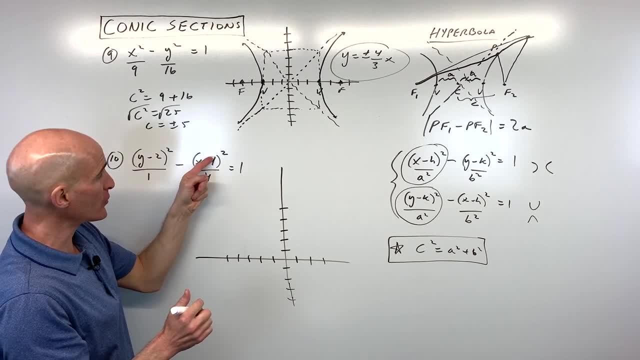 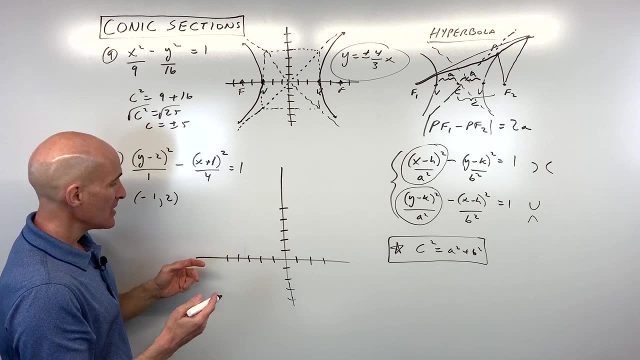 Well, we can see it's gonna be at negative one, positive two. Remember, the one group of the X is the X coordinate, One group of the Y is the Y coordinate. It's, the sign is gonna be the opposite, right? So we're gonna go left one up two. that's our center. 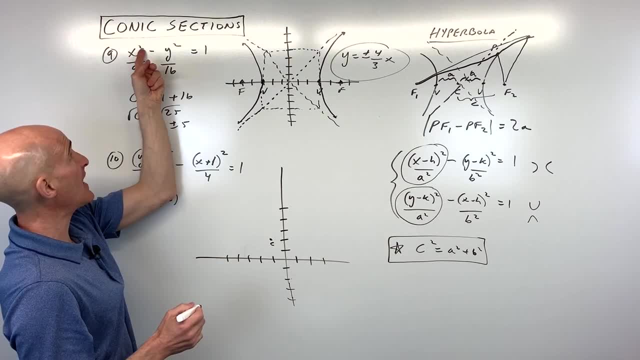 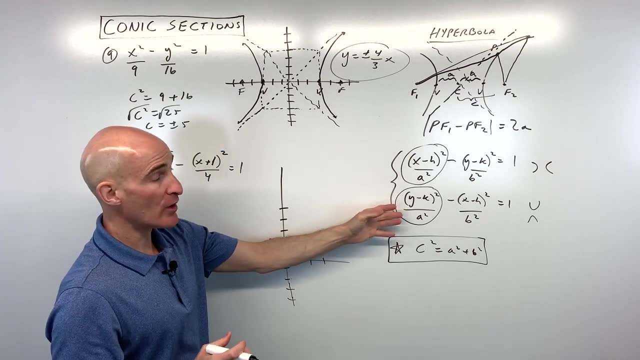 I'll just put C for center. Notice that it's Y squared, whereas this one was X squared. Whichever term comes first, or whichever term is positive, that's gonna give you an idea about whether the graph's gonna open up and down. 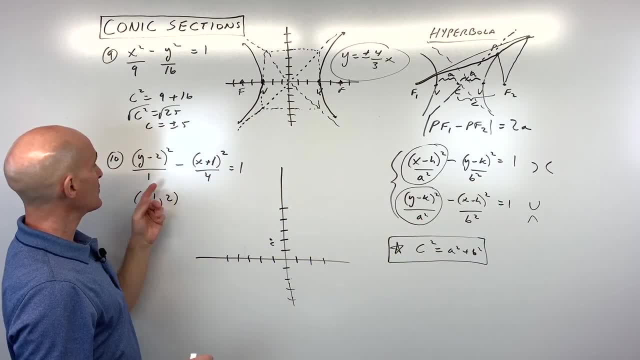 like this one here, or left and right, like that one there. So because it's Y squared, it's gonna be opening in the Y direction, okay, up and down, And this is gonna be our A squared value. So we can see that A squared equals one. 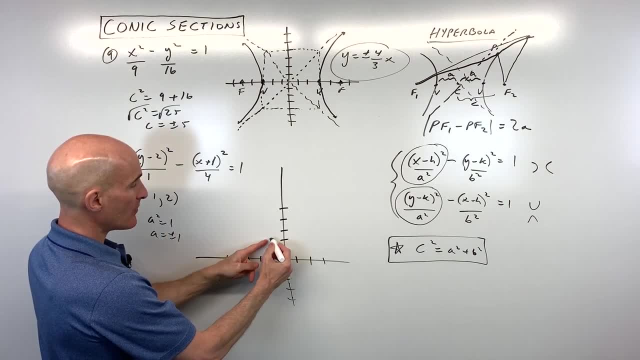 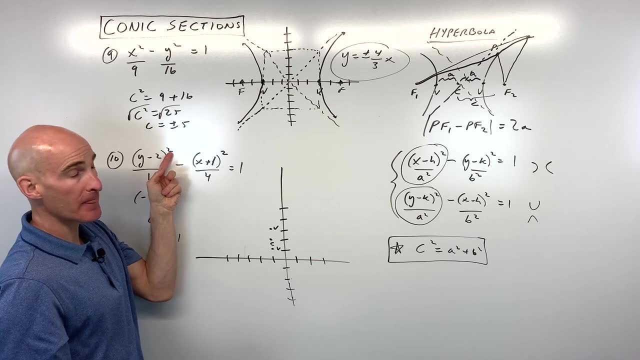 So if we take the square root, A equals plus or minus one. So from the center I'm gonna go up one, That's our vertex, down one that's our other vertex, Again opening up and down because it's Y squared. 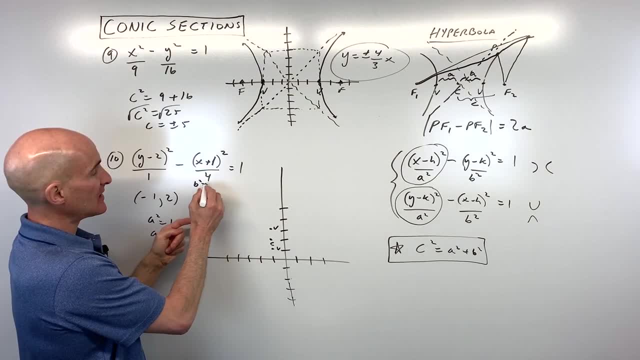 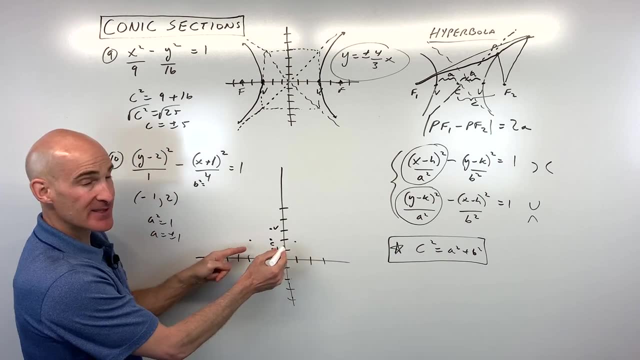 This one, this is our B squared. this one is four. If I take the square root of four, I get two. So what I'm gonna do is, from the center, I'm gonna go right two and left two. Now you see how I put points there. The number underneath the x is going to be like your run. So you can kind of use that as a guide here. 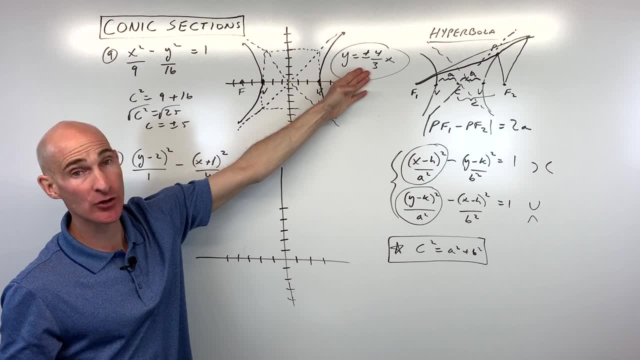 Square root of 16 over square root of nine gives you your slope, positive or negative. Now in the next problem, the center is not at the origin. So it's going to be a little bit more challenging to find the asymptotes. 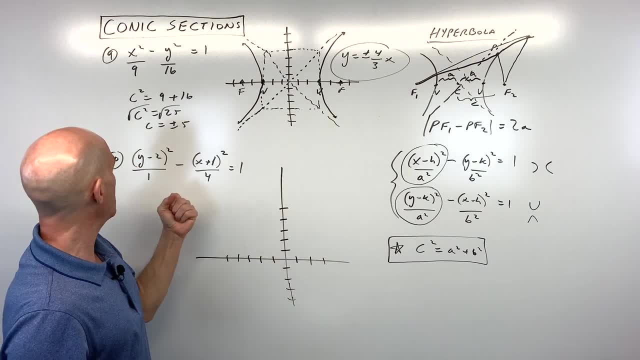 And I'll show you how to do that using point slope form. But let's go on to number 10. 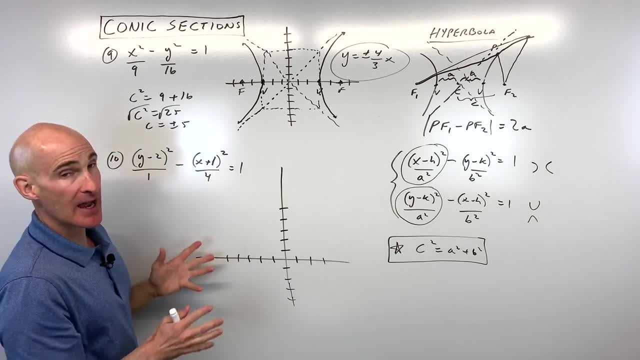 So for number 10 now, where is the center of this hyperbola? Well, we can see it's going to be at negative one, positive two. 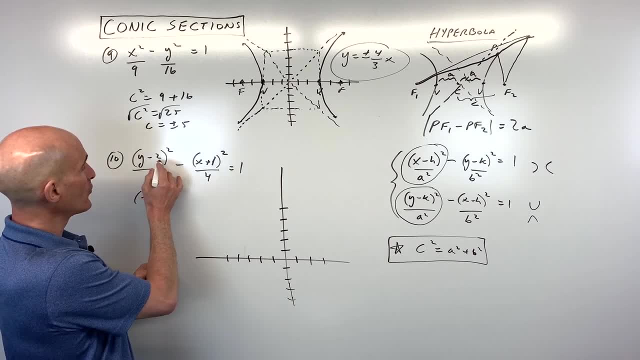 Remember the one group of the x is the x coordinate. One group of the y is the y coordinate. 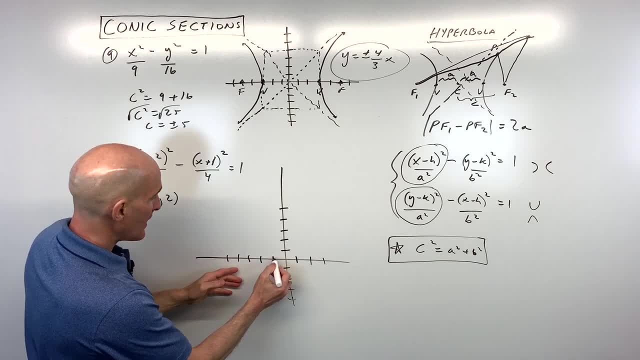 It's the sign is going to be the opposite, right? So we're going to go left one, up two. That's our center. I'll just put c for center. 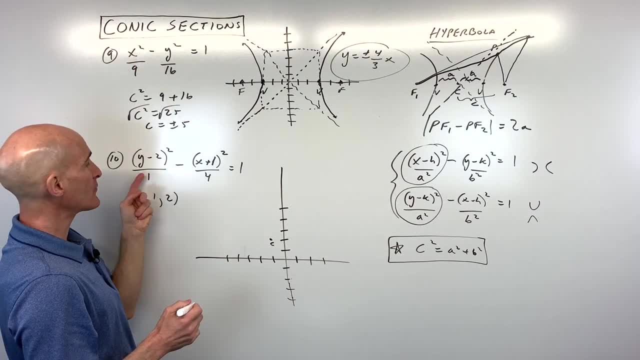 Notice that it's y squared. Whereas this one was x squared. Whichever term comes first. 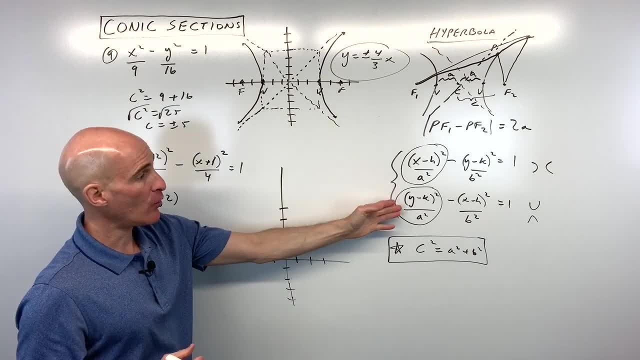 Or whichever term is positive. That's going to give you an idea about whether the graph is going to open up and down. Like this one here. Or left and right. Like that one there. 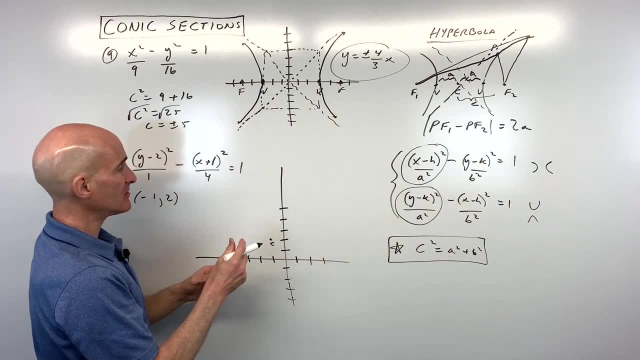 So because it's y squared, it's going to be opening in the y direction. Okay, up and down. 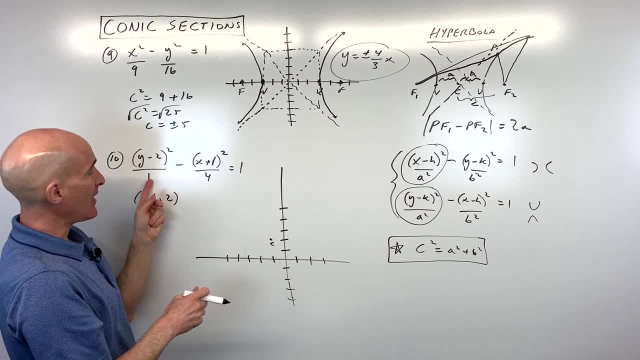 And this is going to be our a squared value. So we can see that a squared equals one. 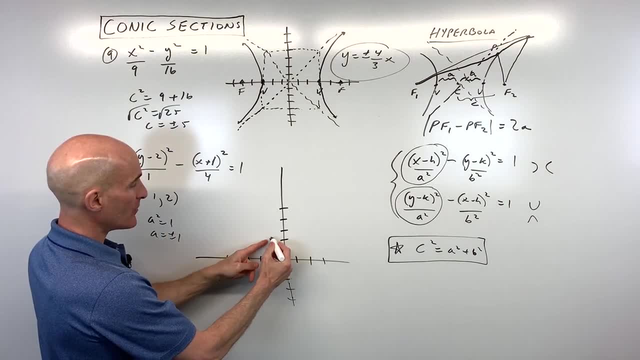 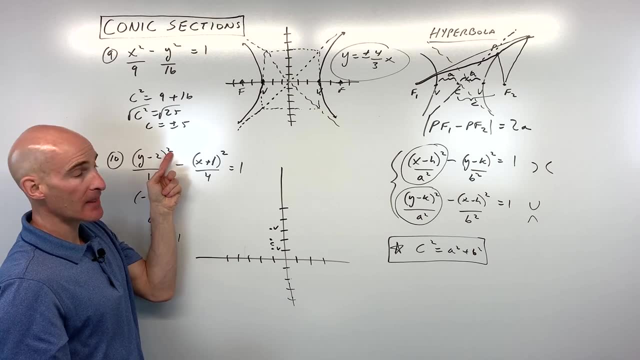 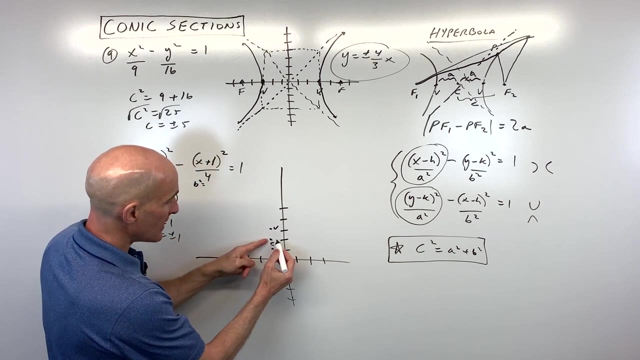 So if we take the square root, a equals plus or minus one. So from the center, I'm going to go up one. That's our vertex. Down one. That's our other vertex. Again, opening up and down because it's y squared. This one, this is our b squared is four. If I take the square root of four, I get two. So what I'm going to do is from the center, I'm going to go right two and left two. 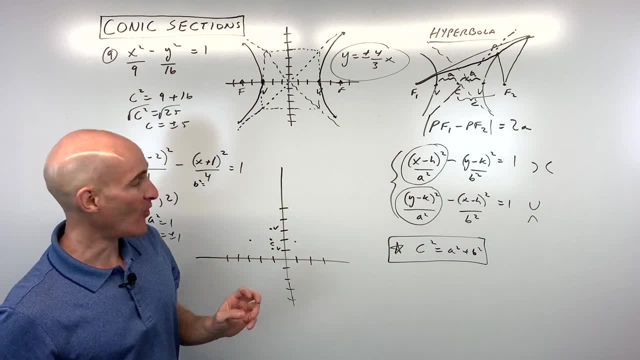 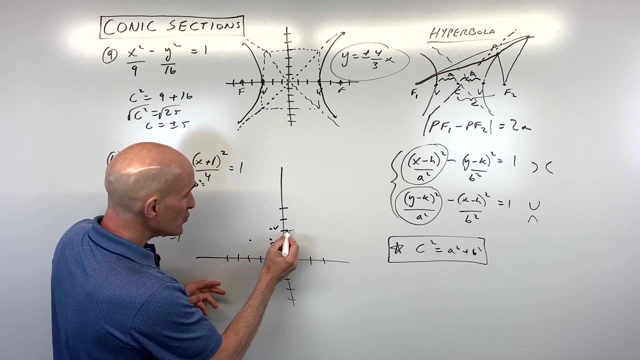 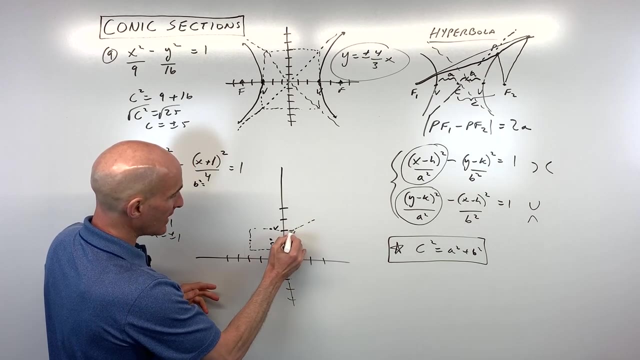 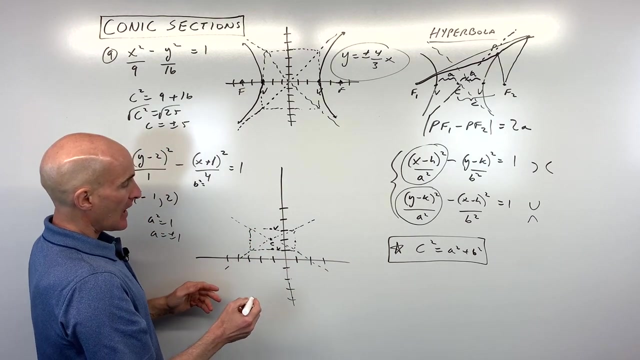 Now, you see how I put points there? Some teachers kind of frown on that. They don't want you to put those points there. Because they don't want you to get confused and start graphing the hyperbola in the wrong direction. But what we're doing is we're just using these points to help us to, you know, draw our rectangle here. And we use the corners of the rectangle and the center point. To draw our asymptotes. Okay, these dotted lines here. So you might not want to draw those points just so you don't get confused. 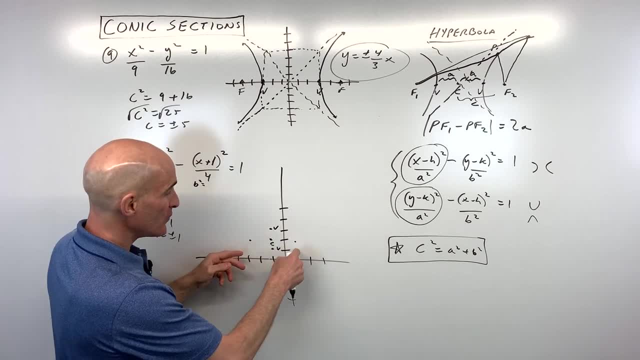 Some teachers kind of frown on that. They don't want you to put those points there because they don't want you to get confused and start graphing the hyperbola in the wrong direction. But what we're doing is we're just using these points. 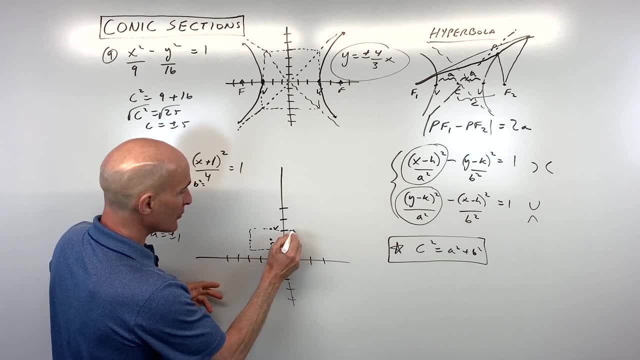 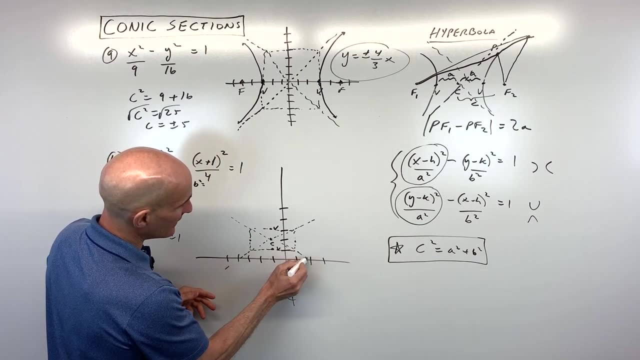 to help us to draw our rectangle here, And we use the corners of the rectangle and the center point to draw our asymptotes. okay, These dotted lines here, So you might not wanna draw those points, just so you don't get confused. These are our vertices here. 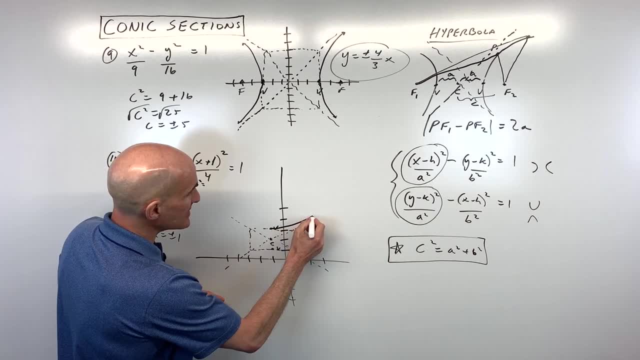 These are our vertices here. These are the points that we're interested in using as the graph goes through the vertices and it approaches those asymptotes. Doesn't cross, doesn't touch. Okay, so that gives you an idea how wide the graph is or how narrow. 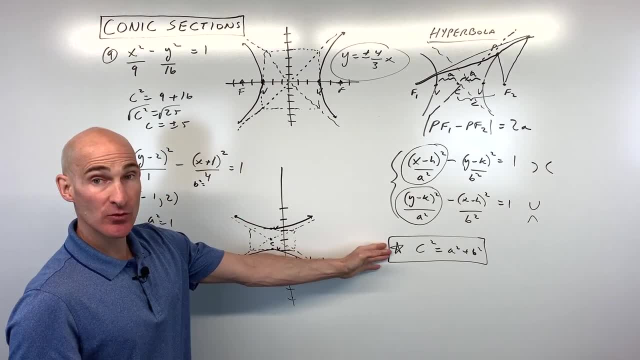 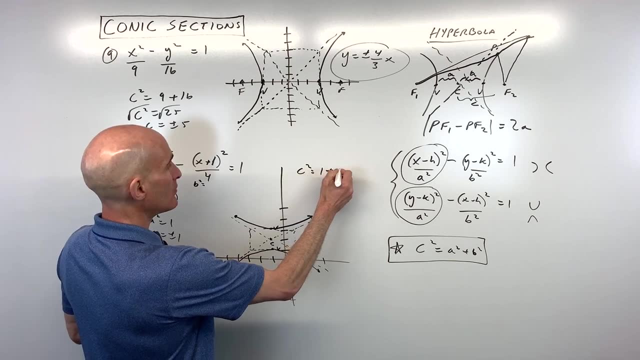 Let's go ahead and find the foci using this formula. C squared equals a squared plus b squared. So this is our a squared. This is our b squared. And so that comes out to c squared equals one plus four. 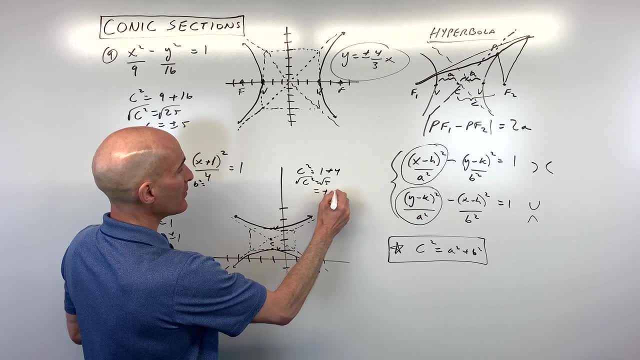 So c squared equals five. And if we take the square root we get plus or minus square root of five. Which is about 2.2 or so. 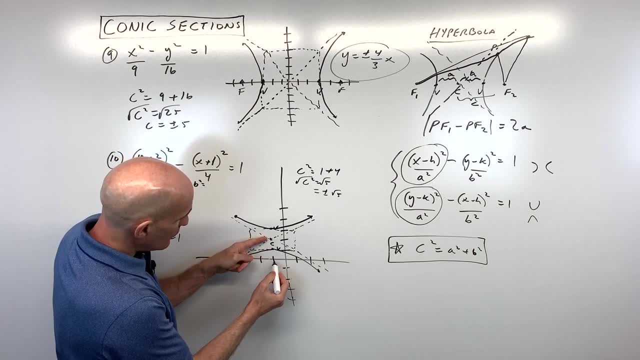 So from the center I'm going to go down 2.2 which is right about here. And I'm going to go up 2.2 which is going to be right about here. 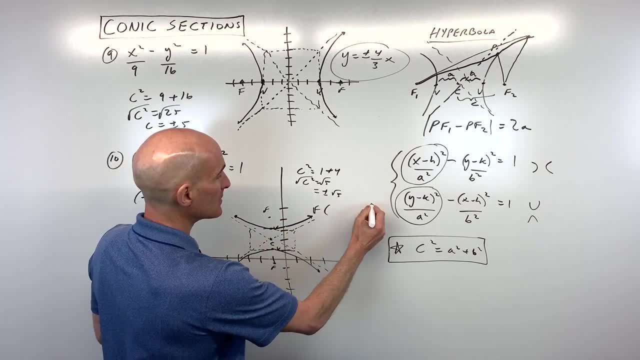 But if you want to be more precise because your teacher is probably going to want to know the exact coordinates of the foci. You can take that center point. Which is at negative one two. 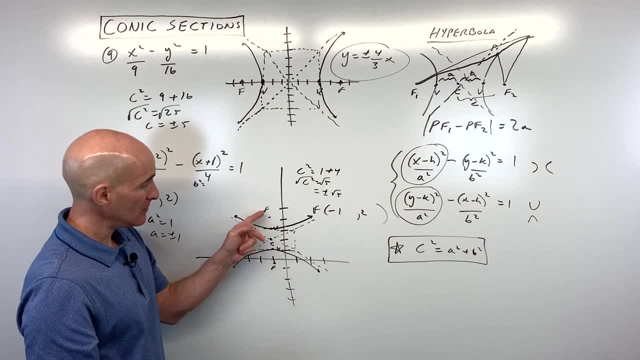 But because I'm going up and down that's affecting the y value. 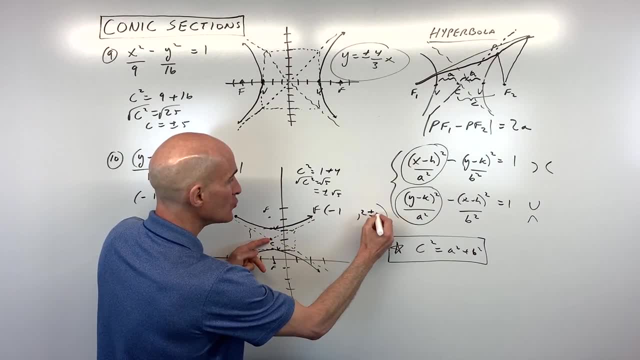 And we're going up square root of five, down square root of five. So that's going to be two plus or minus square root of five. 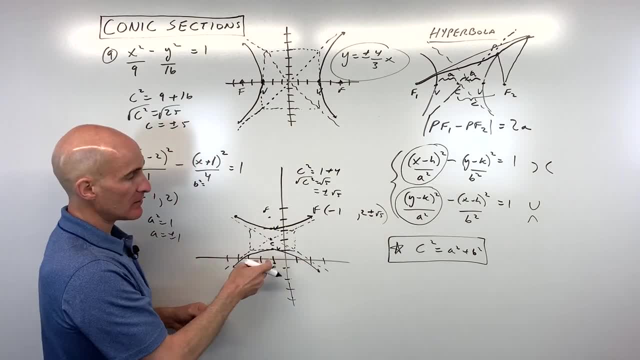 I'm adding that to the y coordinate for that vertical up and down. 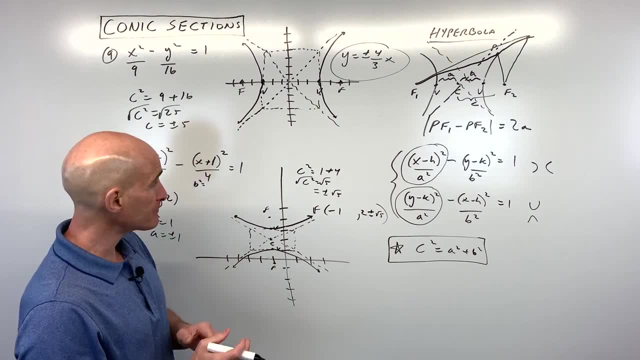 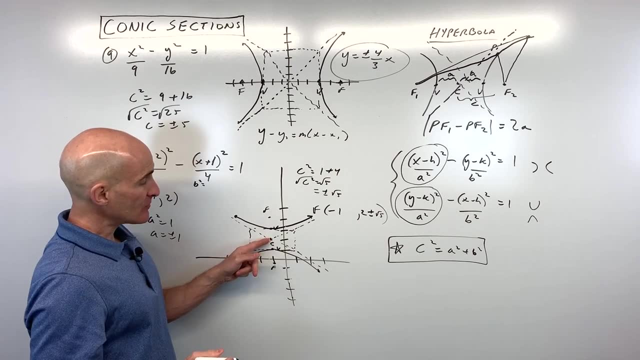 So now the equations of the asymptotes. Probably the toughest part about this problem. Remember the point slope form. Remember y minus y one equals m times x minus x one. The asymptotes they always go through that center point. Which was negative one two. 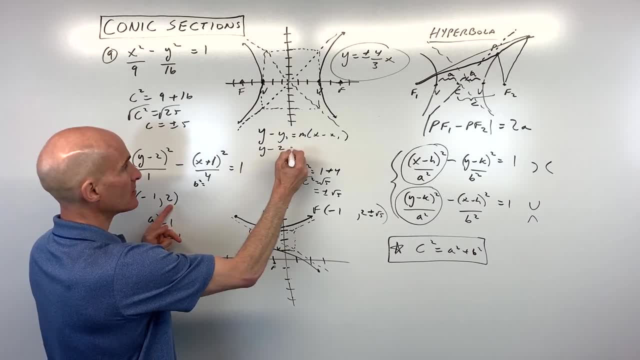 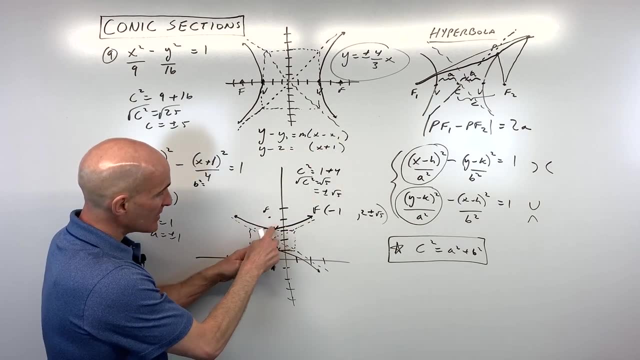 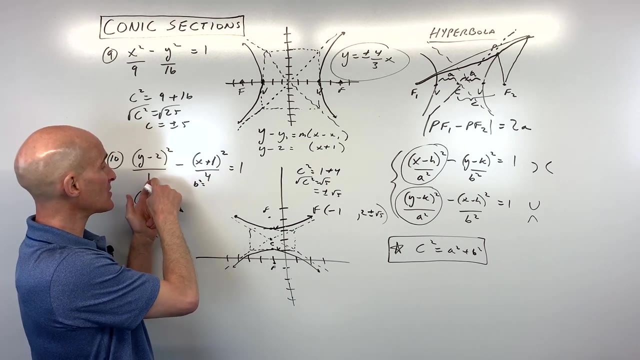 So we can start off by saying y minus the y coordinate of the center equals x minus the x coordinate of the center. Those two negatives cancel. The slope is rise over run. Right? Or you could think of the number of the y is going to be the rise. The number underneath the x is going to be the run. But these are squared. We have to take the square root. So square root of one is one. Square root of four is two. 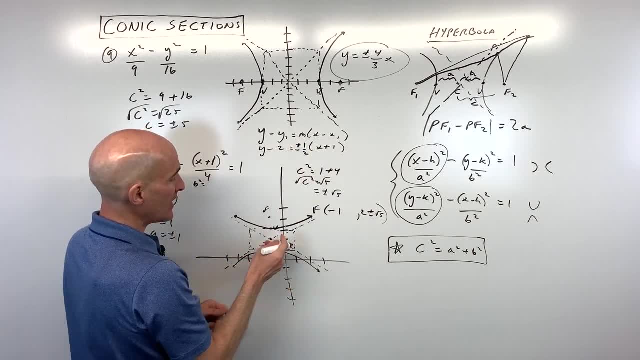 One over two. Plus or minus. Right? So this one has a positive slope. This one has a negative slope. 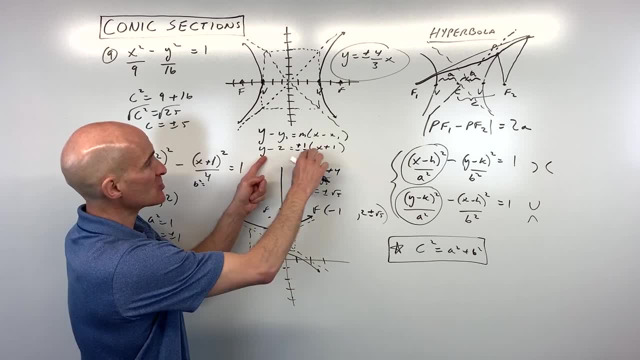 Now if you want to take it further and solve for y. You could write this as two separate equations. 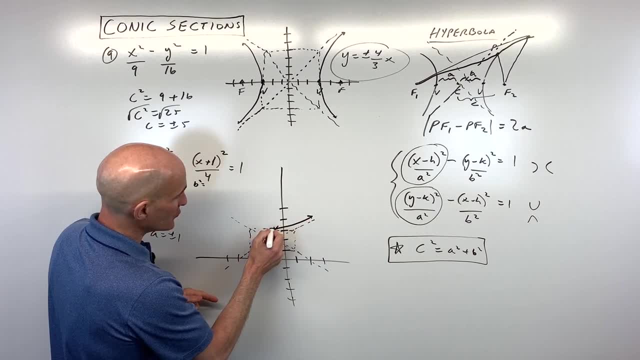 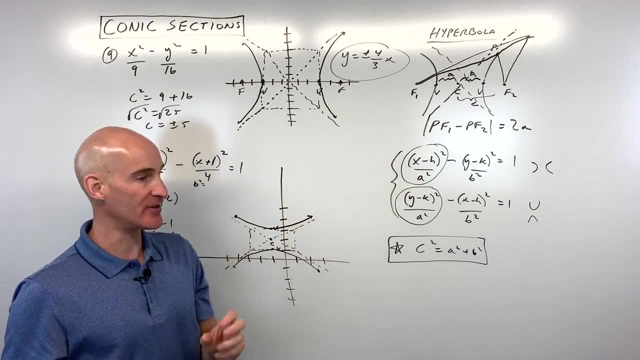 These are the points that we're interested in using, as the graph goes through the vertices and it approaches those asymptotes: doesn't cross, doesn't touch, okay. So that gives you an idea how wide the graph is or how narrow. Let's go ahead and find the foci using this formula. 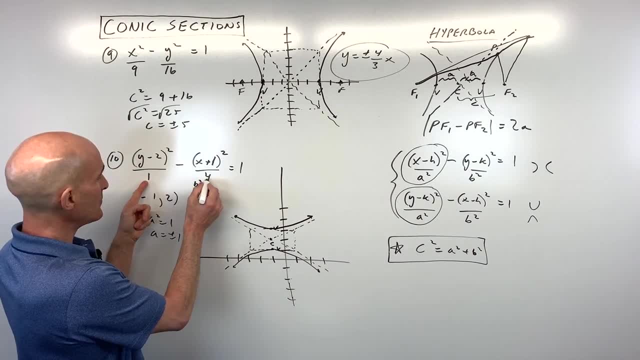 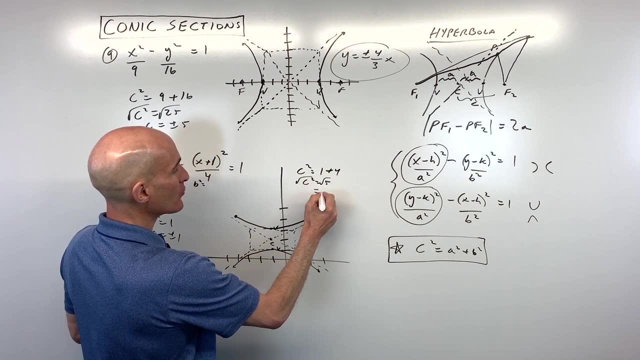 C squared equals A squared plus B squared. So this is our A squared, this is our B squared, And so that comes out to: C squared equals one plus four. So C squared equals five, And if we take the square root, we get plus or minus square root of five. 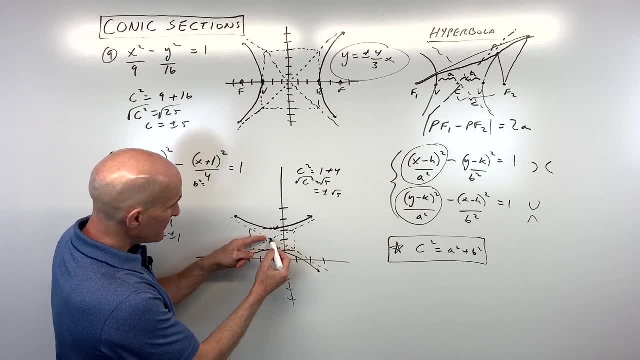 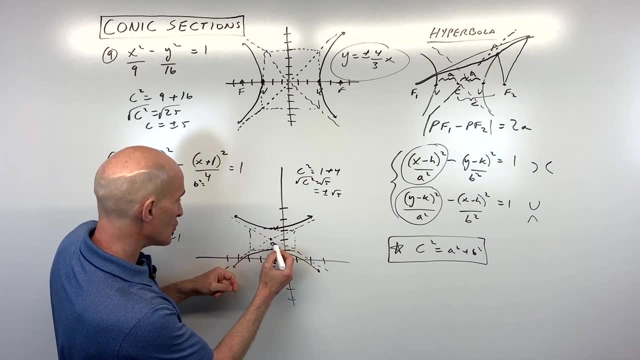 which is about 2.2 or so. So, from the center, I'm gonna go down 2.2,, which is right about here, And I'm gonna go up 2.2,, which is gonna be right about here. But if you wanna be more precise, 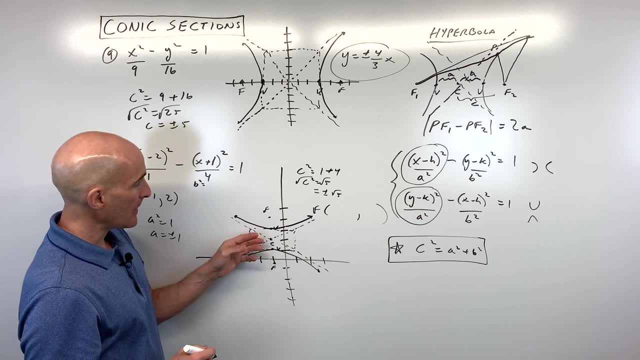 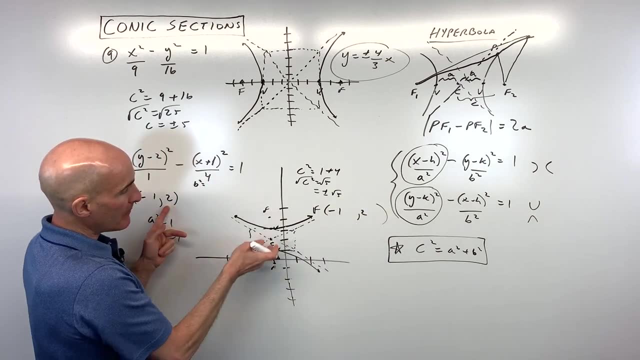 cause your teacher's probably gonna wanna know the exact coordinates of the foci. you can take that center point which is at negative one two. But because I'm going up and down that's affecting the Y value And we're going up. square root of five. 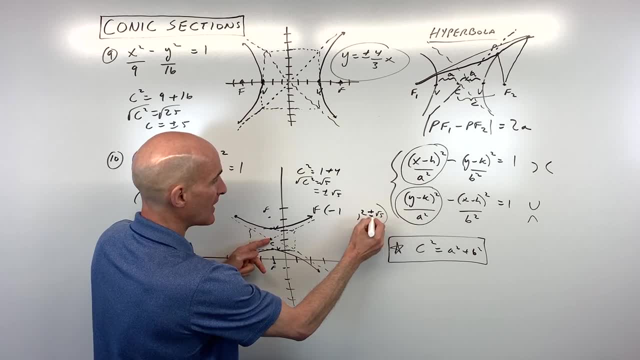 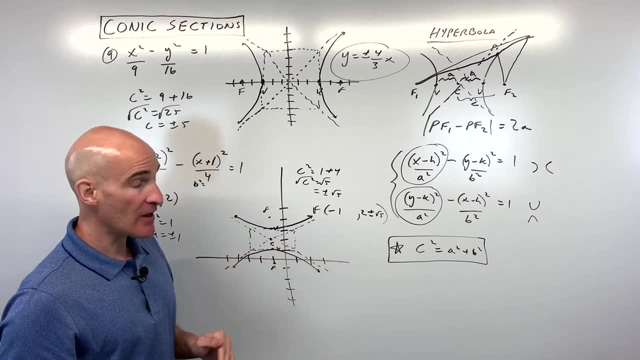 down square root of five. So that's gonna be two plus or minus square root of five. I'm adding that to the Y coordinate for that vertical up and down. So now the equations of the asymptotes, probably the toughest part about this problem. 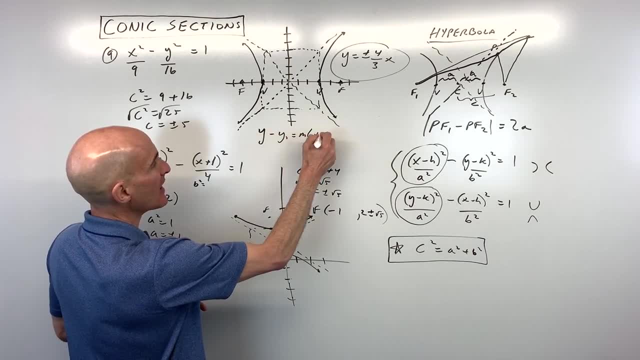 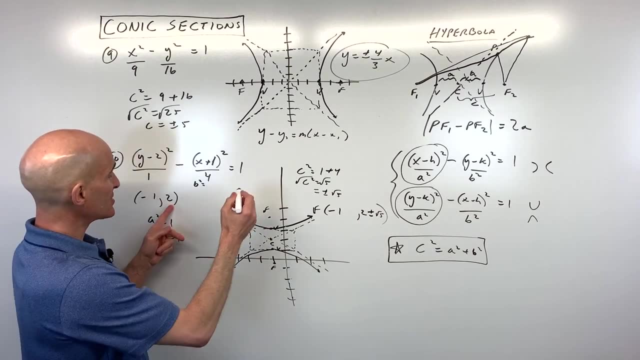 Remember the point slope form. remember Y minus Y one equals M times X minus X one, The asymptotes they always go through that center point which was negative one, two. So we can start off by saying Y minus the Y coordinate of the center. 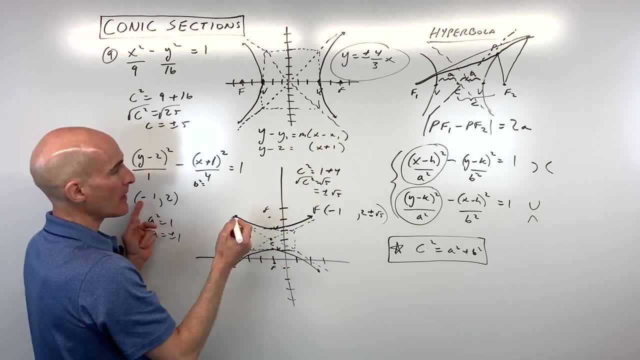 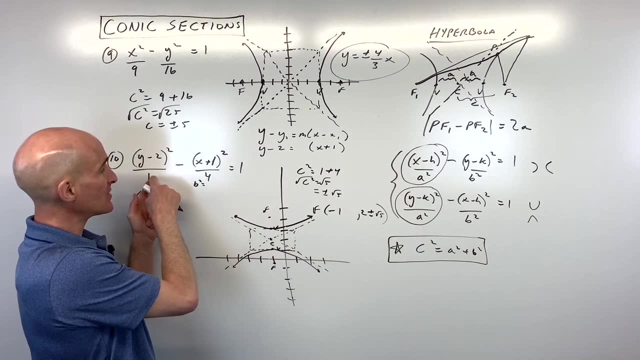 equals X minus the X coordinate of the center. Those two negatives cancel The slope. is rise over, run right. Or you could think of: the number of the Y is gonna be the rise, the number underneath the X is gonna be the run. 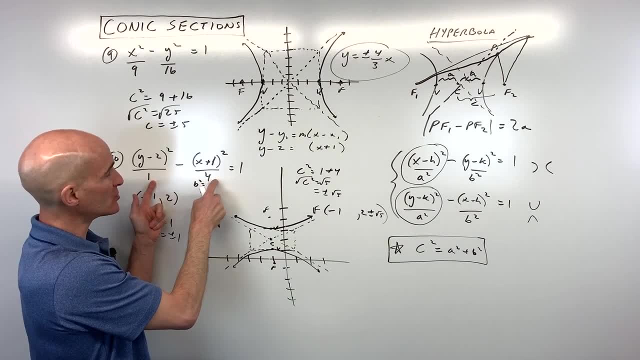 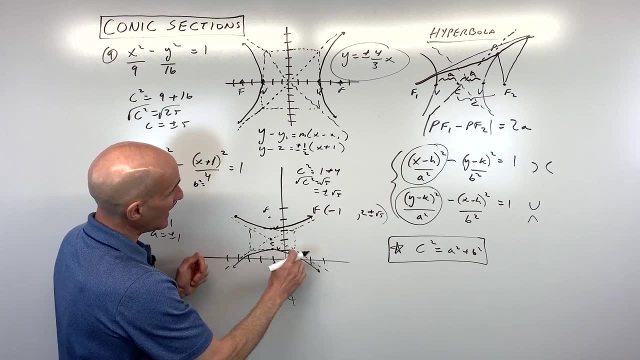 but these are squared, We have to take the square root. So square root of one is one, square root of four is two, one over two plus or minus, right? So this one has a positive slope, This one has a negative slope. 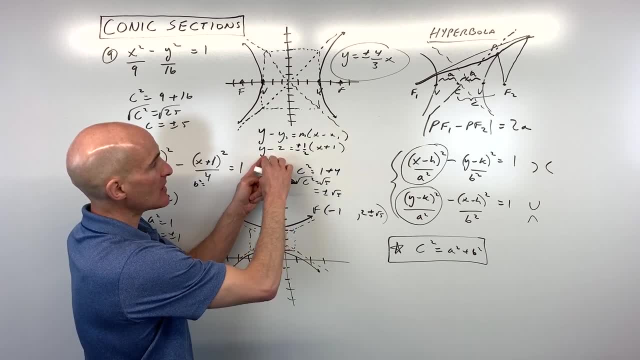 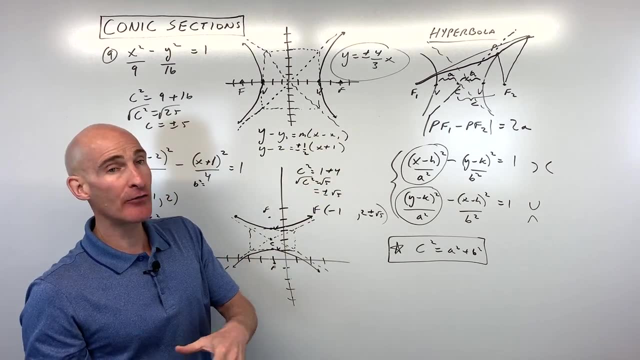 Now, if you wanna take it further and solve for Y, you could write this as two separate equations, one with the positive one half, one with the negative one half. You could distribute the one half, add the two, get the Y by itself.